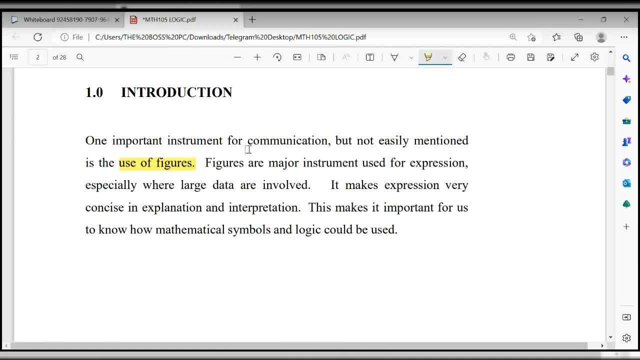 it's not giving the recognition that it serves, and we are studying it so that we can, you know, know that, yes, this is what this should be about. Okay Now, figures are major instruments used for expression, especially when large data is involved, and it makes expressions very concise. It makes 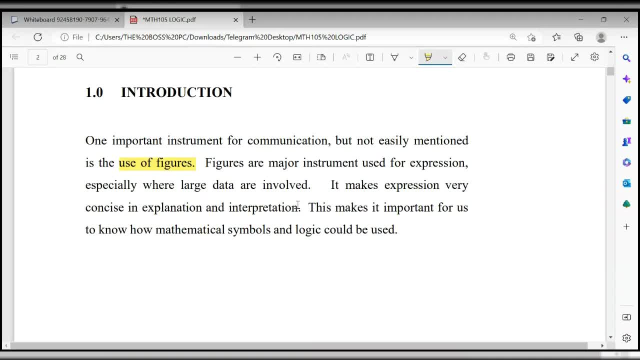 very, very concise in explanation and adaptation So you can be able to explain all right and interpret things easily when you use figures. Now, when we say explanation, please, who can describe? you see, explanation to explain something. That means to tell more, to give more. 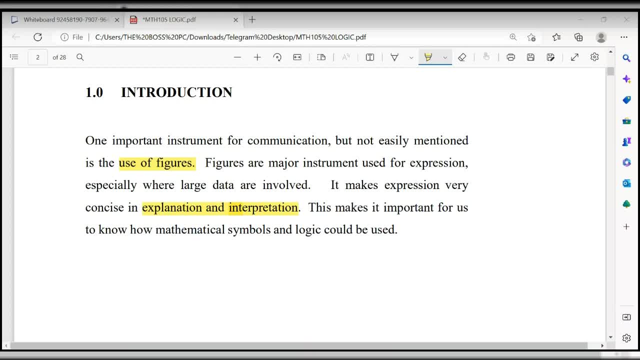 information about a concept. okay, Interpretation is different from explanation. Interpretation means to give something your own meaning. all right, i can come here and tell us, um, i can come here and tell us that, um, that nigeria is a very, very good country. all right, nigeria is a very, very good country that. 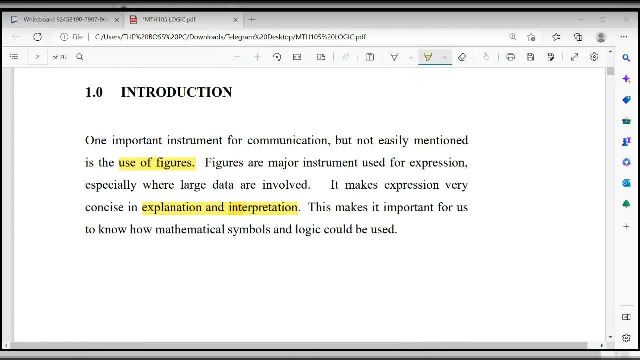 has an information. all right now to you. is nigeria really a good country or not? that is your own interpretation, all right. so if i begin to give you reasons why nigeria is indeed a good country, that becomes explanation. if you're actually understanding what i'm saying, please give me a love emoji. okay, give me a love emoji if you really get it. that's what sucked in. 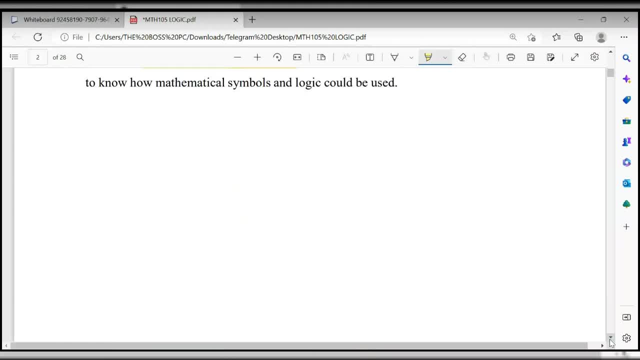 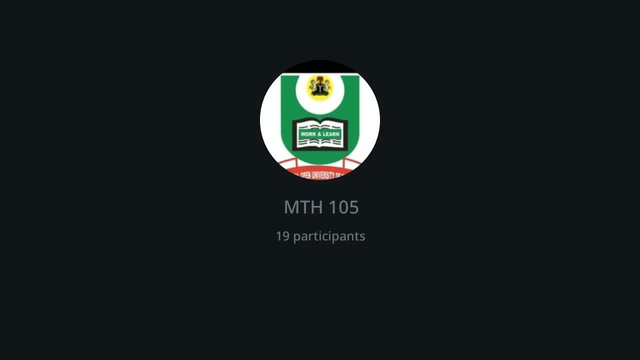 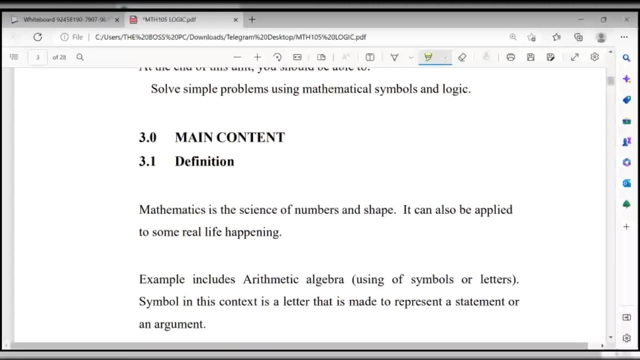 because this topic is a topic that you need to take bit by bit, like beat by beat is the first topic in the course material, but you see, you saw how difficult to understand, so you need to be taking it little by little and explaining them one of them. okay, yes, thank you. thank you so much. 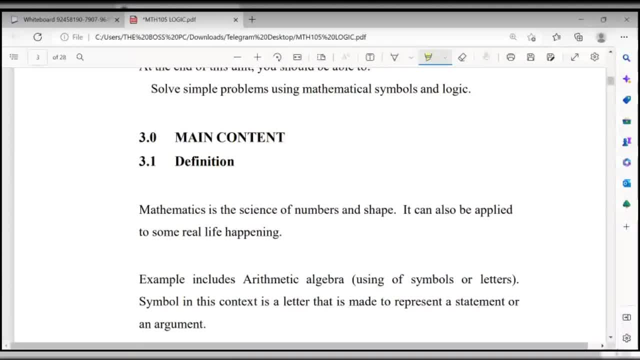 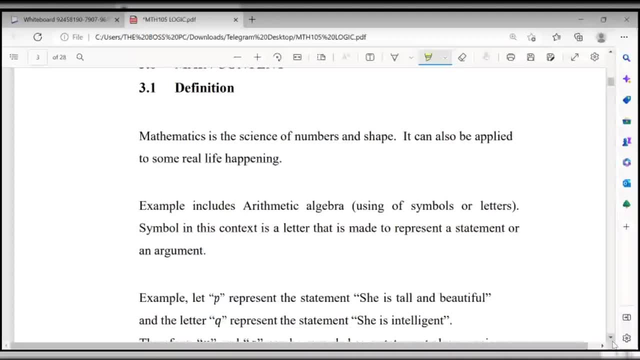 journey. thank you so much, donio. you're all loved by the boss, okay, so let's continue. definition: what are we supposed to define here? we're supposed to define mathematics as opposed to define logic. you are supposed to define symbols, all right, yes, you're supposed to define all these things, and 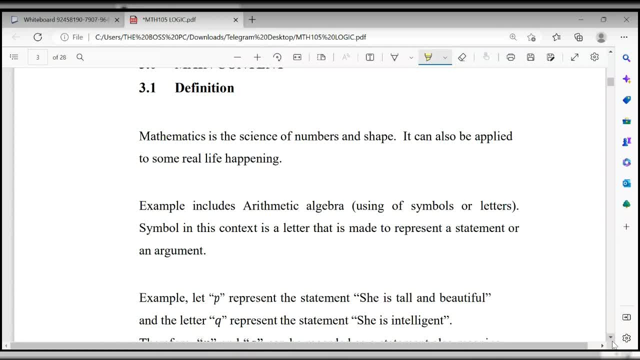 that's not how you want to do it. your cma and examination questions- you always have all this. okay, they will always ask you um this question questions and omits, um, you know omits um certain words in the sentence. it's okay now. mathematics is the science of numbers and shape. it can also be applied in to our real life. 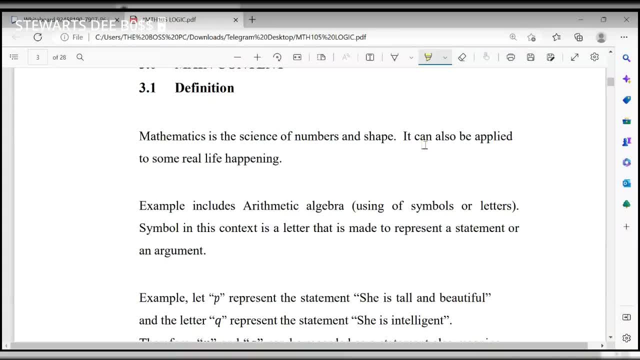 scenario. okay, so you can. it can also be applied into real life situations. so we say: real life situations, realize situation. hmm, realize situation. what are we really I'm talking about here? okay, you know. what I started to say is that mathematics is not always abstract. okay, two plus two is four. that 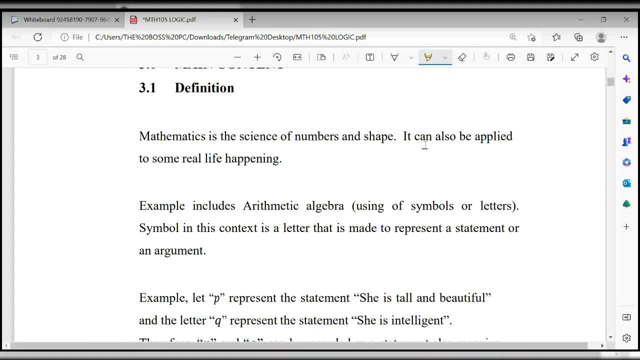 is. you know in the abstract? um, that's looking at it as abstract. we're not tell somebody: okay, two cups of rice and two cups of rice added together, what will it be? so in that case, you're not applying that knowledge to solving problems around you. there we have examples of mathematics. 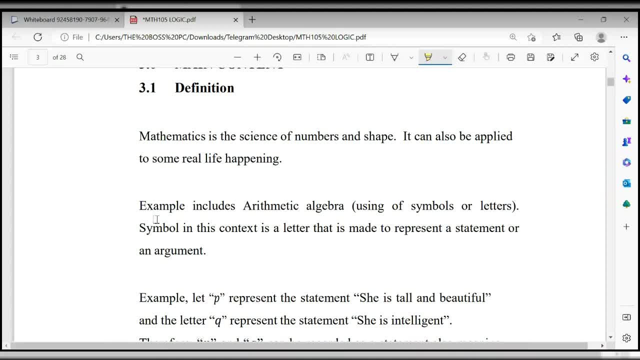 now they always ask this as a question. so notice we have orgy. mathematical algebra that is a topic in sorry arithmetic, orgy by the topic in mathematics, all right, and they not explained that mathematical algebra okay and said it is use of symbols or letters. please, aside from arithmetic. 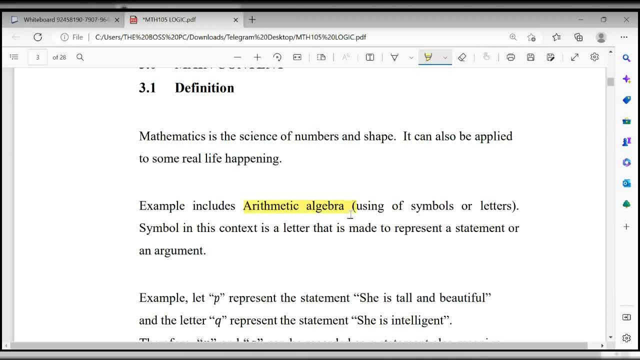 algebra. there are other examples, there are other topics in mathematics. can somebody give me um one or two? can somebody give me one or two? nobody hope. we have linear equation. linear equation- uh-huh, we should have one again. we have logarithm log reading. very good, yeah, thank you so much. you have matrix. okay, a matrix is matricul matrix, no matrix matrix as X. 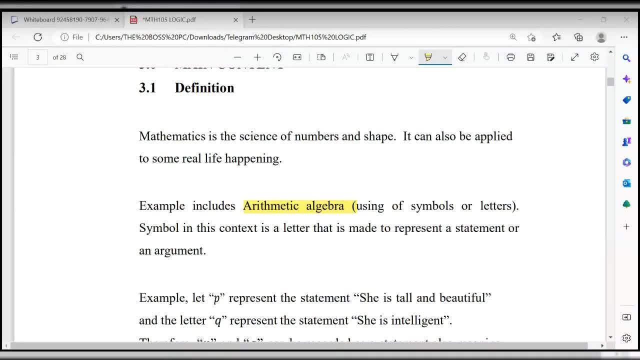 okay, there is set theory, there is trigonometry and so many on as a lot of other topics. okay, now, from this arithmetic algebra, we can see symbols, and that's symbols. that was being explained. they say symbol in this context is a letter that is used to represent a 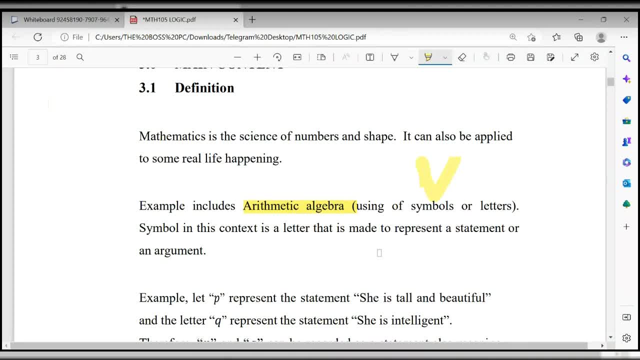 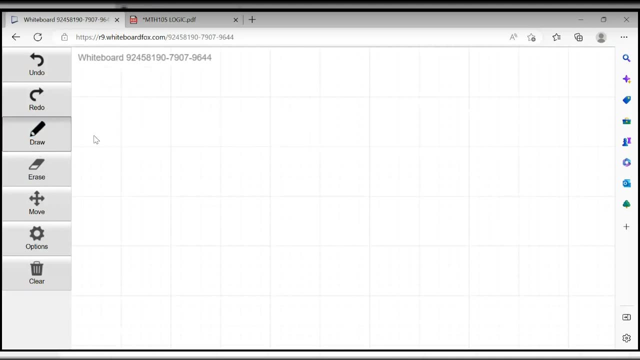 statement or an argument. letters that are used to represent a statement or an argument is what you call symbols. okay, so um. in the last class, I shared my board just this way and I told us: okay, fine, you have something like um 2x X, excuse me. 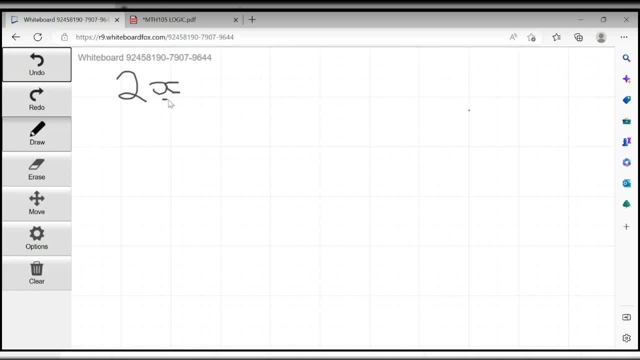 has something like 2x. now this X here, X here- represents a value, because this actually means two times X. all right, so you know, if X should be one, for example, then you have two times it equals to 2if X should be two, then you have 2 times two equals sum. so this is the variable, all. 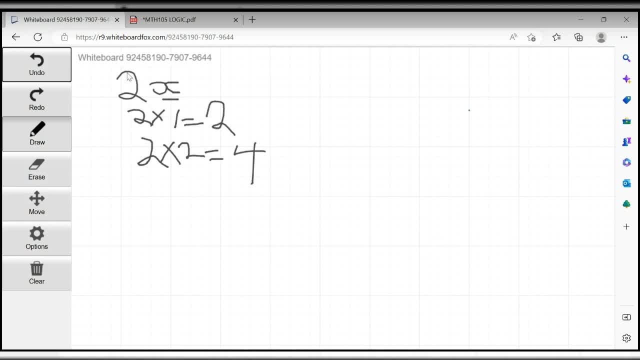 right. the column variable in mathematics and this two here is the constant, so it's variable because he can change. you can take any value, but this one is constant, he stays that way. all right, I think when about um computer or um somewhere in computer. but talking about constant and variable, changing the 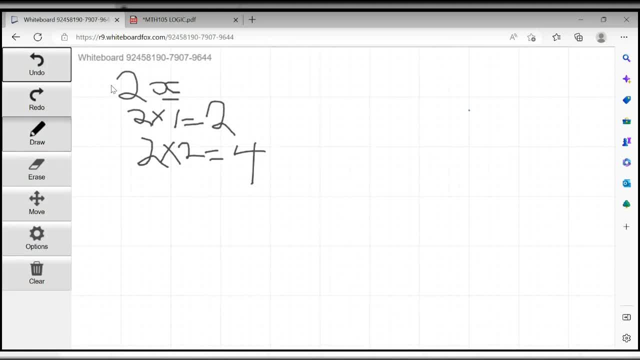 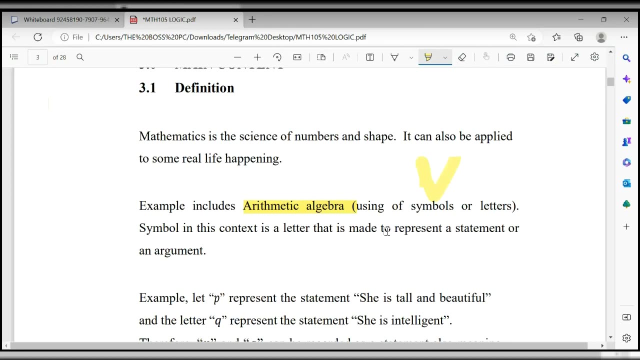 the constant to see the impact, and stuff like that. okay, so this is simple. when you use a letter to represent a word, a preposition, and in logic it might not really be this expressed this way. okay, so these symbols could be used to represent a statement, just as we can see in this example here. 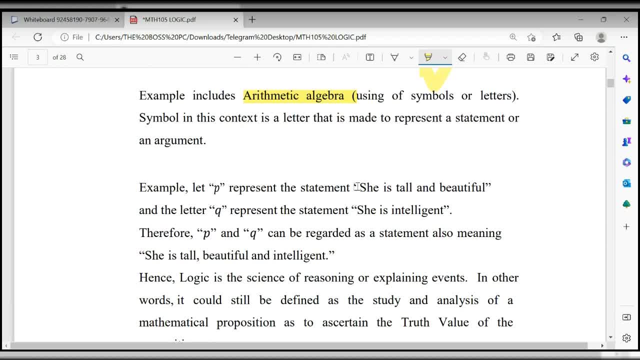 so let's say that: um, we have a statement here: she is tall and she is beautiful. we have a statement here: she is intelligent and we use symbols. the symbols that we use here to represent them are p and q. so anywhere you see she is tall and beautiful, okay, or anywhere you see p in this. 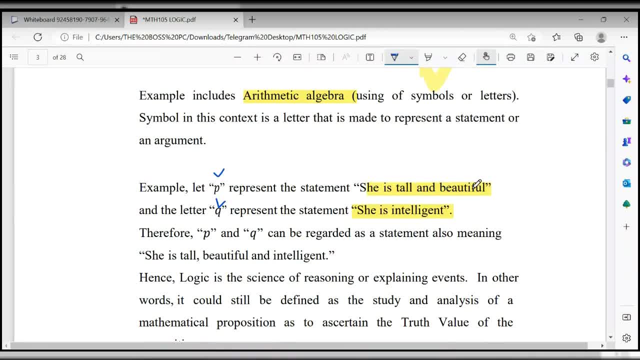 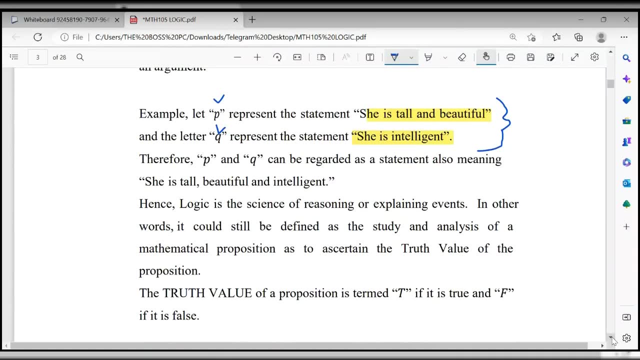 context, it means that they're saying she's not beautiful anyway, you see q. so these are symbols representing d these statements. okay, so logical statements will be represented by symbols, right? you know, sometimes we apply this, maybe when you are writing or when you are. you know, mostly your write-up. 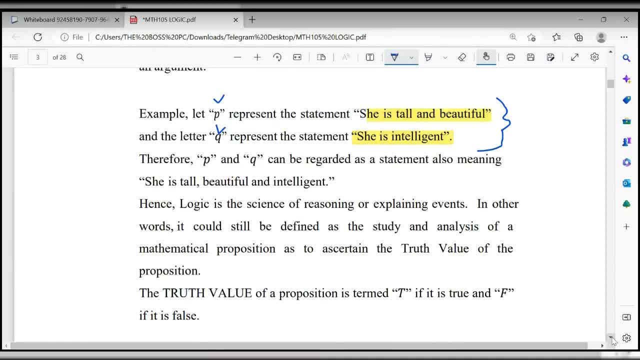 you don't want to, or you don't have time to be writing so long, and just use these symbols to represent what you want to represent. um, do we really get that? is that pretty clear? yes, i see some people are just joining. you're welcome, um, so we move on now. 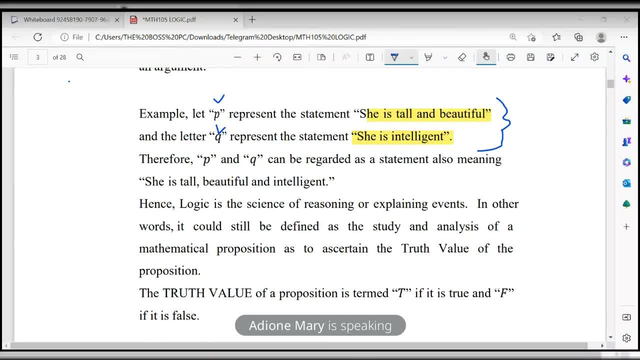 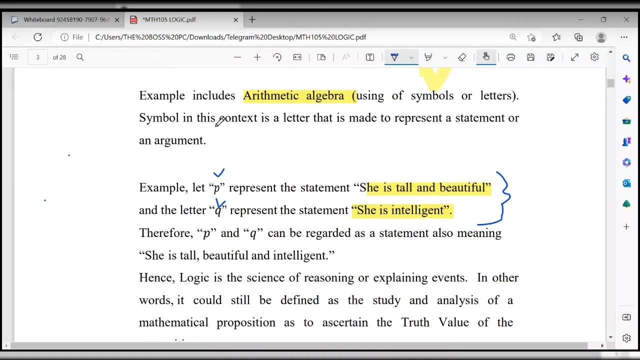 um, uh, who is that? where should i? where should i come again? please, i missed isyama. where were you lost? excuse me, mrs. the use of symbols. okay, man. so when we talk about us, symbols means in this context, because we have other contexts in which we use symbols. let me. 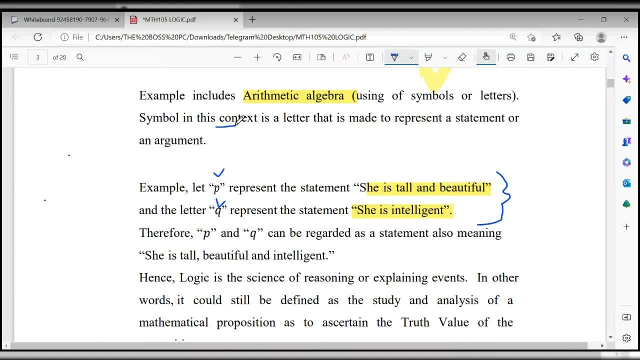 um, give us some other examples so that you can understand this one better. okay, so we have a situation like this. so, um, we have situations whereby, um, you are moving on the road, okay, and then you see a sign, danger, okay, see, you know an image, you know. 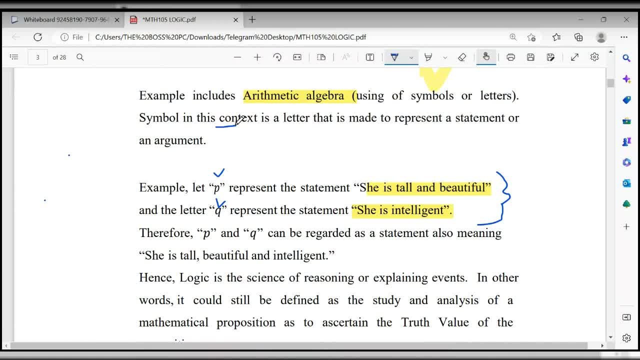 with they, maybe with the woman's call and stuff like that, singing, reading danger, so telling you that maybe you shouldn't encroach into such territory. that's a symbol, right, that's a a symbol. so definitely, um symbols. we have to represent something. all right, use of images. 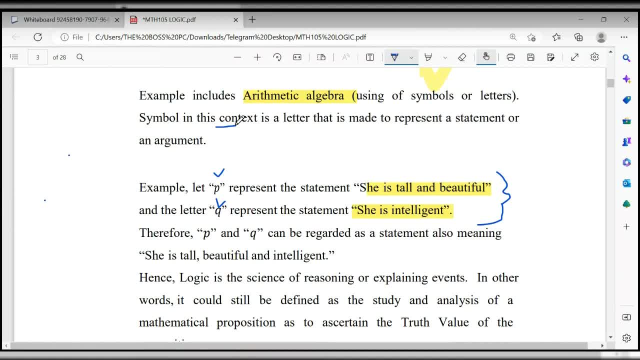 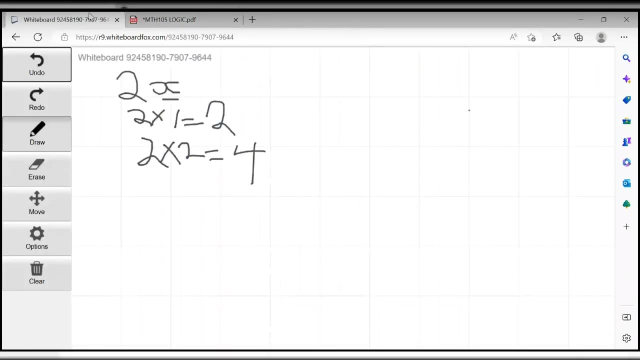 to represent something, um, to code some kind of information or instructions, all right, yes, so that is generally what symbols means, but in this case, the image that we are using. all right, the picture that you are using here is a letter. it's a word letter. so who can tell me the letters we have? 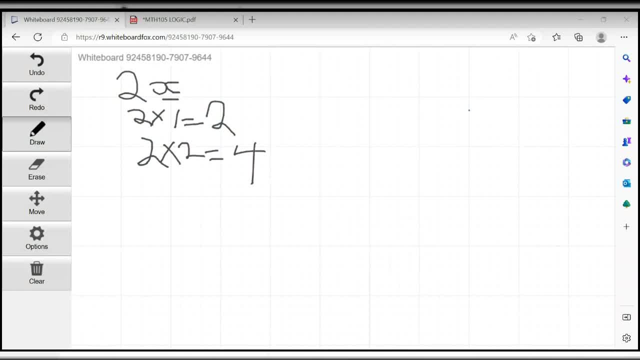 um, in english alphabet or english language, the letters are: what are the letters? which other letter do we have? we have y, q, q, q is a letter, a is a letter, p is a letter. okay, your a, b, c to z are all letters. so they say that you, when you use a letter to represent a statement or argument. 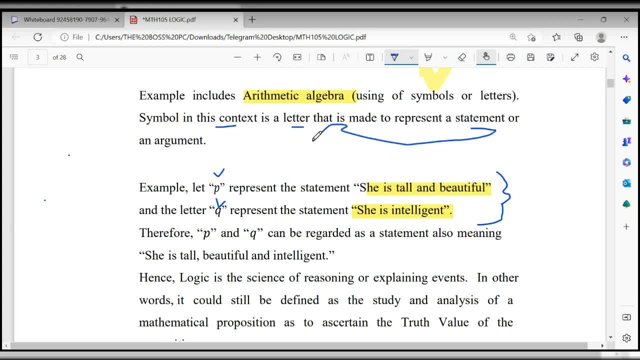 you are using a symbol. okay, so um statements or argument. we'll get to see states with that argument later, like, talk about them um, in on a larger scale much later. all right, so that is what they are trying to tell us: that you're using letters of the alphabet to represent. so that letter. 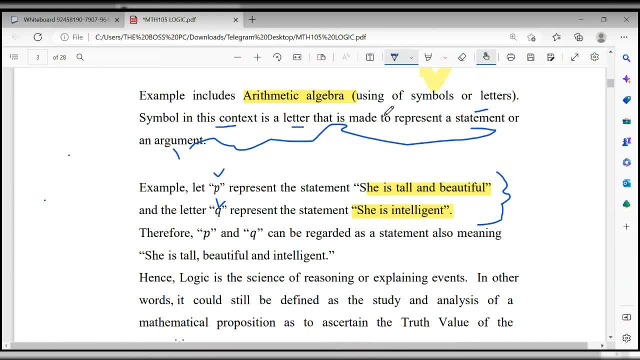 is not just their last song. lastly, if we just ordinary abc, it is representing something. the way that's now. maybe, um, your dad or your mom tells you to go to a location that they would have gone to. when you get there, you balance. you know normally if you go down your oh, maybe nobody. 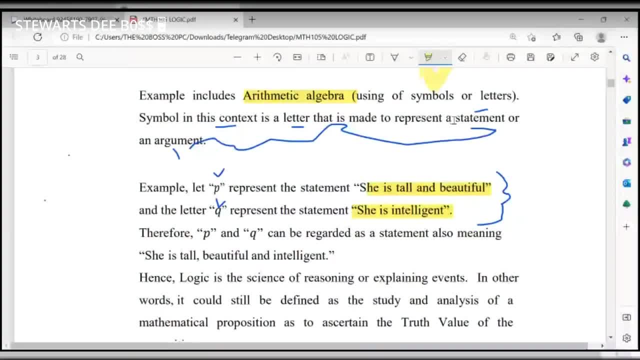 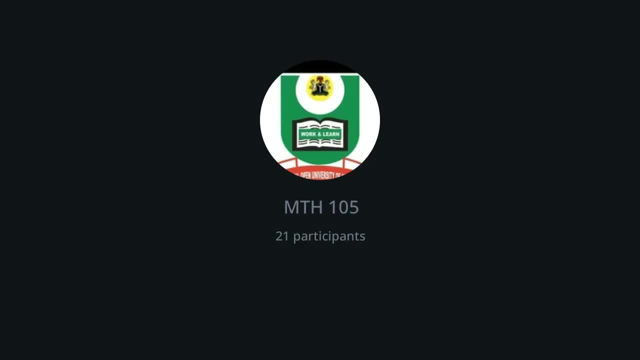 will recognize you. you'll just be somewhere in the background, but perhaps so that is very, very influential. or you know, i remember a very influential way that i think that will affect a lot of us. or you know, i remember very well when one of my uncle asked me to attend a wedding on his behalf. 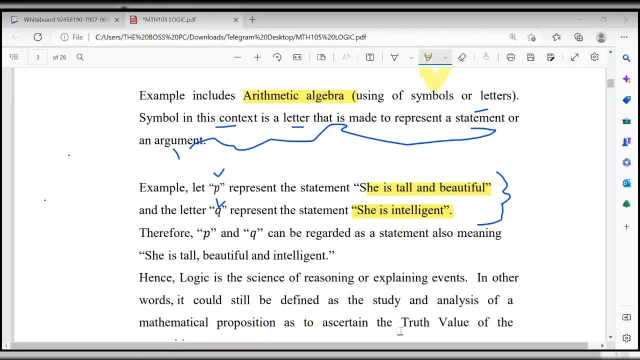 when i got to that wedding. i not carry second, like it was first position. i took that because normally i know my uncle is one influential kind of a person that if he was there will be on the high team. if i even called him on high table that day. you need to see me how i came. 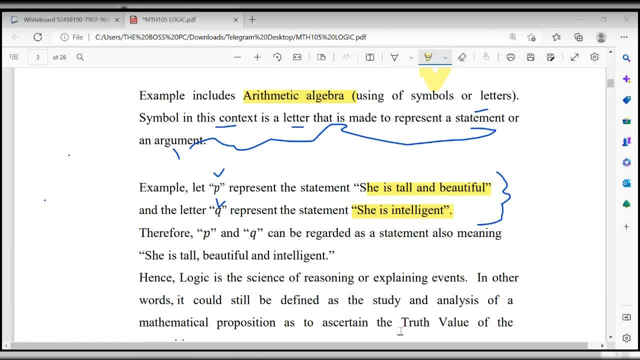 out how, with my swag and dignity and glorification to the front seat in the high table, i was sitting with timbers and calibers and i will not carry second. i wasn't just changing numbers with them, i was just in with them, because i know that i'm not just okay, i know that somebody sent me, so i 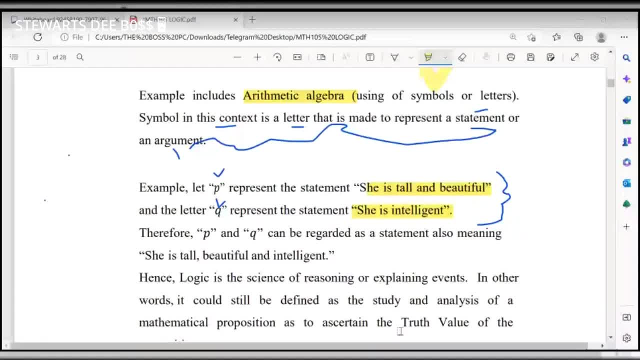 am there in the name of that person. just imagine you now going for an occasion and they invited you know they invited the president and the president said that okay, i cannot really go now. send you. you know they do it a lot. and then you now go there and start behaving anyhow. no now. 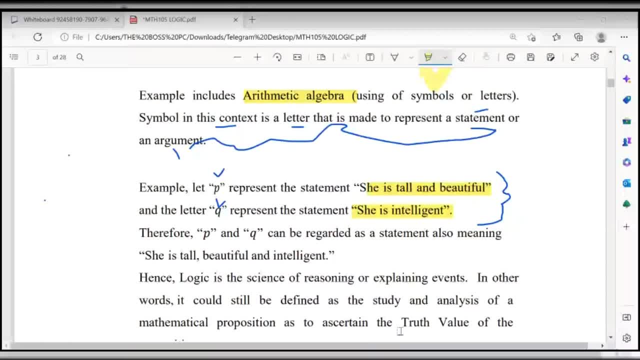 you carry yourself. that's as i've seen you, that's seen the president. because there's anything, you are coming there to give like that now. i gave them money. the money was not my money that i gave them. i gave them the money that my uncle gave me to deliver. so if there's, 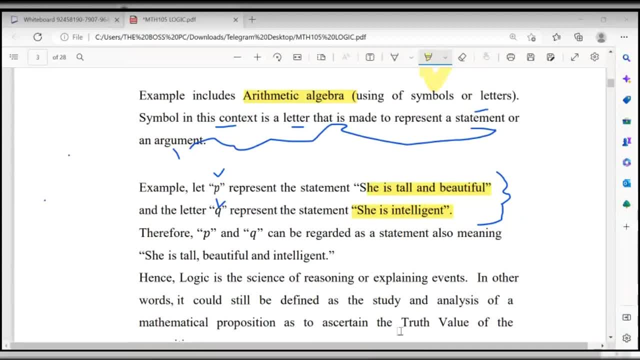 any message, there's any instruction, there's anything, i come here to deliver. you are giving it on behalf of the person that sent you. so if that person, um, is somebody big, you also look big. so that letter you are seeing there is no letter like well abcd, no, it's not for children, it is. 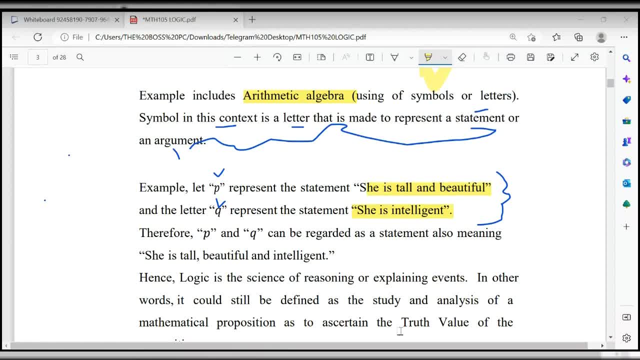 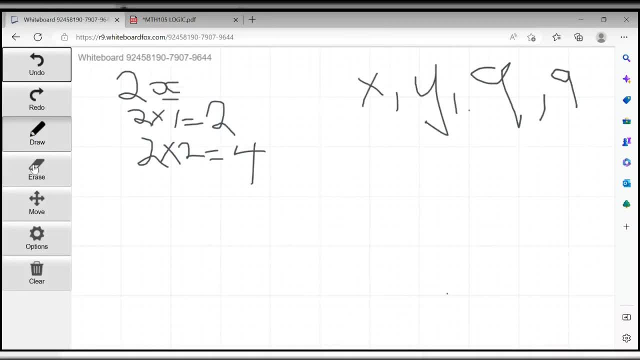 like: okay, let me just represent it in a simple way. that way i'm using it as a symbol. that is why i gave you that example i gave you earlier. you can see. they can see 2x. i used um. i used x. okay, as an example, i said 2x. i can use other examples. i can say, okay, um, 3y, all right, so if y should be 5, 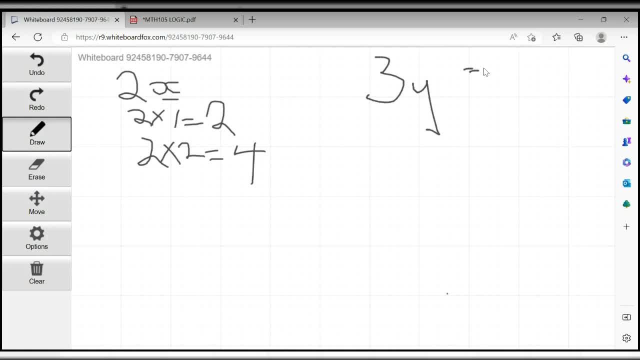 ordinarily this means that was 3y is equal to 3 times five, okay, which is equal to 15. all right, so if this, if y should be 10, it should be three times five. so this y now is what is a symbol, because it's representing something in this case, or representing five. 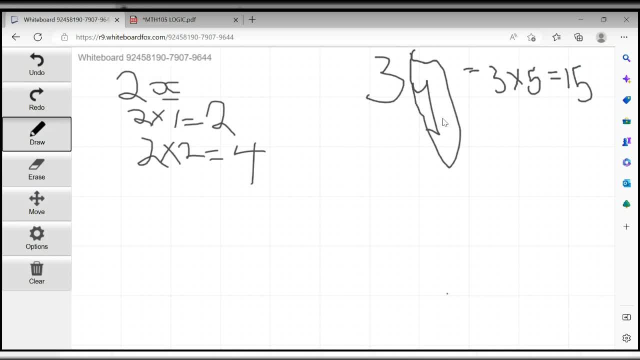 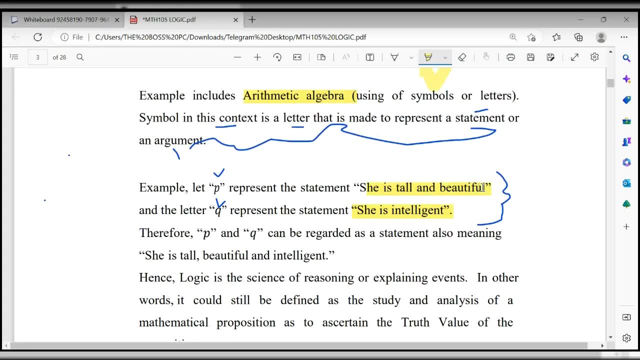 in other cases representing um 10, another case representing 20. okay, that's just it. okay, that's just it. if we come to this, please give us an example. let's say that this p representing she is thought in another example. in other situations p could represent the boss is the best teacher in the 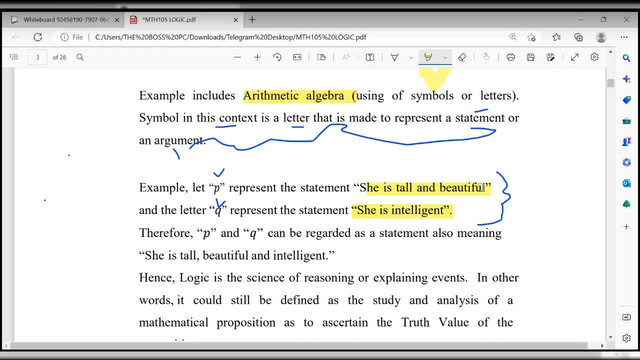 world, okay. in another example it could represent open university of nigeria is a wonderful school. in another example it could represent i am so hungry. in another example it could be: oh, she looks so tired. you know, it could be anything, all right, it's not by force, can she play? don't jump away. 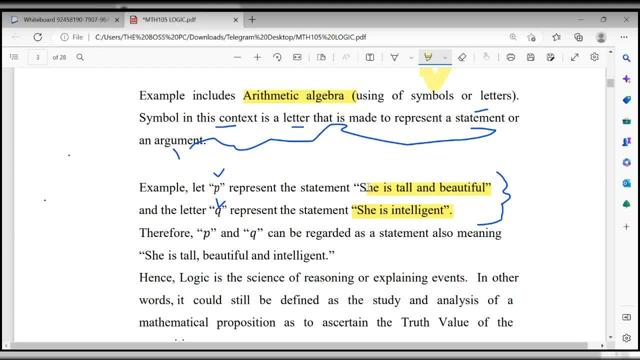 and because of it is mp represents. She stole Everywhere you see Pinot. it varies, all right. The main thing you need to know about Symbol is that it is where you use letters to represent a statement or an argument. So, Ms Isyoma, how about now? Are you cleared? Are you still lost? 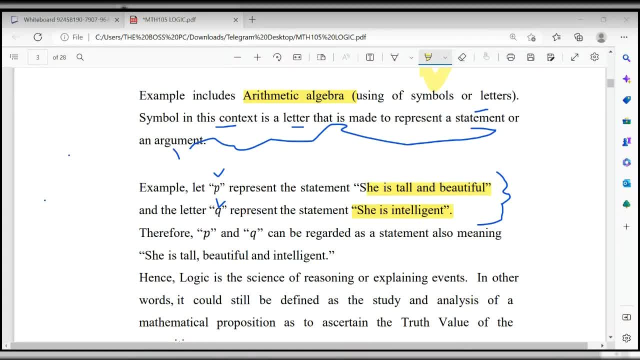 Are you still lost? ma, I think we have lost her, so let's continue, Let's continue, Let's continue, continue, continue. Okay, let's continue. Now we have a situation in our hands, So we are going to look at this better when we get to connective. 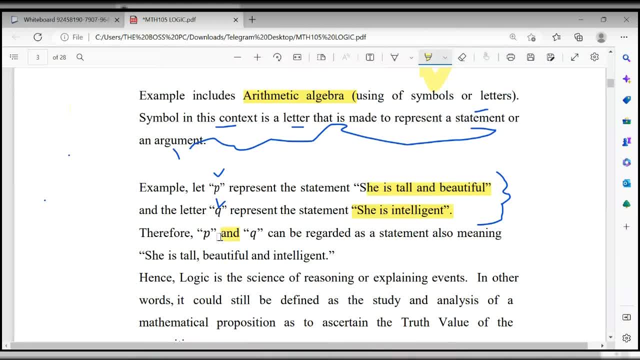 So you can see, here it says P and Q, So you are adding them together, all right, So how do you now express it? looking at this, So it should be what P and Q regarded as what she is, thought she's beautiful. 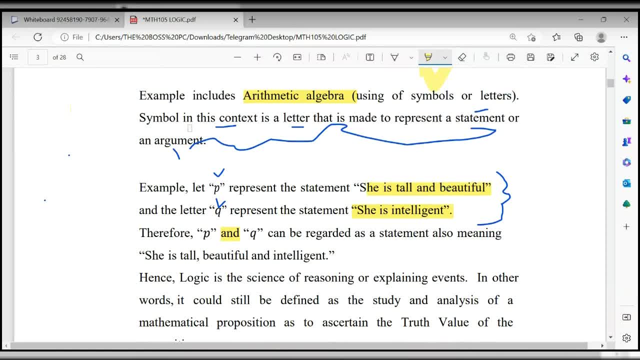 You know she's thought I'm beautiful is a statement. So in this case now you cannot say she is thought I'm beautiful And And Because they're using and to join it. So this and will be here. 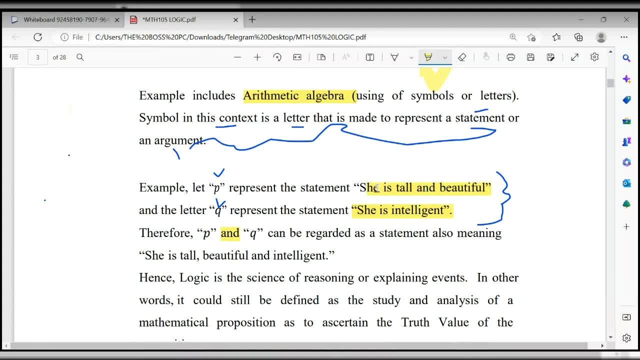 Just remove the and from here, Separate it by comma. all right, Normal English. I went to market to buy oranges, mangoes, pineapple, kwa-pao, kakumba and coconut. So the and will come before the last item. 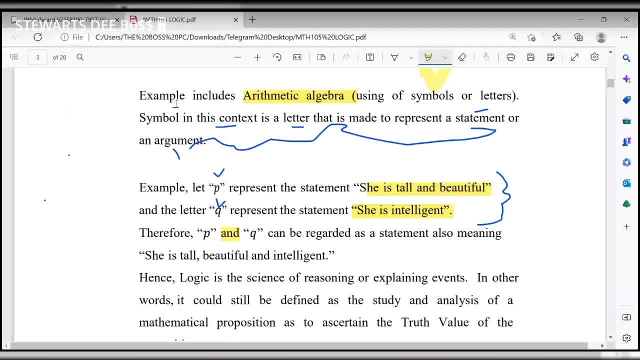 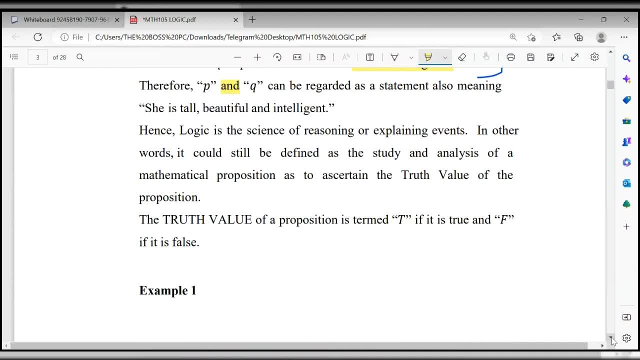 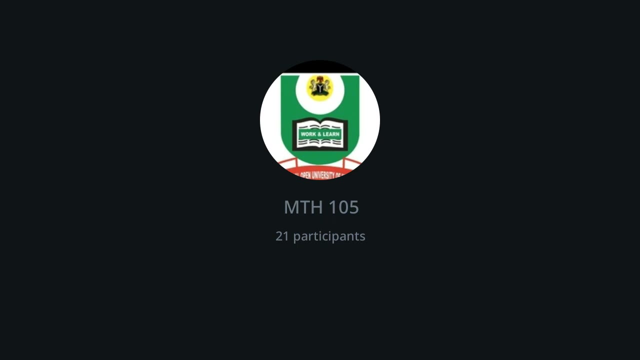 So that's just what happened here: So tall, beautiful and intelligent. Is that clear? Okay, this is clay. yes, sir, all right. so the last thing to this fight? yeah, it's logic. i would say logic, logic, logic, logic, very good. 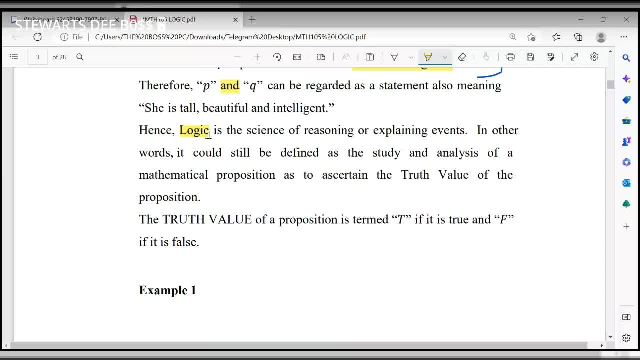 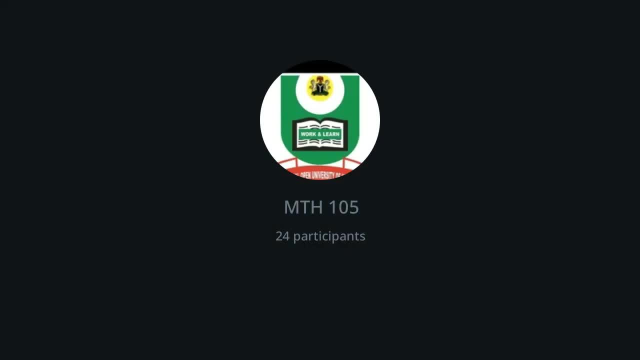 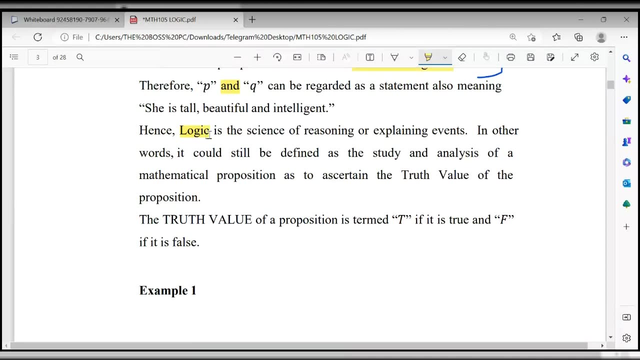 why are you laughing at the boss? why are you laughing at the boss? hey, you are laughing at the body, boss, of what i'm not places. are you lost? i can see your face. you are laughing at the boss. better you, thanks, because let me say something. all right, anyway, that just by the way. 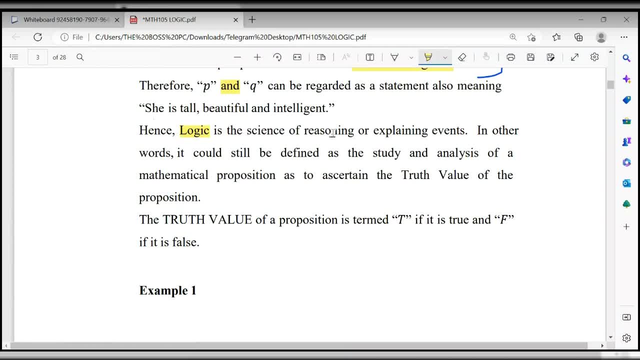 so um, hence logic is the word, the science of what's reasoning or explaining event. please. i talk about explanation before explanation, with um interpretation doing introduction. so reason means to think, all right, let's assume that, okay, fine, um, so you want to. so you want to. you buy your electric Deutsche мы. 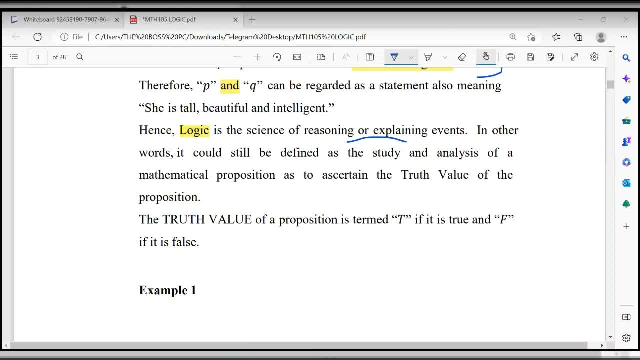 want to let you know how to learn, how to teach yourself, how to produce your communication, um, um, how to communicate your soul. you need to. the person could have been making some kind of sense, but you need to like think about it very. you need to be able to think and be like, okay, is this what is best for me? 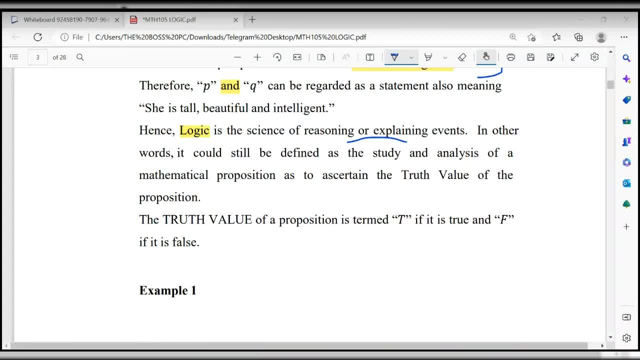 right? um, i'll be in a situation whereby people will excuse me, miss benis, can you meet yourself in a situation whereby people will want to um advise me? um, the boss do this this way, the boss do that that way? i mean no, no disrespect to them. um, mr tina janica, you meet yourself. 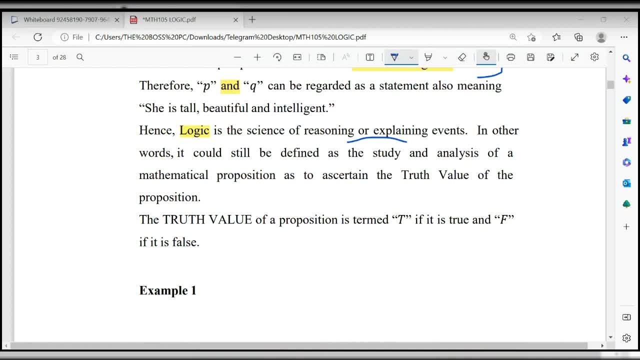 they are actually um making sense. they're actually making um lots of sense, but i still need to like be able to, you know, accepting whether what they are saying is actually the best. for me, that is reasoning. so when you are able to reason, you can be able to do that that way. i mean no disrespect to them. um, miss benis, can you meet? 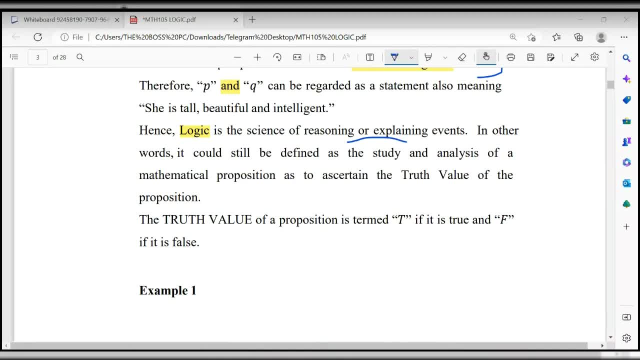 you can be able to think well, you can be able to, you know, define what is best for every situation. all right, it is logic. that makes it impossible, because, if you look around most of the courses you guys have been doing, i've been talking about being objective and many things like that. so 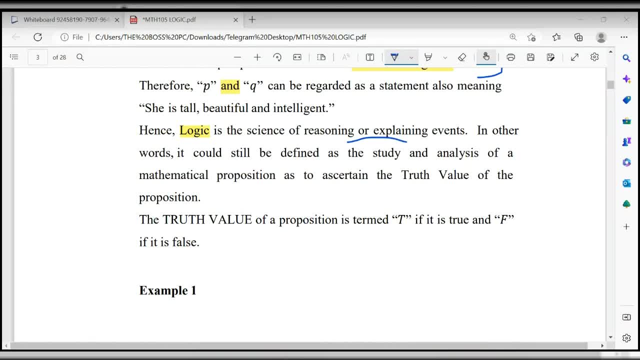 logic will help you. all right, they've told you: okay, this person, um, is doing this, this thing is happening here, it's happening there. final good, you should be able to see them and now know. okay, after everything is said and done, what is actually the best for me. all right, and then you should also. 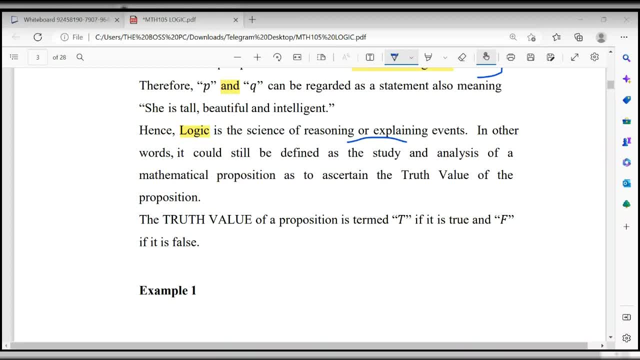 be able to explain events. so, apart from thinking and making decision, when it comes to painting a picture of what happened okay to people, logic helps you to do that and do it very, very well. i'll be able to tell people that okay, and i was in the class today. look at what happened for. 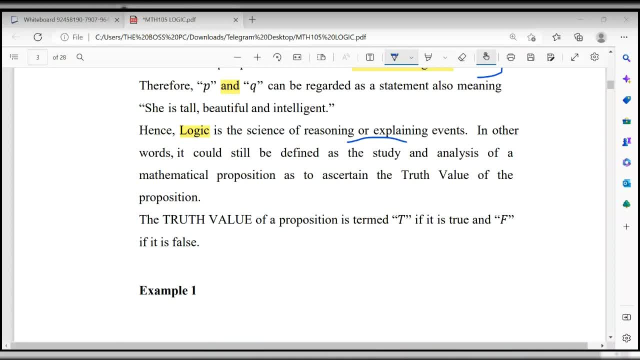 example. now, most times i get situations whereby students can have some kind of issues with themselves and somebody is like trying to, maybe because that person has a friend. you know, sometimes it can happen. the friend of that person is involved. you now want to start. you know, saying things the way, 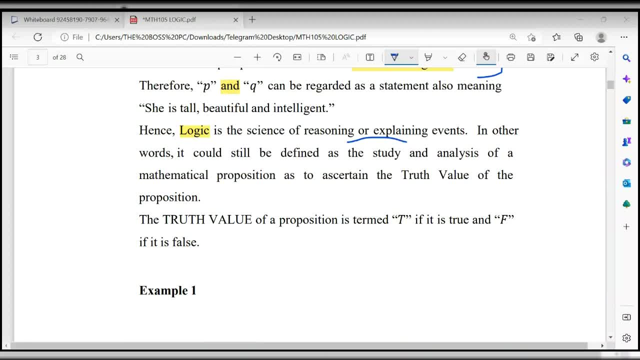 they are not. just because you want to favor your friend and someone else, that is logical. we call my person. doesn't even care whether you are a friend or not. just say that this is what happened in this case, who. i think you are the wrong person. you know that kind of situation so 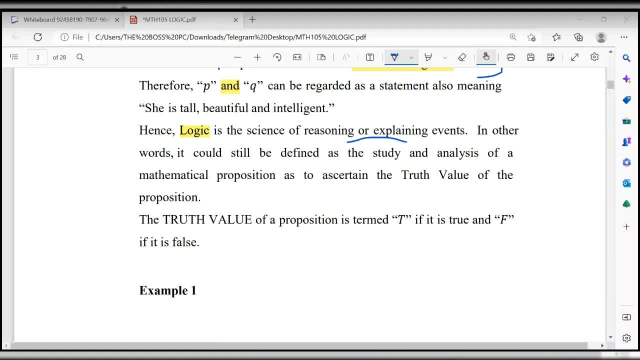 it and then maybe somebody is trying to like say to you guys, and the person can comes into the scene and it's like what is going on? the boss, look at what happened, what happened? you can be able to say the thing the way it is why? because i've been logical. 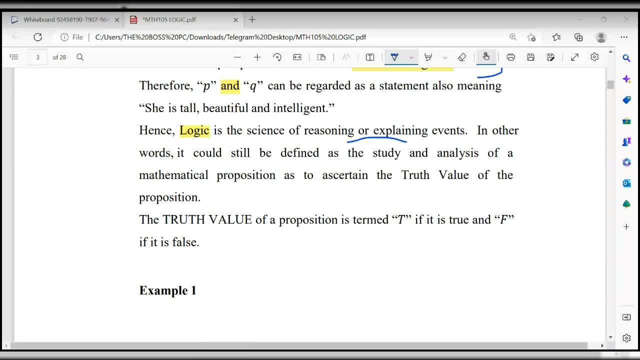 so it helps you to what to reason and explain, and you can only do this scientifically. that what they say is the science. okay, there are many ways that you can be able to reason and explain things. sometimes we, we can explain things and reason from the perspective of the scriptures. most of us are. 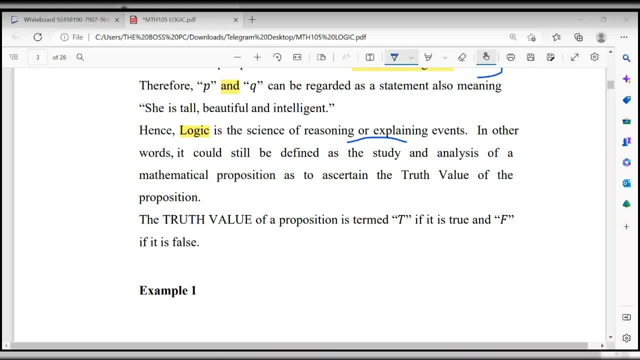 like: oh, the way, it is why i'm doing this. why don't you want to marry that man? well, my pastor said that he's not. i should not marry him. why don't you want to marry him? my spirit do not really agree with him the way he's behaving. i don't really like it. okay, um, why don't you want to marry her? 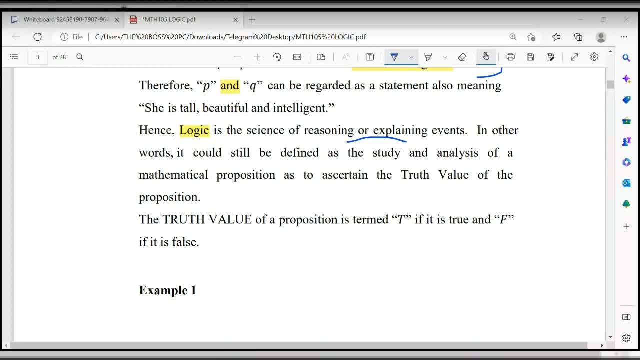 i come from my place. you know it does not usually marry people that people that might be from day my own family. they are not really enjoying that marriage like my own family. now, that's some kind of like. i have an uncle that i'm married from somewhere i don't want to mention. 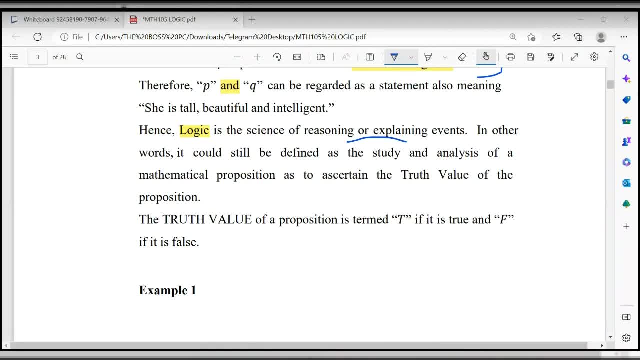 the people, because people from there are in this class and the marriage is not really sweet like that. so all of us that are growing up, i think, also, don't marry this person. no, don't marry a lady from this place, nobody from that place. let's say tomorrow, now, somebody now falls in love and the 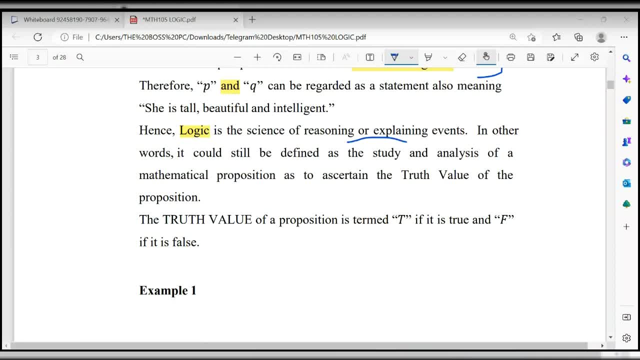 person is from that aspect for that area and the little nasty- i'm not married, why my family that one is not- is not scientific, it is based on other things. so it is not um, you can reason your basis and you can understand it and it is not just a relationship between you and that person. 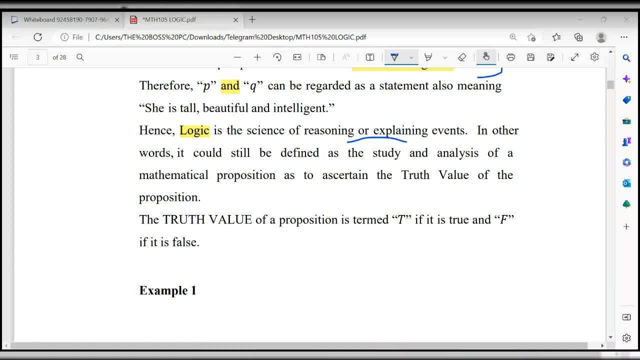 that is why i say in the early stage of your brain, why you realize the next things that happen right, because that person is not only the one that you're going to like but also the one that you want. so that's why i say: don't marry that person, because you know that person is a little bit. 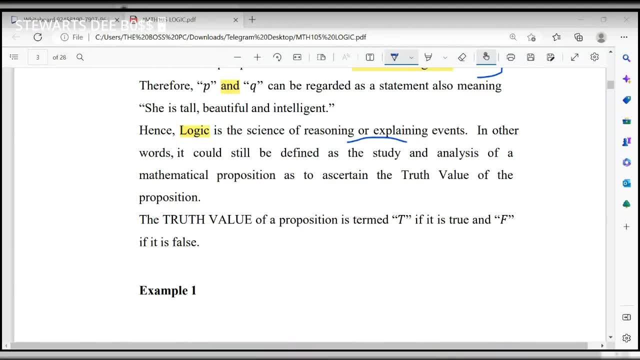 different now, it's less than you. i think you have to start believing that that person is the one you're going to like. that is very important, right? that's what i'm saying. you might be saying, hey, this woman is a little bit different from this person. she's black, is a little bit different from 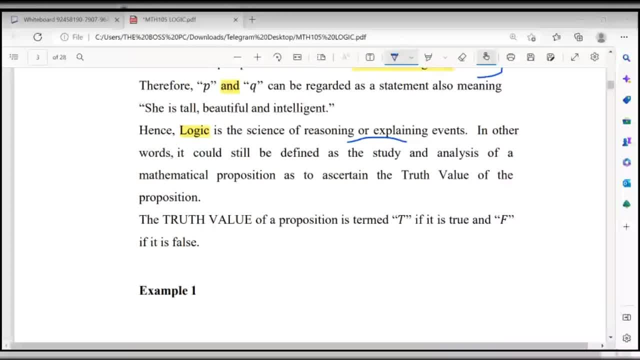 on what is going on following. i say that if you actually reason and explain events through other means, okay, it is not. you know it is not logical. once it is, then it is logical. let me just believe that you do not hear me. well, that's why you are able to respond with the class. yeah, thank you. 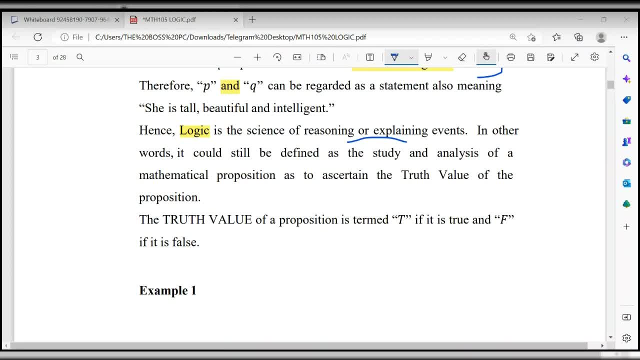 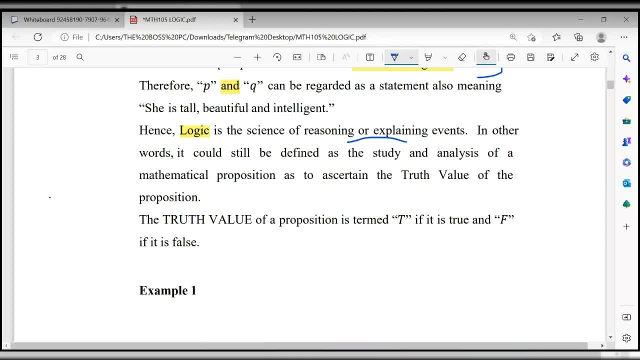 now, when it comes to logic, there are something you need to understand and, um, it has to do with what analysis? okay, has to do with what analysis, analysis of what, the true value of every preposition. so, once, as i said, once it everything is being presented, or? 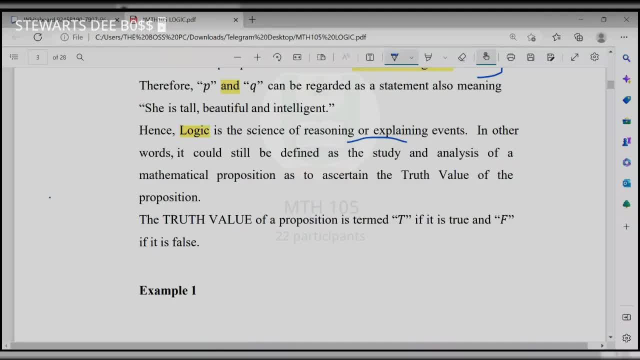 right. you need to what you need to be able to make good decision, rational decision, and this decision has always been influenced by what the true value of that preposition. so if someone is telling you something that is blatantly a lie- erotic, this one is a lie. it's a blue light. it's. 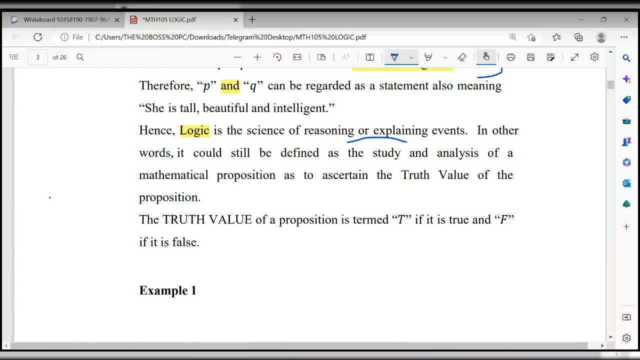 a white light, yellow light. you will not accept seeds. you cannot assess. you will be like: i am smarter than this, but if the thing is actually true, then you know. okay, fine, even if anything goes wrong, it is not because of this person deceived me. i'll give you an example. you come to the class and i'm teaching you. 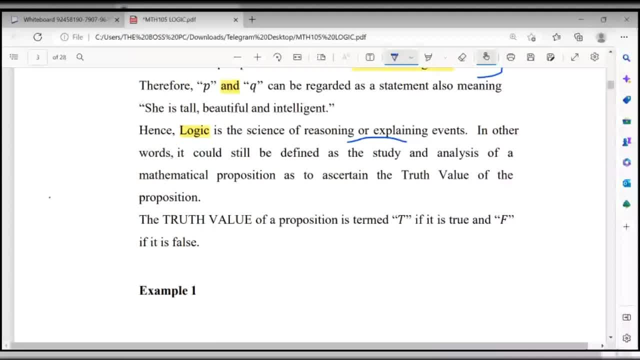 as far what i'm teaching you, you know that is the correct thing. i'm teaching you, right? okay? whether you pass the course or you not pass the course is now dependent on other factors perhaps. maybe how fast you can assimilate, um how distracted you were during the class. 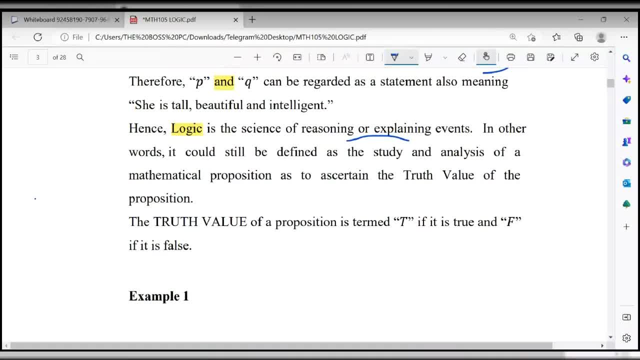 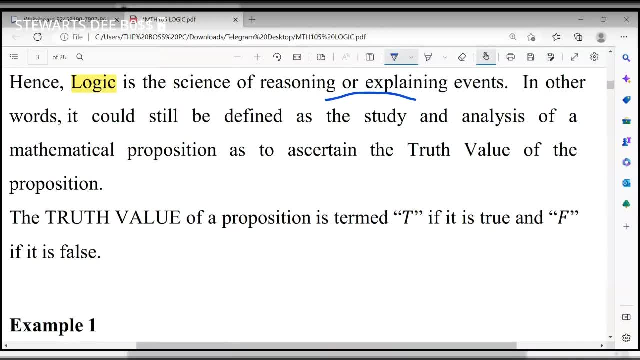 many other things will really come into play to be able to determine whether you're going to pass or not. okay, so you want to really just make a decision: whether to join my class, subscribe for my classes. you know, the first thing you want to know is: is that, is he actually teaching well? 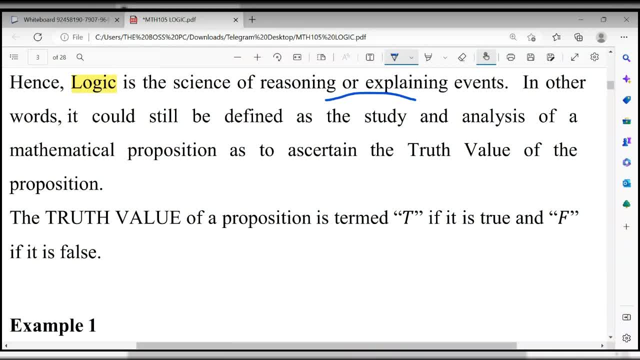 what? what is teaching? what he's always saying? is it how it is? so once you can know that, okay, definitely you should be moving. you know, in, except either other reasons, you know, for example, maybe money or other reasons could come in and now be taking you to other places. 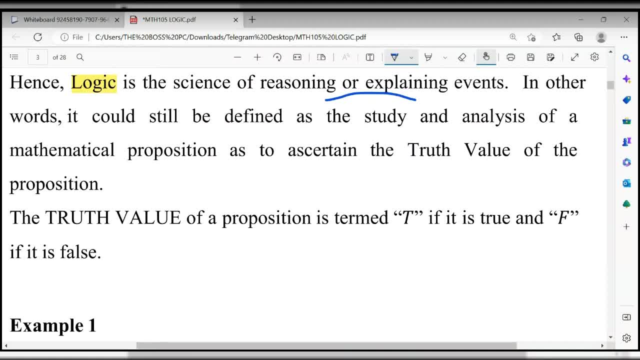 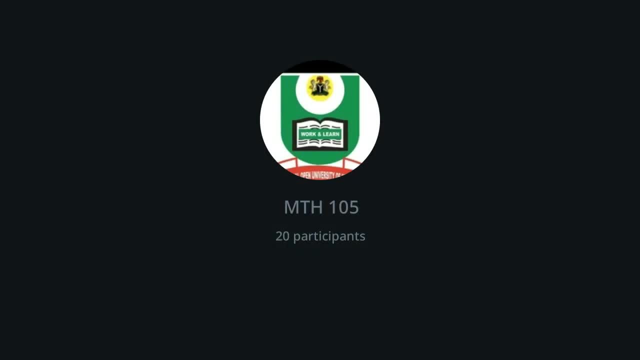 so that is what um logic has us to do, because you need to know the truth in everything. the truth is actually very, very instrumental. once the truth is there, okay, every other thing is very, very instrumental. okay, every other thing is believed to be able to fall in place. now, in logic, the true value of a. 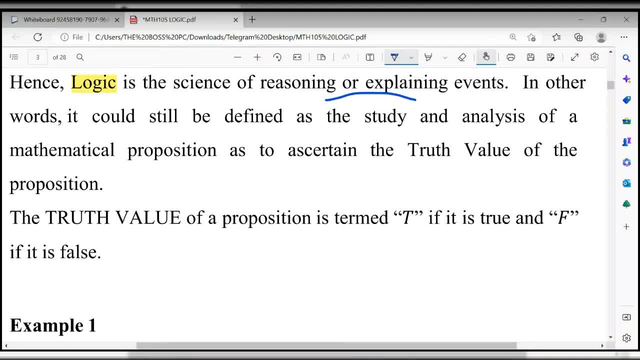 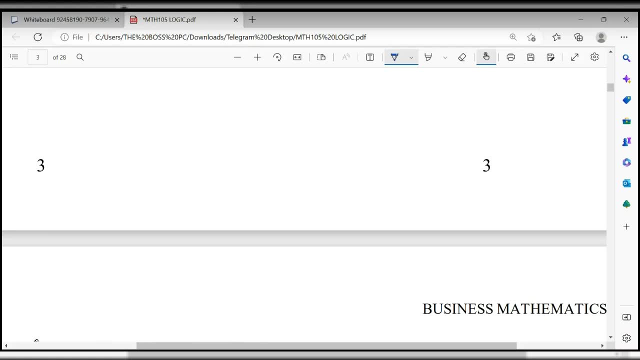 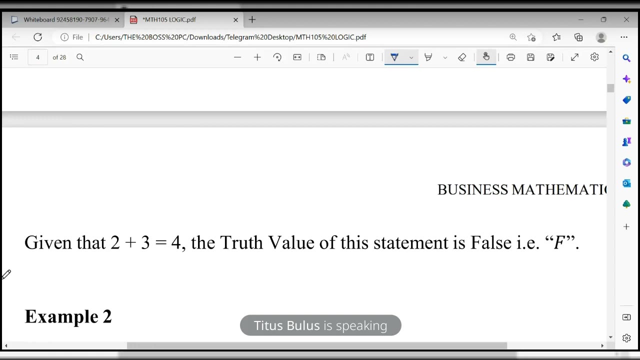 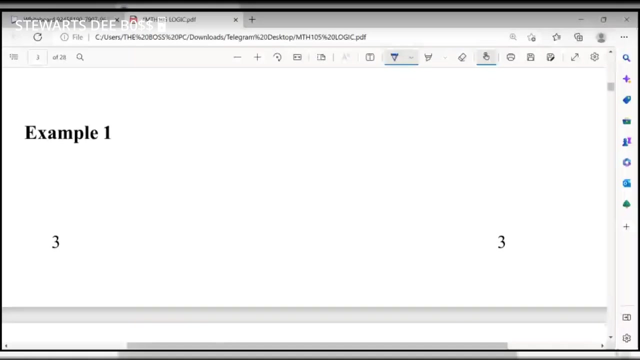 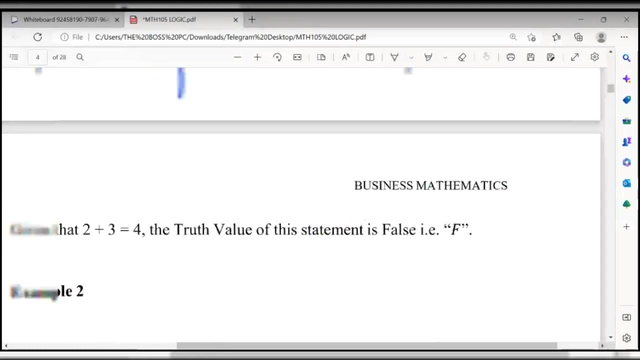 progression is time t, and when we don't have the truth, we have force you time it f. and then there's an example for us to look at and digest. okay, uh, i want to see. yes, who is that? so we have an example here. they said, giving that two plus three is equals to four. 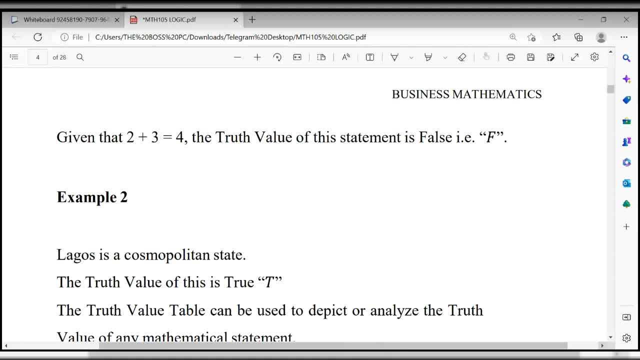 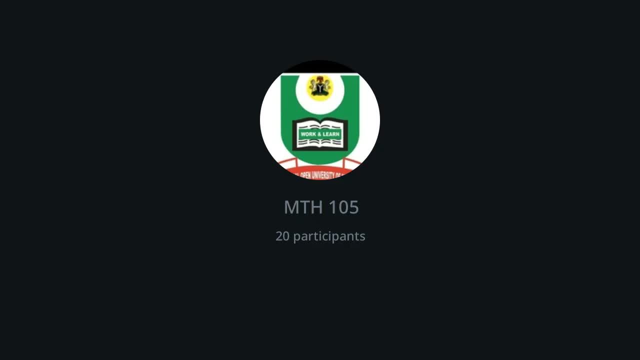 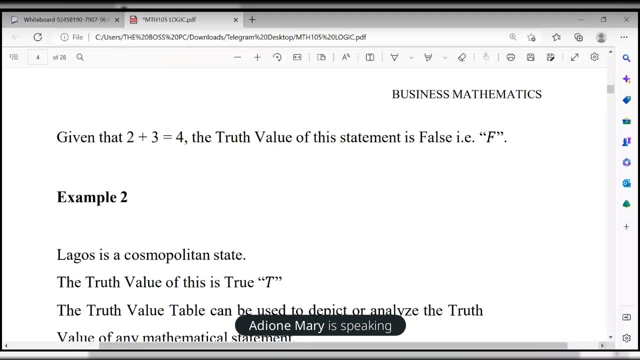 what would be the true value of the statement two plus three? when you work it out, you're going to have five. so two plus three is obviously not for them. is first, please. these people are pointing our, our class for us. now people are going to use the replay. 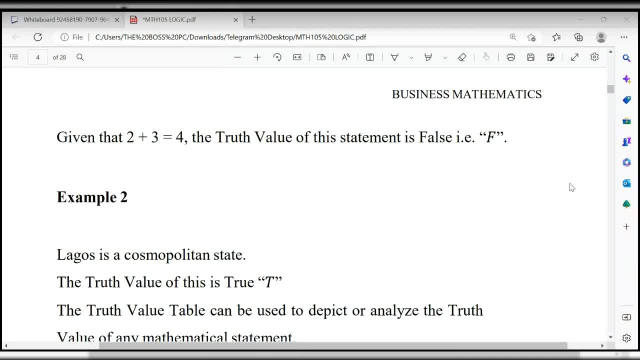 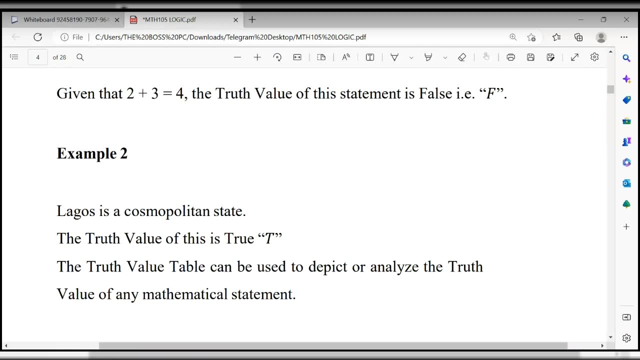 if you're in a noisy environment, don't meet yourself. only on mute yourself when you know you're in your quiet. please only omit yourself when you're in a quiet place so that when we post the recording to make sense, all these interruptions- you make people to be very tired of the um of the video when they are. 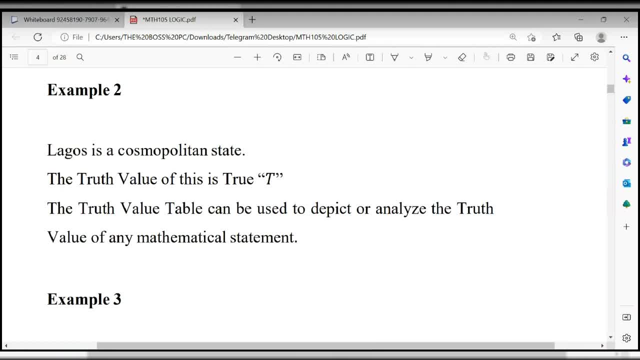 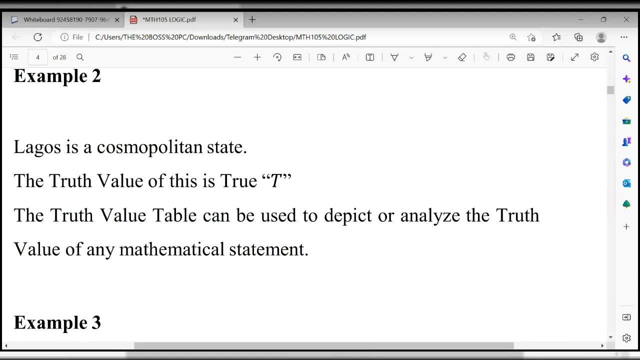 watching it. so please, i beg us, meet yourself, even in a noisy environment. now we have other examples. now lagos is a cosmopolitan state. now, when we say cosmos political, who can tell me what it means? i told us in the last class, so i expect everybody to be able to answer it. cosmopolitan states. what does that mean? so cosmopolitan states is that kind of a state where you have a place where you can have space and, at the same time, you have space to interact with others, have, virtually, yes, um, our tribes. okay, so many tribes from all over the world. okay, that is. 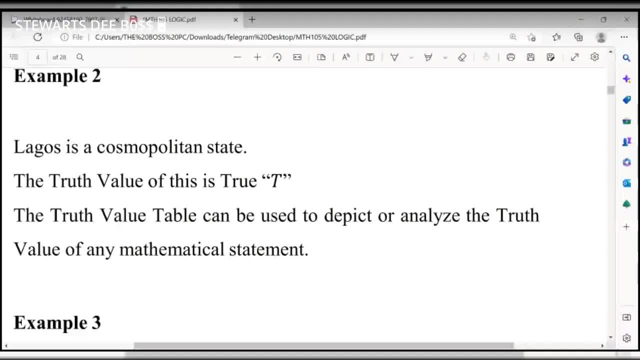 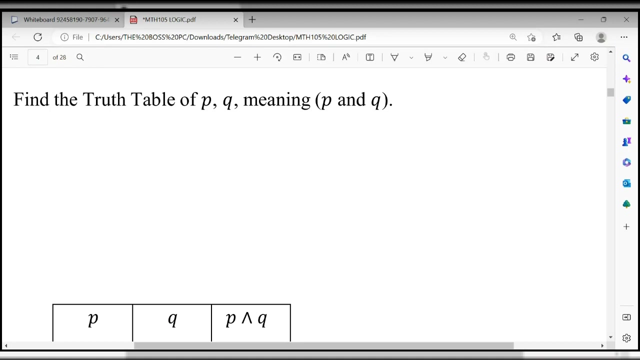 so thank you so much, mr. yeah, you are correct. so you can see that. yeah, in lagos we have people from all over the uh, all places, okay, so he's actually not out of place to say legacy states. all right now, find the true value of pq, meaning p and q. 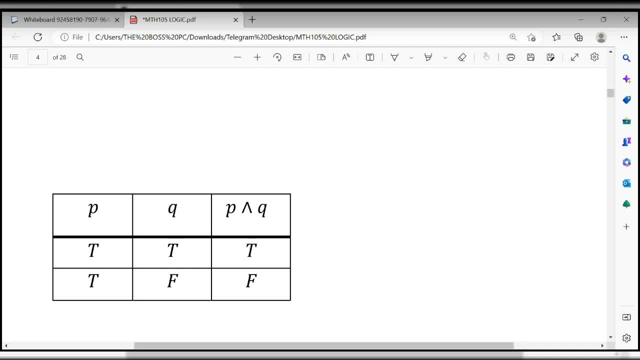 right. so we want to find the true value of p and q. now, mind you, p and q could be any statement, okay, it could be any statement at all: um. so p could mean um. p could mean i am in the class, all right. you could mean um, i am eating. 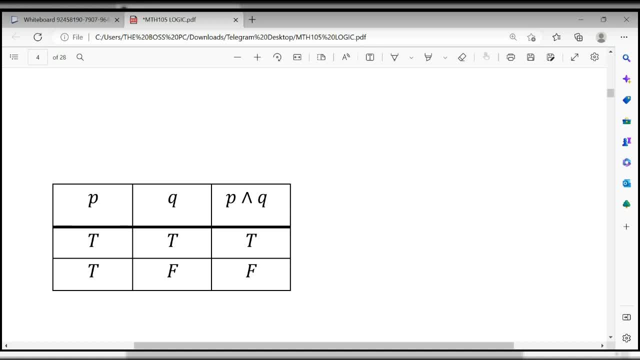 so now p and q with them together. to me, um, i am in the class and i am eating. now, if you are in the class for real, it makes p true, okay, because, yes, you are truly honestly speaking in the class, but let's assume, um, that you are not to be in the class. definitely, this will be false, okay. 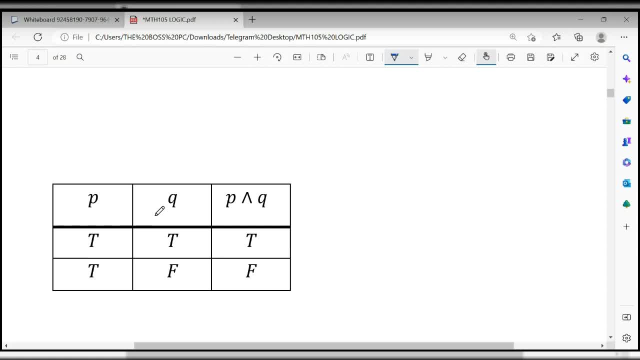 now, if you are to be eating like legitimately as at that time, then this would be true. and in a case where both of them are true, this becomes true because this is very, very simple: if i, if someone comes to your house and you tell that person, um, that you can afford to offer them bread and tea. 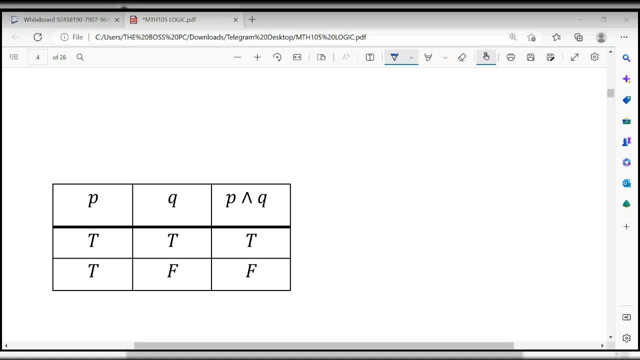 now, if indeed you have bread and tea in your house, that is when you can be able to offer it to them. if you have bread and tea, like, the two options are available, so you you possibly can just go in and make the provision. all right, if you want to eat rice and 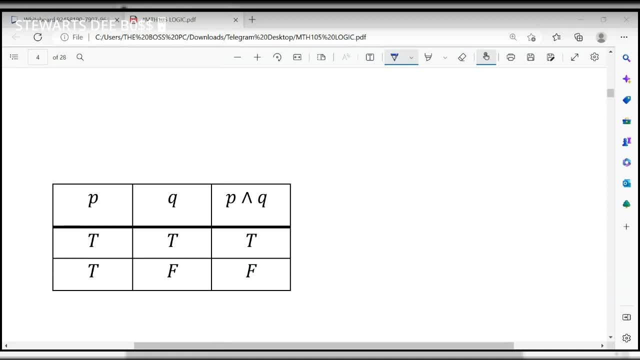 beans and rice is available, beans is available, then it's all good, it's all beautiful, you can be able to um, you can afford to get both of them. because of what? because they are there. the two options are there, but if one is not, is not available, you can't get both. 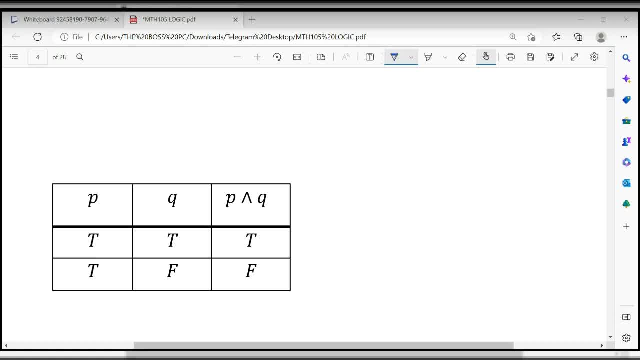 again because and means that two of them are available. so if you have only rice and then saying that you are going to give the person rice and beans becomes a lie. that is why, in this second option, you can see that once one of them is forced, the final um um, you know. 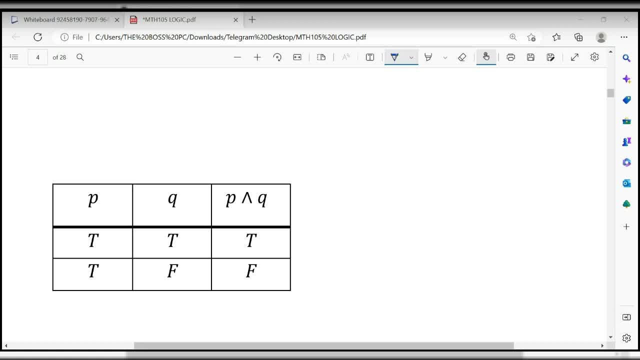 preposition becomes a force right, but let's assume that this one was all right. we have p or q if i tell you how to give you um tea or coffee. so let's assume i have coffee, like coffee is in my house, but there's no tea. if i tell you tea or coffee. 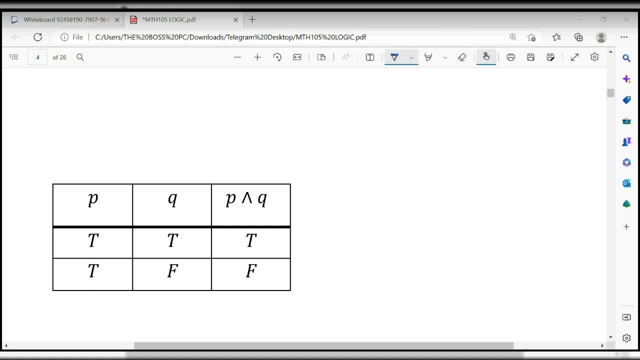 it's still correct, because at the end i'm saying tea or coffee doesn't mean that you need to take both of them. if it is only one you can find, then you should be okay. that is what that is saying. okay, but when you say and and means both of them. so if one of them is forced, everything becomes first. 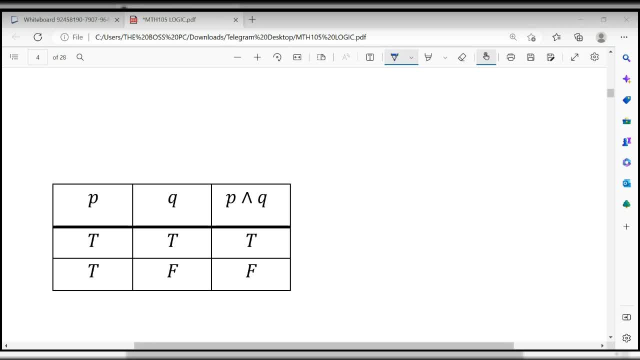 but if you say um, or except if both of them are. first, if i say tea or coffee and i don't have coffee, i don't have tea. there's no way. i cannot find any of them. so i have been lying all right. so that is just what you need to know. we'll talk about. 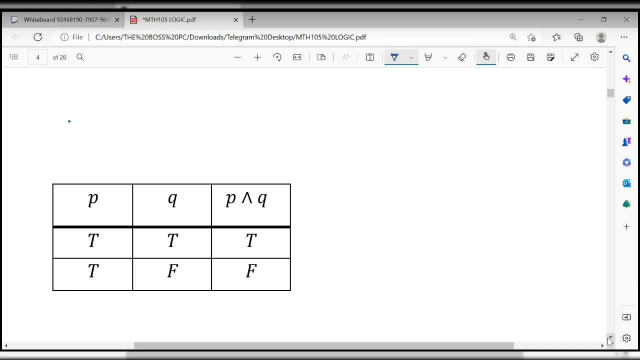 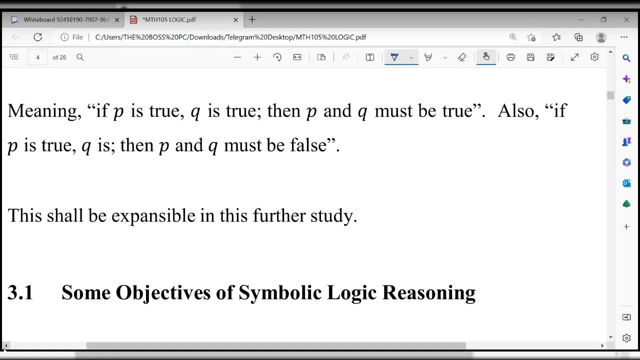 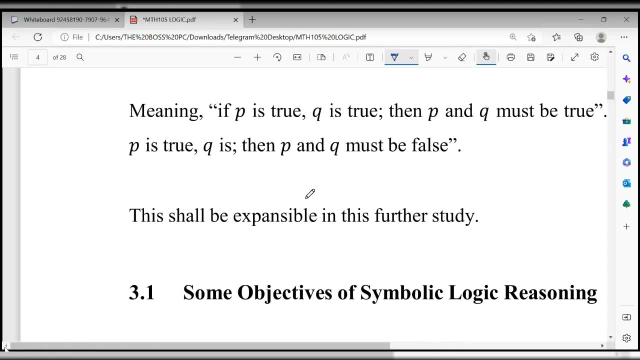 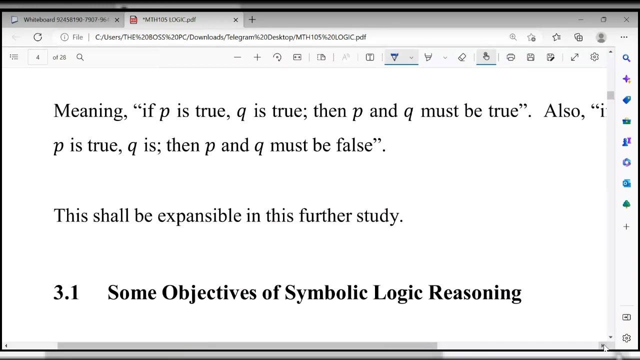 we'll talk more of this when we get down to that part where they talk about um connectives. okay, connectives, connectives, connectives. so i think what i've explained is what they just talked about here. so let's take up. we're just saying something. i hope you're noticing. 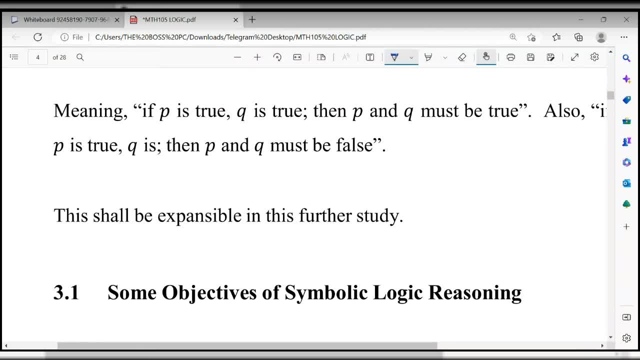 something. so, um, these ones i've explained um so far, um tomorrow, let's see tomorrow. um miss, yeah, okay, i think, yeah, tomorrow these ones i have been explaining so far. miss i've bought. okay, i think, yeah, tomorrow these ones i have been explaining so far a day. hope your life you will. 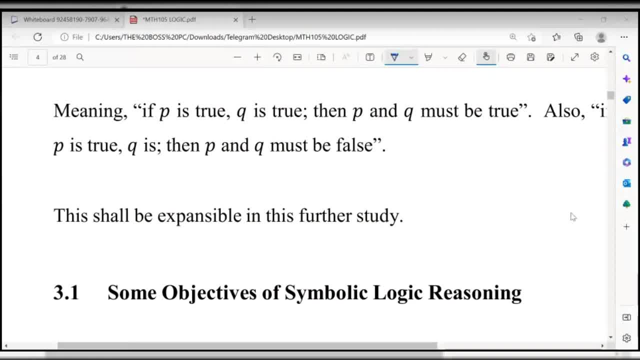 a day, hope your life. you will a day, hope your life you will um, um, um. do the summary and review, do the summary and review, do the summary and review for us, for us. for us, okay on our platform, okay on our platform, okay on our platform. then, 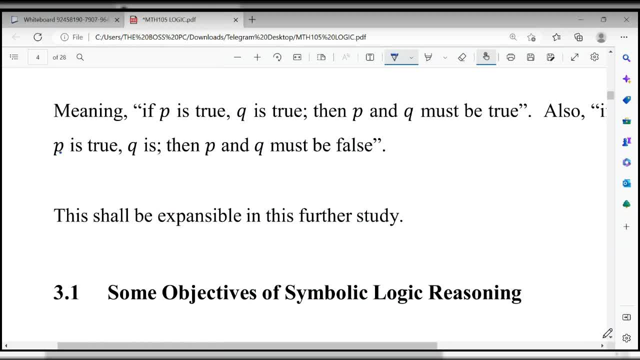 then, then, before the end of the class i will mention. before the end of the class i will mention. before the end of the class, i will mention the second person that we also the second person, that we also the second person, that we also um do something. and after tonight, some. 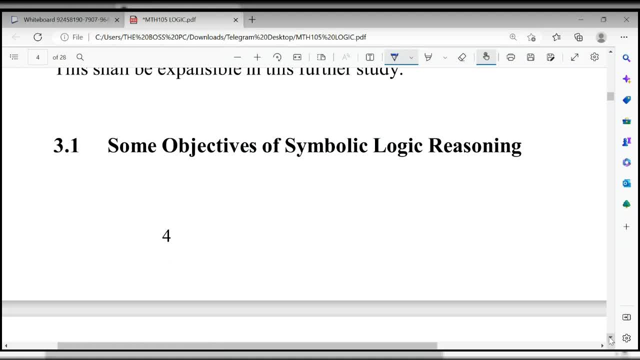 um do something, and after tonight some um do something, and after tonight some. gst107 class as well. i will call out gst107 class as well. i will call out gst107 class as well. i will call out some people, some people, some people to also um. to also um. 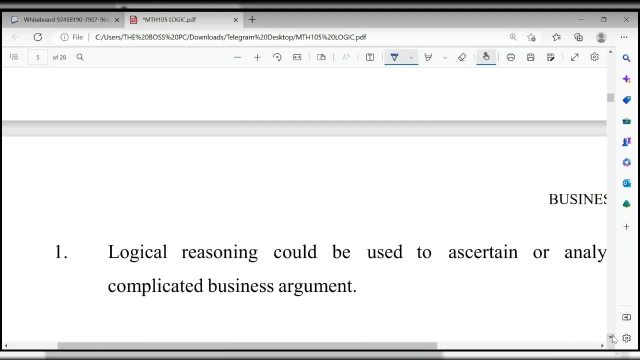 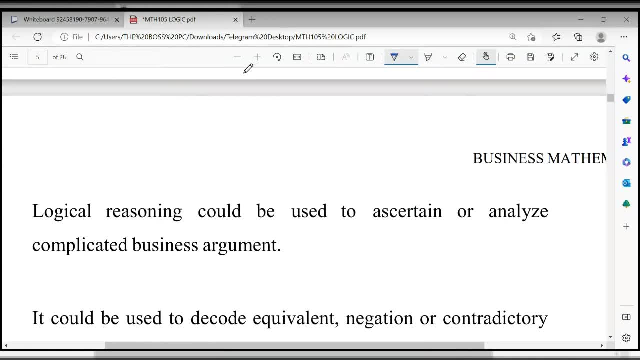 to also, um, you know, you know, you know, help in our help, in our help in our follow-up, follow-up, follow-up exercises, and please so keep reminding your and please so keep reminding your and please so keep reminding your colleagues that you should subscribe, colleagues, that you should subscribe. 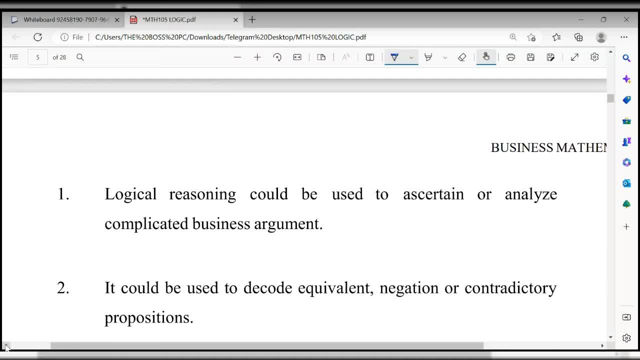 colleagues that you should subscribe for our classes. i'll be inviting them to for our classes. i'll be inviting them to for our classes. i'll be inviting them to class as well, class as well, class as well, okay, okay, okay, it's because they know how. it's because they know how. 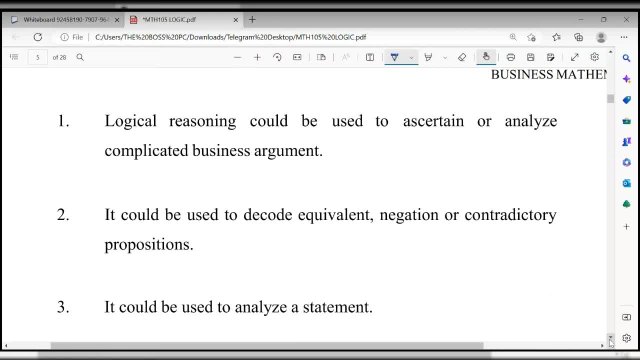 it's because they know how they want to do it. they really need these. they want to do it. they really need these. they want to do it. they really need these. meetings, meetings, meetings. the frustration on the school is only for. the frustration on the school is only for. 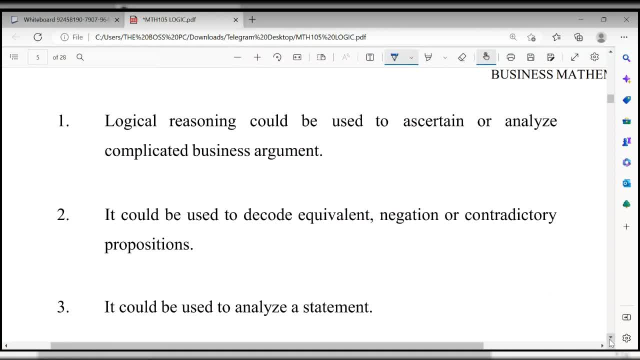 the frustration on the school is only for a few weeks, and even after the weeks. a few weeks, and even after the weeks, a few weeks, and even after the weeks: um, um, um, no, all the course material will not be. no, all the course material will not be. 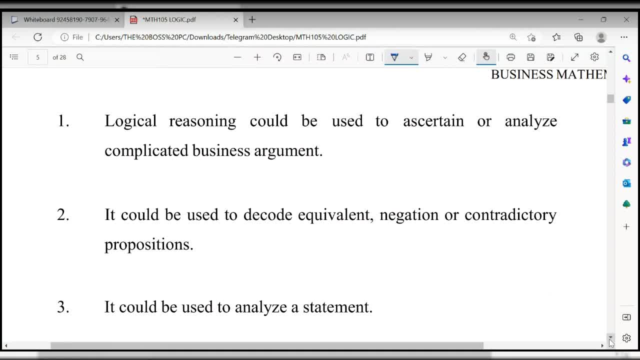 no, all the course material will not be covered and all the courses will not be covered. and all the courses will not be covered and all the courses will not be covered, covered, covered. so it's good that we start getting. so it's good that we start getting. 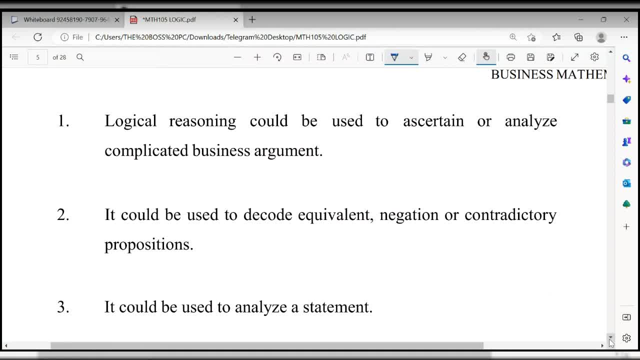 so it's good that we start getting serious here, so that, serious here, so that serious here, so that by the time other students will be, by the time other students will be, by the time other students will be joining us, they'll be meeting us, joining us, they'll be meeting us. 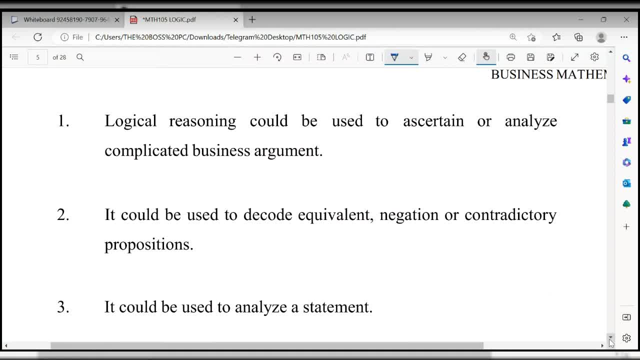 joining us. they'll be meeting us. established, they'll just fit in. established. they'll just fit in established. they'll just fit in when we are not organized and we don't when we are not organized and we don't when we are not organized and we don't know what we are doing. 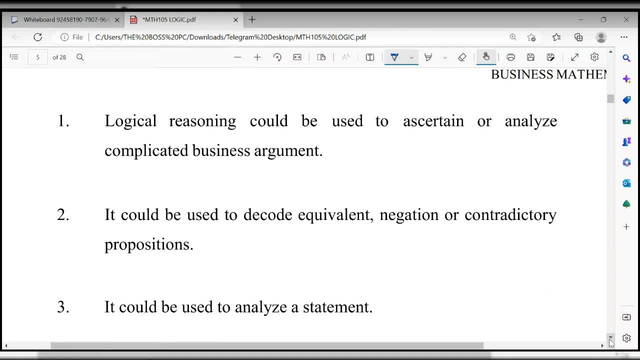 know what we are doing. know what we are doing. other students will come in and you'll other students will come in, and you'll other students will come in, and you'll just be lost. just be lost, just be lost, because everywhere is just a shambles. 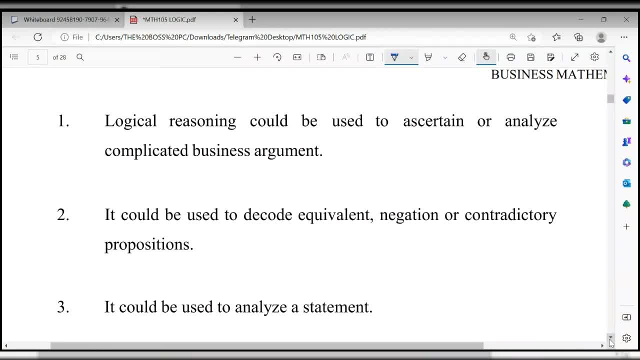 because everywhere is just a shambles, because everywhere is just a shambles, but but but i've never had that experience whereby i've never had that experience, whereby i've never had that experience whereby the students i work with are not really the students i work with, are not really. 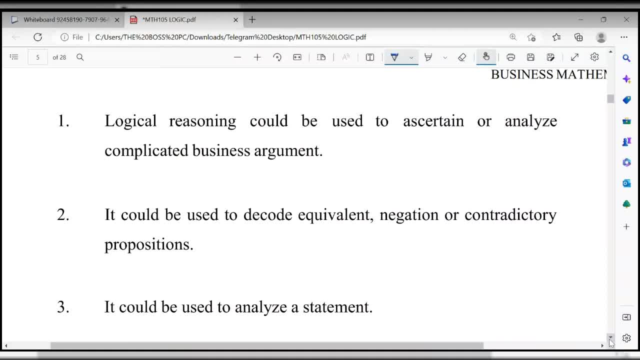 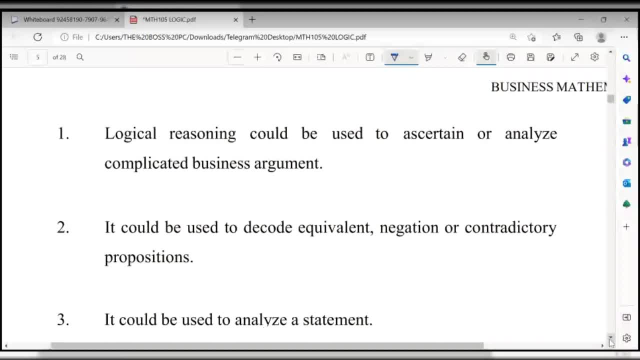 the students i work with are not really organized because organized, because organized because i'm always ready for them- okay before. i'm always ready for them, okay before. i'm always ready for them, okay before they come around. they come around, they come around now, now. now we are going down to objective, or 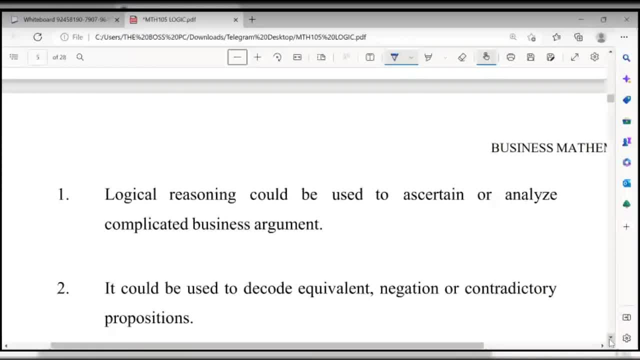 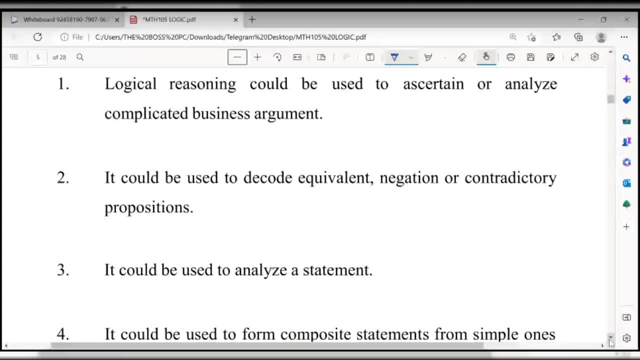 we are going down to objective, or we are going down to objective or symbolic logic reasoning. symbolic logic reasoning. symbolic logic reasoning. okay, okay, okay, now one, now one, now one. logical reasonings could be used to. logical reasonings could be used to. logical reasonings could be used to accepting or analyze complicated. 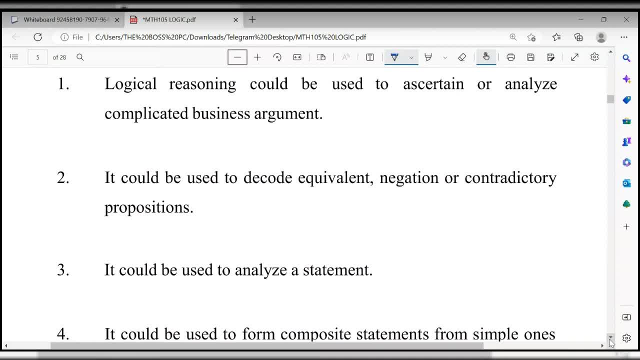 accepting or analyze complicated. accepting or analyze complicated business arguments. business arguments: business arguments: logical reasonings could be used to. logical reasonings could be used to. logical reasonings could be used to assertive or analyze complicated assertive or analyze complicated assertive or analyze complicated business argument. that is one. 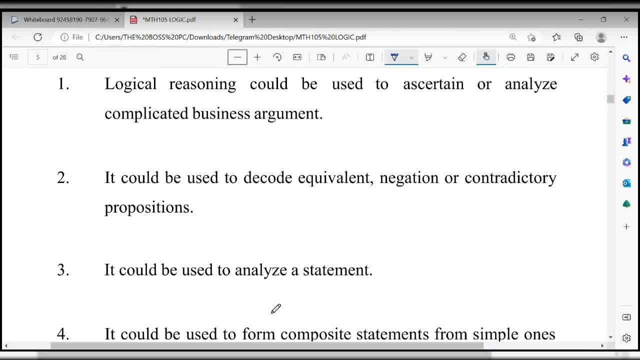 i think i have to invite somebody now. i think i have to invite somebody now. i think i have to invite somebody now to, to, to talk, talk, talk. explain to us what he or she understands. explain to us what he or she understands. explain to us what he or she understands by this. 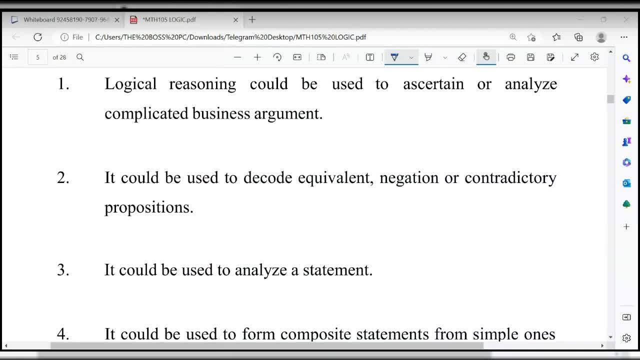 by this, by this statement, let me come to you miss faith statement. let me come to you, miss faith statement. let me come to you, miss faith, miss faith, good evening. how are you doing miss faith good evening? how are you doing miss faith good evening? how are you doing faithful good evening? can you hear me? 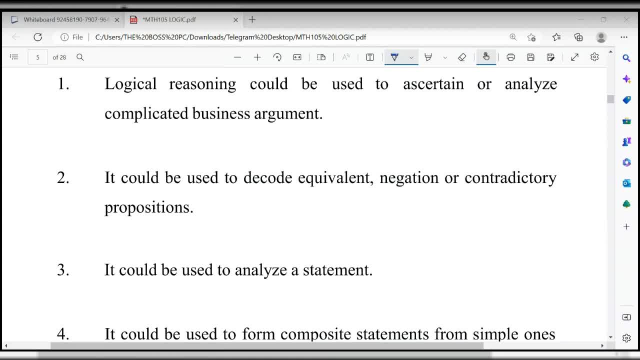 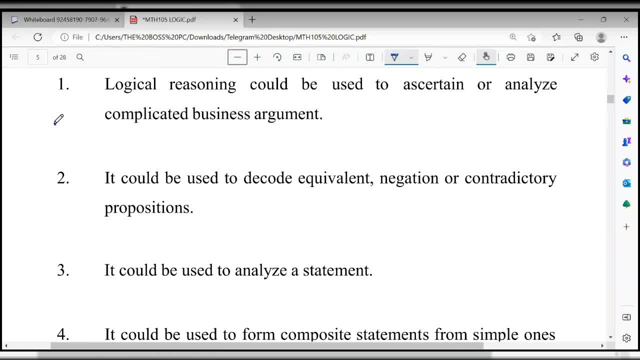 where are you joining us? from what part of the country are you? hello, okay, let me move on because of my time. okay, let me move on because of my time. okay, let me move on because of my time. let me call on jewel jewel oluwa shagon. 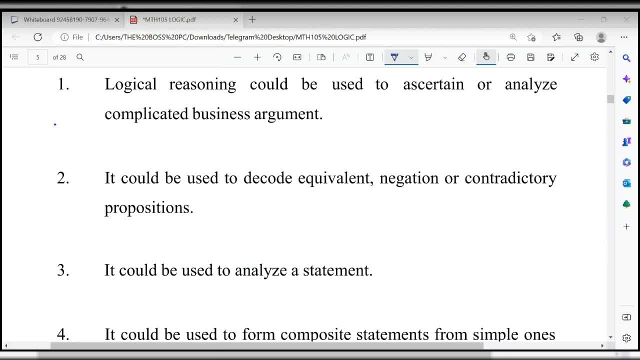 let me call on jewel jewel oluwa shagon. let me call on jewel, jewel oluwa shagon. good evening your life, good evening your life. good evening your life. can we know um? can we know um? can we know um what you think? how can you explain? 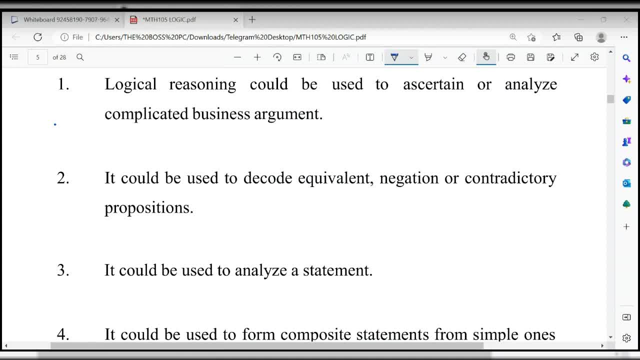 what you think. how can you explain what you think? how can you explain this first objective, this first objective, this first objective? how can you best explain it? yeah, um, can we still hear me? i'm talking? yeah, um, can we still hear me? i'm talking? yeah, um, can we still hear me? i'm talking to mr jewel oluwa shagon. 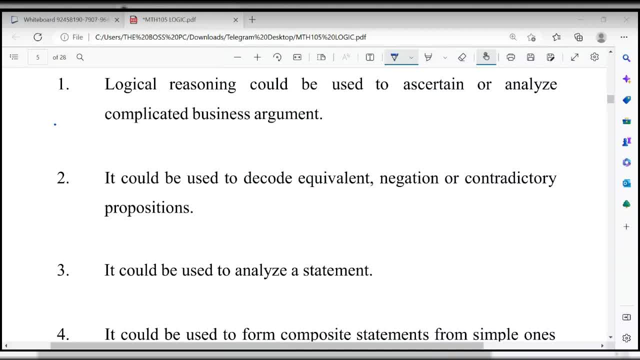 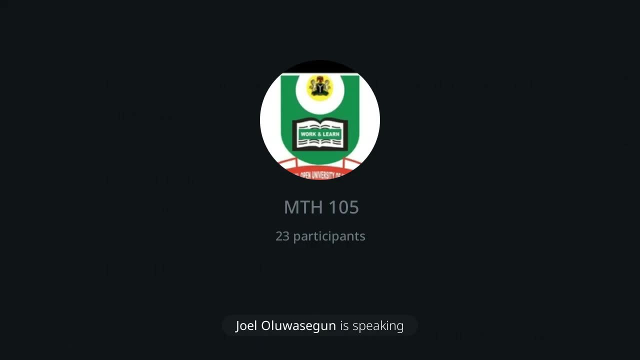 to mr jewel oluwa shagon. to mr jewel oluwa shagon: are you there, sir? are you there, sir? are you there, sir? hello sir, i'm here, but i'm not. hello sir. i'm here, but i'm not. hello sir. i'm here, but i'm not close right now. 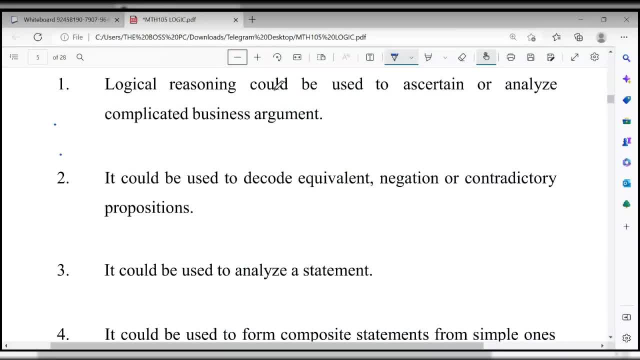 all right. so i always say a lot of all right. so i always say a lot of all right. so i always say a lot of business could be used to assert it, or business could be used to assert it, or business could be used to assert it or analyze complete. 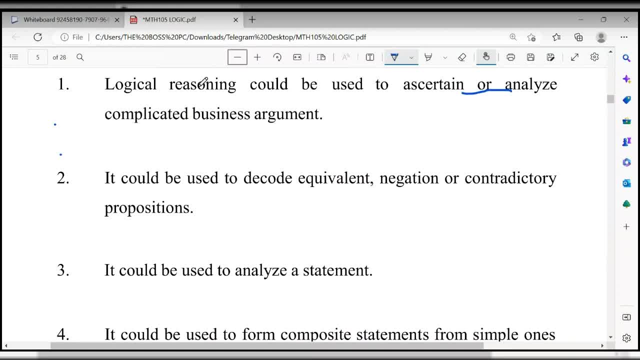 analyze complete, analyze, complete. it said um, it said um, it said um. business arguments: right. so these business arguments right. so these business arguments right. so these arguments with reasoning, since you have arguments with reasoning, since you have arguments with reasoning, since you have seen that reasoning actually helps us. 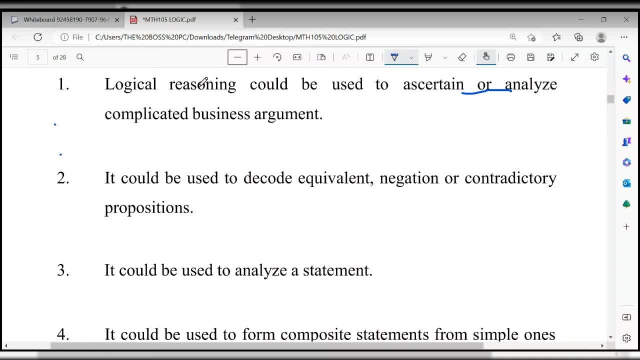 seen that reasoning actually helps us, seen that reasoning actually helps us to um to um to um. logic, rather, helps us to reason and logic, rather helps us to reason and logic, rather helps us to reason and helps us to explain, helps us to explain, helps us to explain um events with, with the knowledge of. 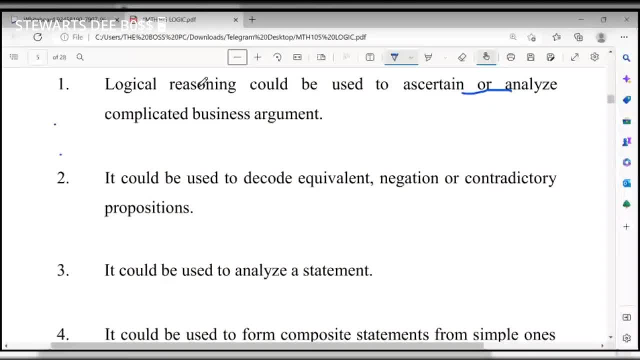 um events, with, with the knowledge of um events, with, with the knowledge of logical reasoning. you should be able to logical reasoning. you should be able to logical reasoning. you should be able to, you know, analyze. analyze has to do with what. analyze? analyze has to do with what? 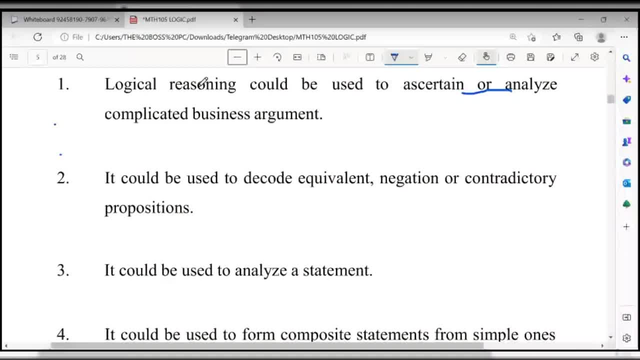 analyze. analyze has to do with what? breaking down like break it into pieces. breaking down like break it into pieces, breaking down like break it into pieces. you know business arguments that are very. you know business arguments that are very. you know business arguments that are very, very difficult to understand, that they. 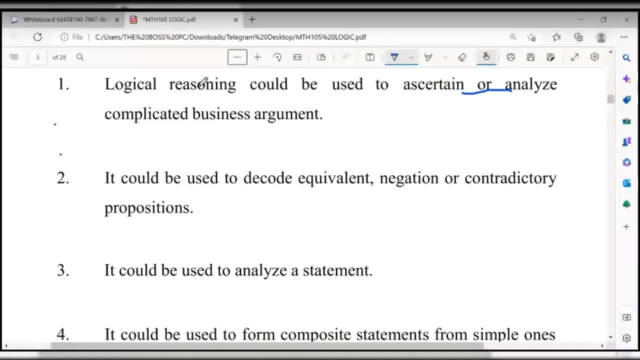 very difficult to understand that. they very difficult to understand that they call it complicated. you can be able to call it complicated. you can be able to call it complicated. you can be able to break it down in a way that you can be. break it down in a way that you can be. 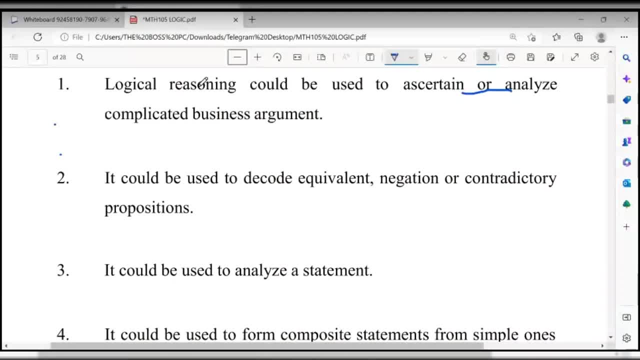 break it down in a way that you can be able to understand yourself, able to understand yourself, able to understand yourself, and then validate it, and then validate it, and then validate it. or or or. you know, you know, you know, debunk it, debunk it. debunk it because when you are where you can, 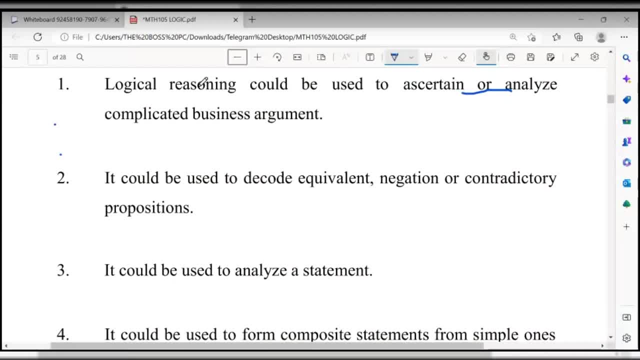 because when you are where you can, because when you are where you can reason logically, it makes it easier for reason logically, it makes it easier for reason logically, it makes it easier for you to understand things, you to understand things, you to understand things from from from a different perspective. okay, you see. 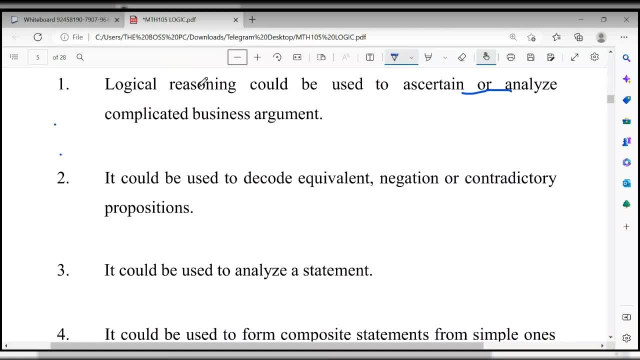 a different perspective. okay, you see a different perspective. okay, you see things from an angle that nobody else is, things from an angle that nobody else is, things from an angle that nobody else is seeing, seeing, seeing, and of course, those things that looks and of course those things that looks. 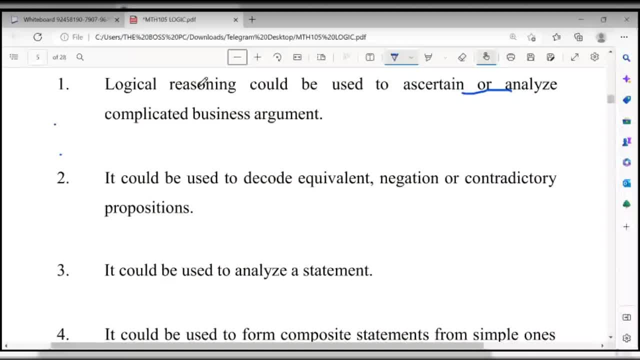 and, of course, those things that looks difficult, those things that looks difficult, those things that looks difficult, those things that looks challenging, those things that are challenging, those things that are challenging, those things that are complicated- all right, you'll be able to complicated. all right, you'll be able to. 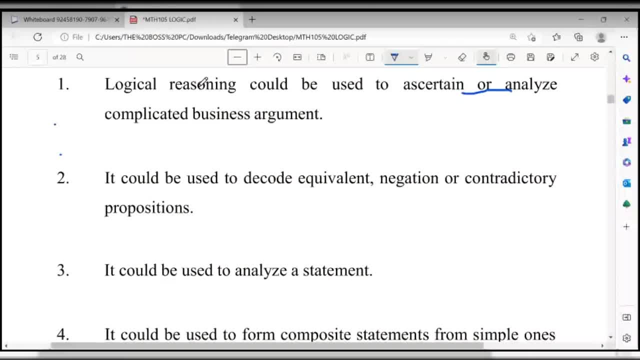 complicated. all right, you'll be able to- you know, you know, you know- go through it with ease. that is what we go through it with ease. that is what we go through it with ease. that is what we mean, mean, mean like this, like this, like this. now number two: 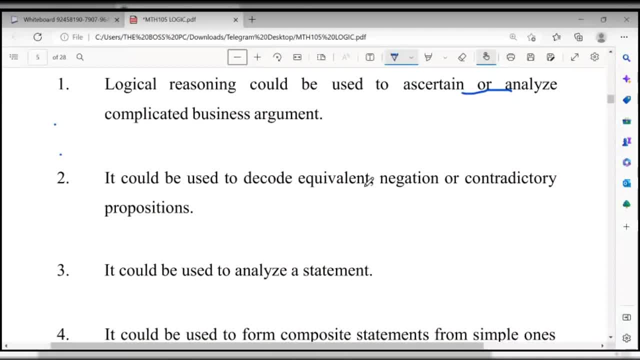 now number two. now number two. it could be used to decode equivalent. it could be used to decode equivalent. it could be used to decode equivalent negation or contradiction. negation or contradiction. negation or contradiction or contradictory preposition or contradictory preposition or contradictory preposition. so we have negation. 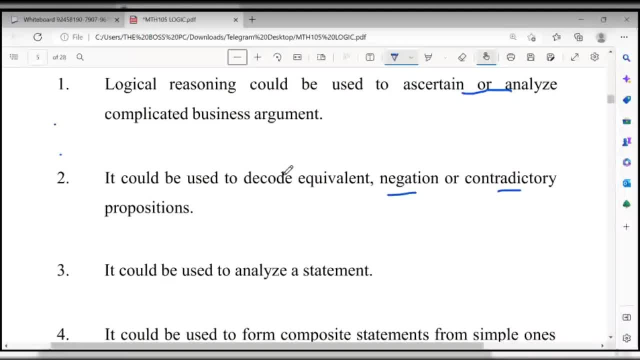 so we have negation. so we have negation. and could be used to decode equivalent. and could be used to decode equivalent. and could be used to decode equivalent. negation or contradictory preposition. negation or contradictory preposition. negation or contradictory preposition. so um 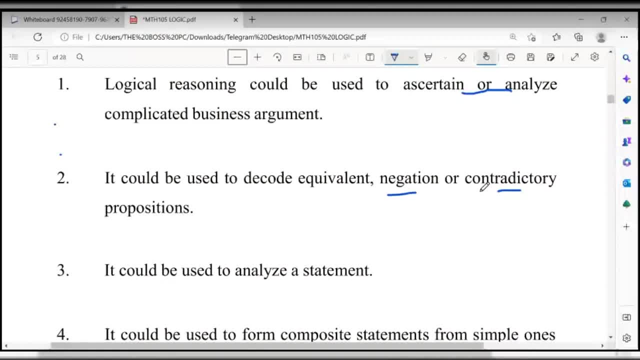 when we say, when we say, when we say negation, we get to see that as a progress negation, we get to see that as a progress negation, we get to see that as a progress as well. negation has to do with as well. negation has to do with: 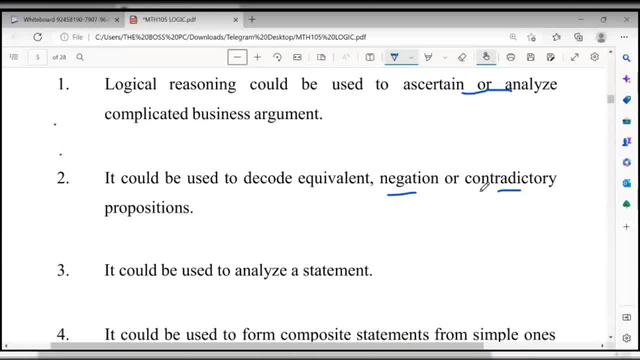 as well. negation has to do with you know, you know, you know the direct opposite of everything, the direct opposite of everything, the direct opposite of everything. i am coming, i am not coming into, i am coming, i am not coming into, i am coming, i am coming into negation, all right, um, she's beautiful. 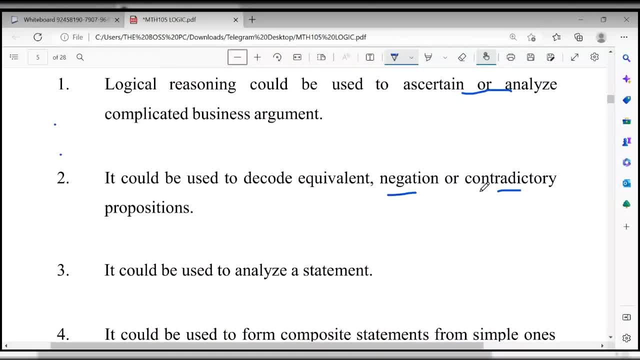 negation: all right, um, she's beautiful. negation: all right, um, she's beautiful, she's not beautiful, right? that is just she's not beautiful, right, that is just she's not beautiful, right, that is just it. and then we have it, and then we have it, and then we have um, the equivalent, equivalent, obviously. 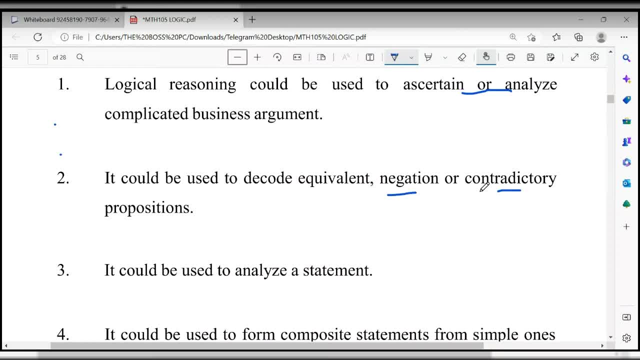 um the equivalent equivalent. obviously, um the equivalent equivalent. obviously, that is uh an equal, all right. that is uh an equal, all right, that is uh an equal, all right. and of course um we talk about and of course um we talk about and of course um we talk about contradiction, contradiction in um. 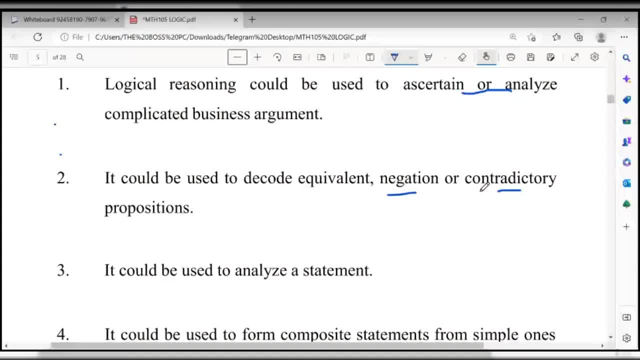 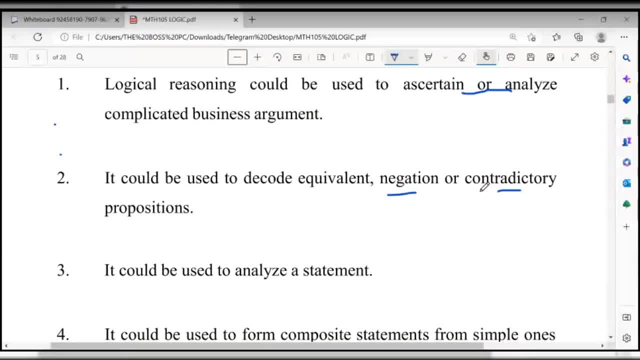 a place we get to. we talk about contradiction and tautology, contradiction and tautology, contradiction and tautology. all right, so this one is just like all right, so this one is just like all right. so this one is just like giving us a pre. 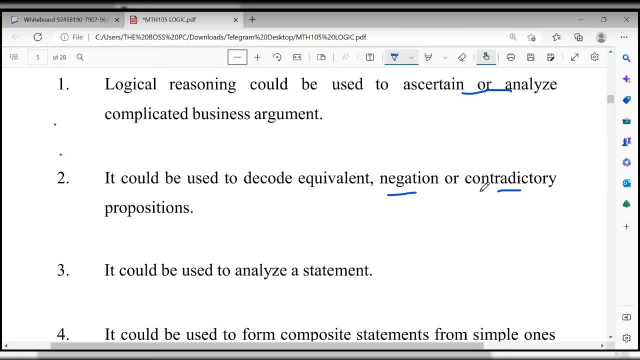 giving us a pre, giving us a pre, a preamble, a preamble, a preamble of what is, of what is, of what is yet to come, yet to come, yet to come, right, right, right, so. so, so, when we have, so, we have um, so we have um, so we have um. contradictory. 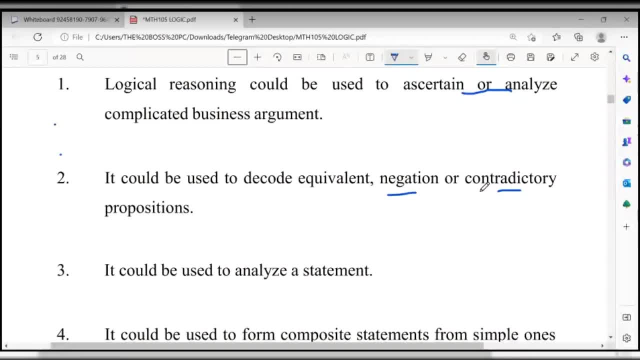 contradictory, contradictory, tautology, tautology, tautology. okay, so this is a kind of um. okay, so this is a kind of um. okay, so this is a kind of um um, you know, um, you know, um, you know prepositional logic that is forced in all. 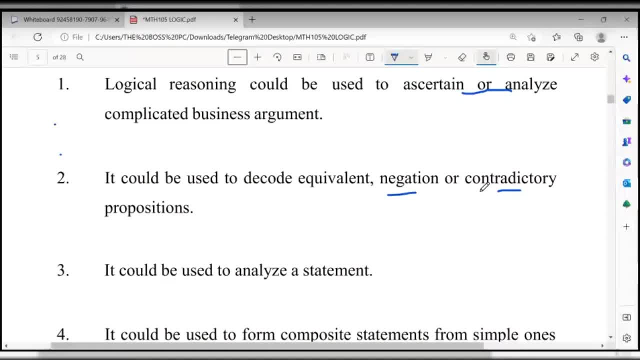 prepositional logic that is forced in all prepositional logic. that is forced in all situation, situation, situation, okay, okay, okay, that is it is false for all possible. that is, it is false for all possible. that is, it is false for all possible value of his variable. that is to say, 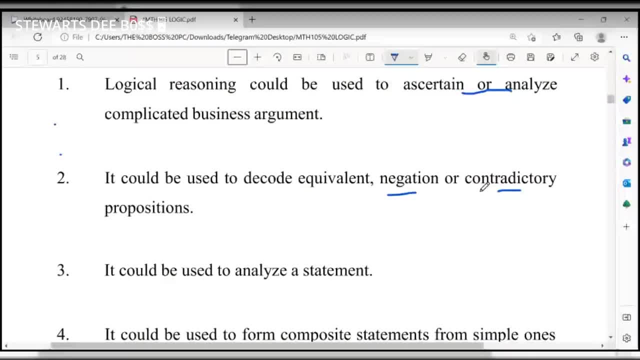 value of his variable. that is to say, value of his variable. that is to say that, that, that in every situation, it is always in every situation, it is always in every situation, it is always forced, if you see, um, how about, what kind of is i'm going to? 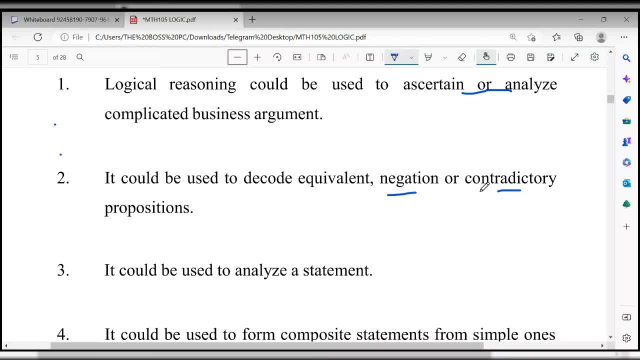 how about? what kind of is i'm going to? how about what kind of is i'm going to? give us a random example? give us a random example. give us a random example. okay, um, i'm just trying to look for an example. i'm just trying to look for an example. 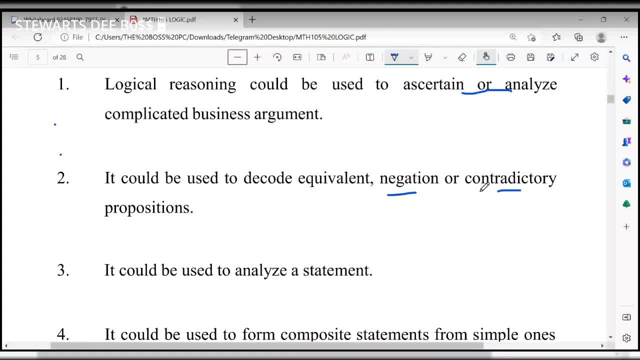 i'm just trying to look for an example that we work like something. that is that we work like something. that is that we work like something that is always forced, no matter how you look at. always forced, no matter how you look at. always forced, no matter how you look at it. 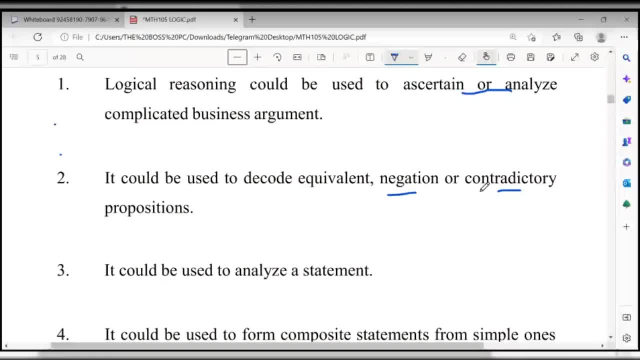 okay, um, all right now, all right now, all right now. when? what do you say? what do you say? ma saying someone is right, okay, same um people. um yeah, okay, same um people. um, yeah, okay, same um people. um yeah, yeah, that is um. that looks more like. 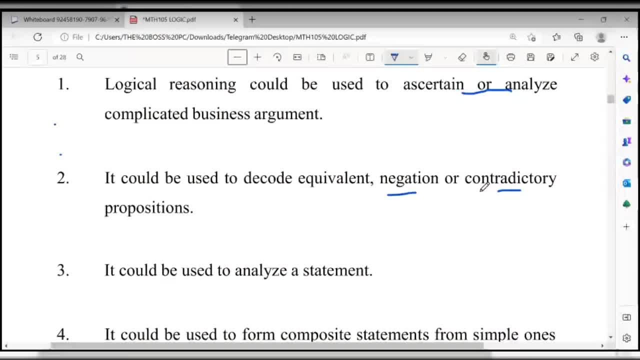 yeah, that is um that looks more like. yeah, that is um that looks more like it. but there's something i'm looking for like you know something that you look at. like you know something that you look at. like you know something that you look at it. it will not really be. it's not like. 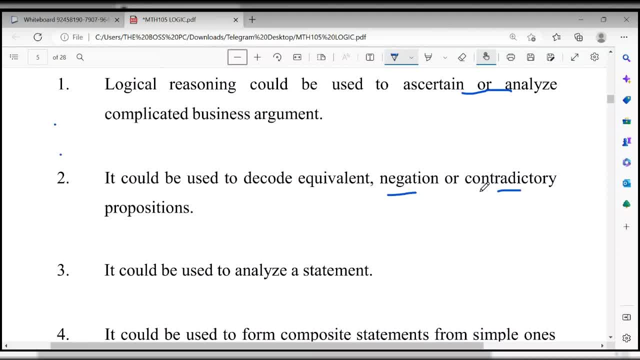 it. it will not really be. it's not like it. it will not really be. it's not like something that is easy for you to just something that is easy for you to just something that is easy for you to just write off, write off, write off. all right, it's. all right, it's all right it's. it's kind of it's something that will. it's kind of it's something that will. it's kind of it's something that will make you think a bit before you conclude. make you think a bit before you conclude. 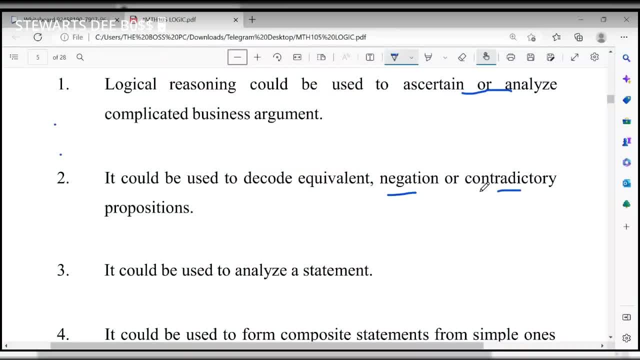 make you think a bit before you conclude that it is actually that. it is actually that it is actually um first, um first, um first. i'm going to. maybe i have to scroll down. i'm going to. maybe i have to scroll down, i'm going to. maybe i have to scroll down a bit soon. 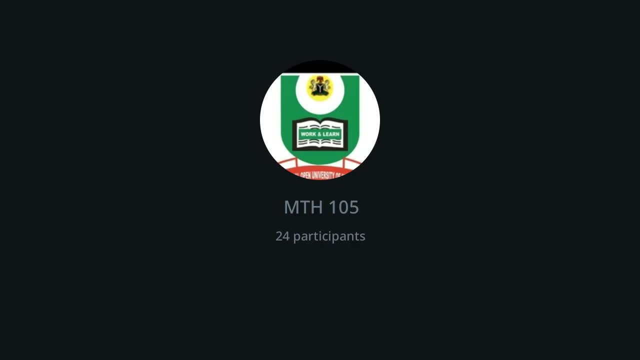 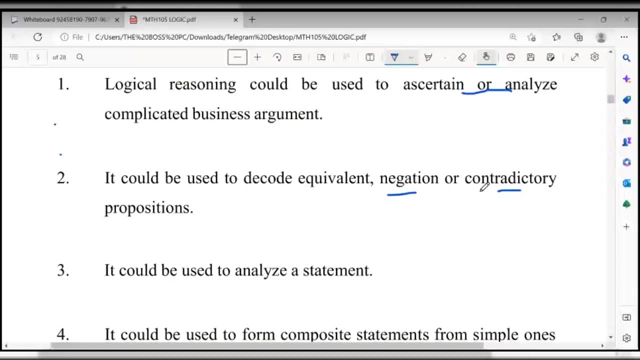 and hey, i think i've gotten the example. and hey, i think i've gotten the example. and hey, i think i've gotten the example i'm looking for, i'm looking for, i'm looking for um, um, um, now something, something, something cannot like now, cannot like now. 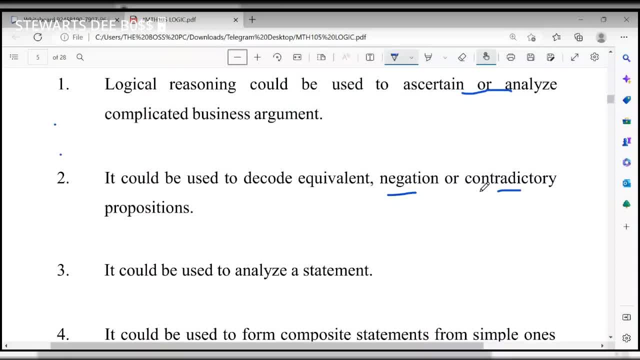 cannot like now. you cannot be a man and a woman at the. you cannot be a man and a woman at the. you cannot be a man and a woman at the same time. same time, same time, okay, okay, okay. that is what. that is what. that is, what a contract. 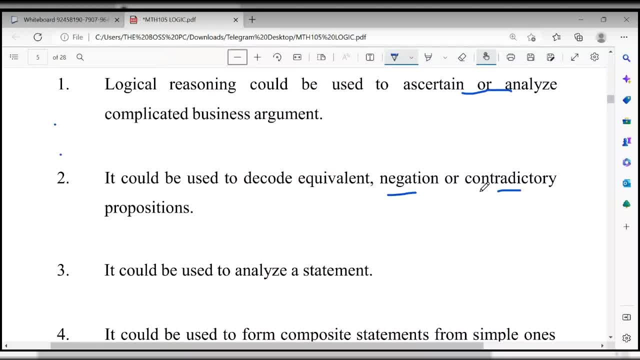 a contract, a contract. this show like to say that, okay, fine. this show like to say that, okay, fine. this show like to say that, okay fine, i'm a man, i'm a woman at the same time. i'm a man, i'm a woman at the same time. 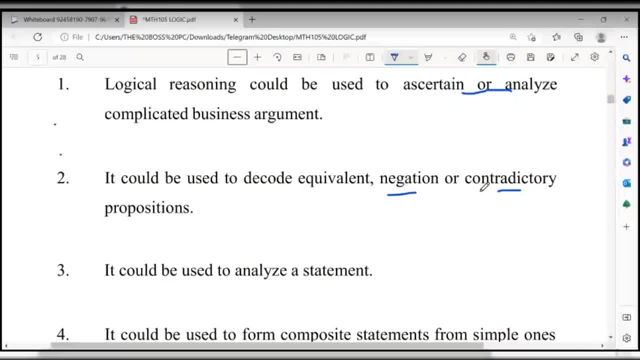 i'm a man, i'm a woman at the same time. this could be possible for one person to. this could be possible for one person to this could be possible for one person to be a man today and be a man woman. be a man today and be a man woman. 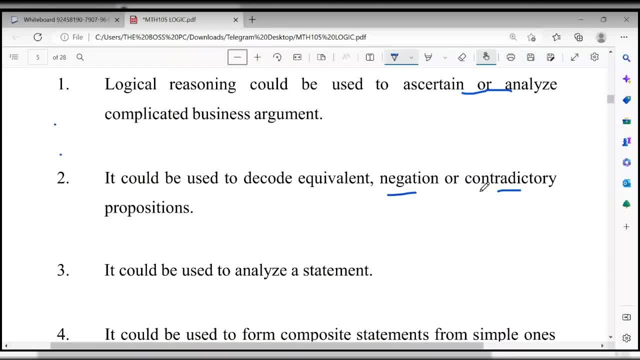 be a man today and be a man woman tomorrow. you know, tomorrow, you know, tomorrow, you know. be a woman today, be a man tomorrow. you be a woman today, be a man tomorrow. you be a woman today, be a man tomorrow. you know, know, know. just kind of thing, transgender and other. 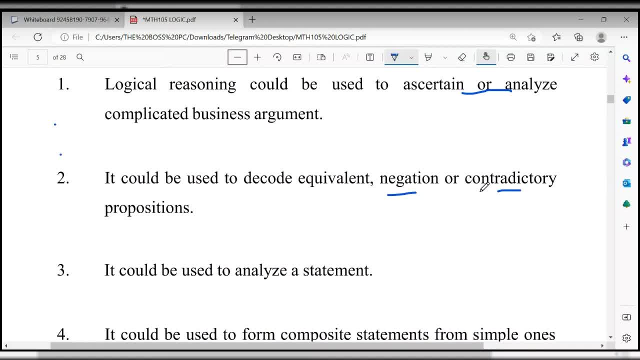 just kind of thing- transgender and other, just kind of thing, transgender and other things has not made it. things has not made it. things has not made it. it made our world a very confusing one. it made our world a very confusing one. it made our world a very confusing one. but 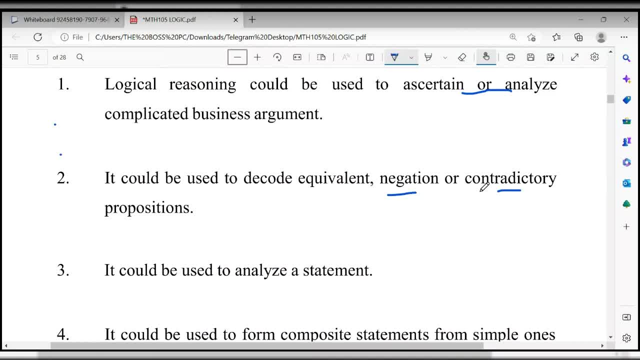 but. but it is not possible for you to be, because it is not possible for you to be, because it is not possible for you to be because there are two. there are two, there are two different realities. you're either one or different realities. you're either one or 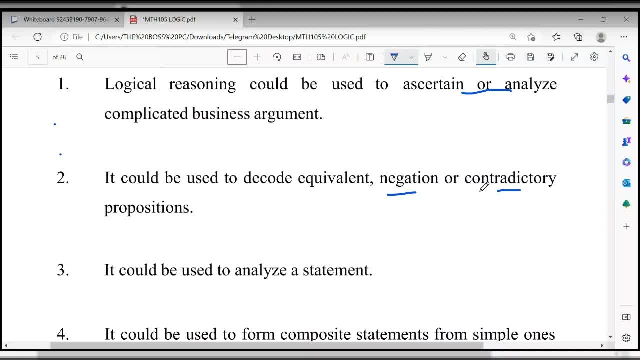 different realities. you're either one or the other, the other the other. okay, you cannot be. there cannot be light. okay, you cannot be. there cannot be light, okay, you cannot be. there cannot be light and darkness at the same time, and darkness at the same time and darkness at the same time is: either you're having light or you're. 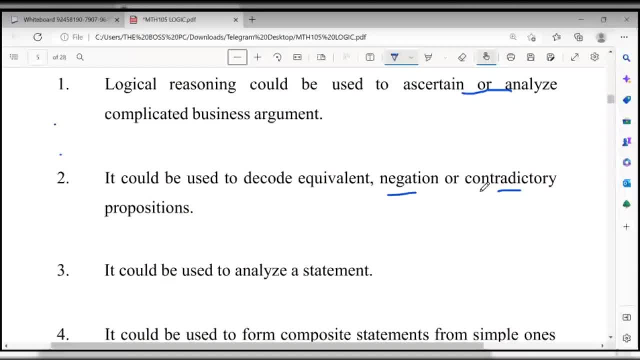 is either you're having light or you're is either you're having light or you're having darkness. so having darkness, so having darkness. so if you are not making a proposition, if you are not making a proposition, if you are not making a proposition, you're making a statement. 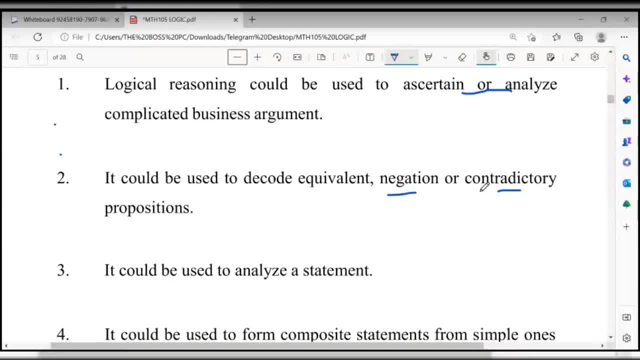 you're making a statement. you're making a statement where you are claiming to have something, where you are claiming to have something, where you are claiming to have something like these, like these, like these- two different things at the same time. two different things at the same time. 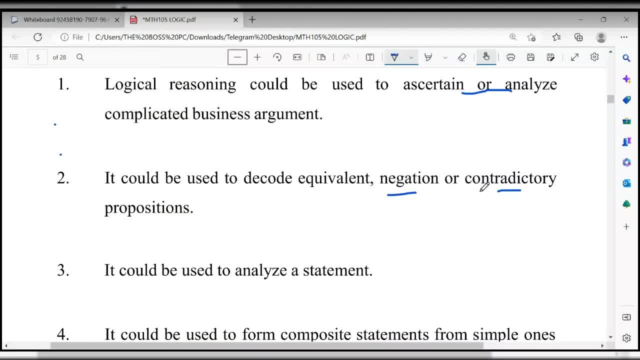 two different things at the same time. all right. so you know that that is what? all right. so you know that that is what? all right. so you know that that is what. not true, because it can never happen. not true because it can never happen. not true because it can never happen. all right, there are many things that can. 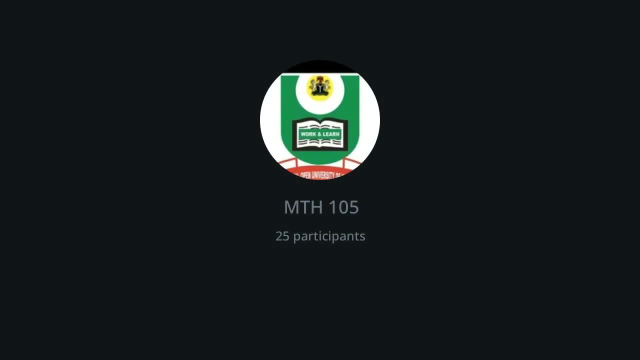 all right, there are many things that can. all right, there are many things that can coexist together, coexist together, coexist together. but this was cannot, so that is um. but this was cannot. so that is um. but this was cannot, so that is um called a deeper position, but we're not. 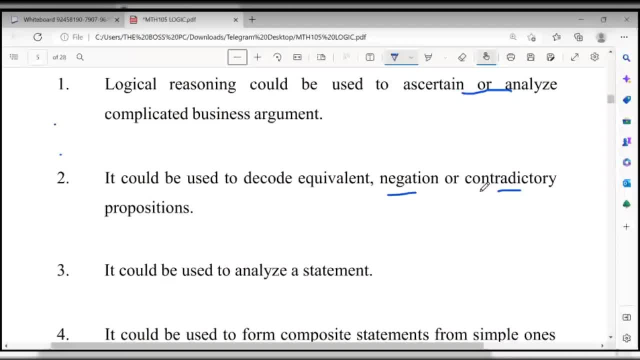 called a deeper position, but we're not called a deeper position, but we're not actually trying to explain this. what we actually trying to explain this, what we actually trying to explain this, what we need to know, is that logical reasoning need to know, is that logical reasoning? 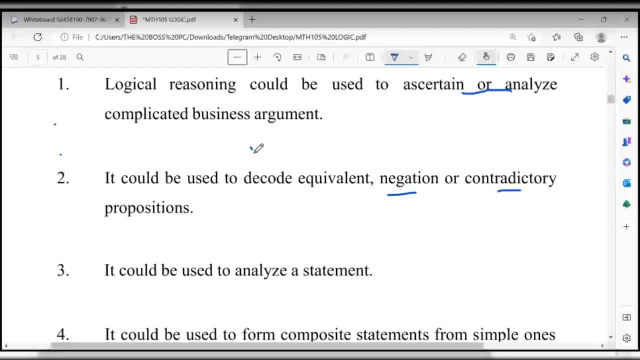 need to know is that logical reasoning can help us to decode. that means it can can help us to decode. that means it can can help us to decode. that means it can help us, to help us, to help us to know. so you can help us to understand. 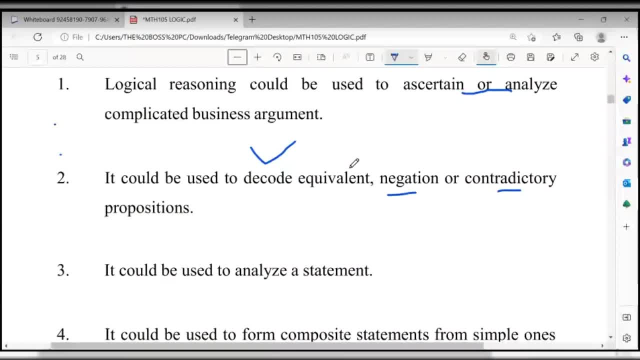 know so you can help us to understand. know so you can help us to understand all these. when we see equivalent to be all these, when we see equivalent to be all these, when we see equivalent to be able to tell this is equivalent, when we able to tell this is equivalent. when we 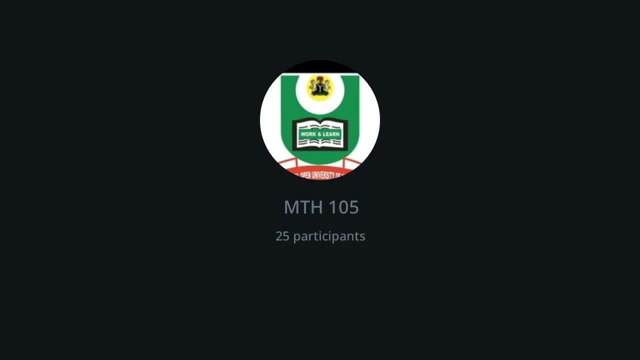 able to tell: this is equivalent. when we see negation: no, this is negation. when we see negation: no, this is negation. when we see negation: no, this is negation. when we see contradiction: we also know this is. see contradiction: we also know this is. 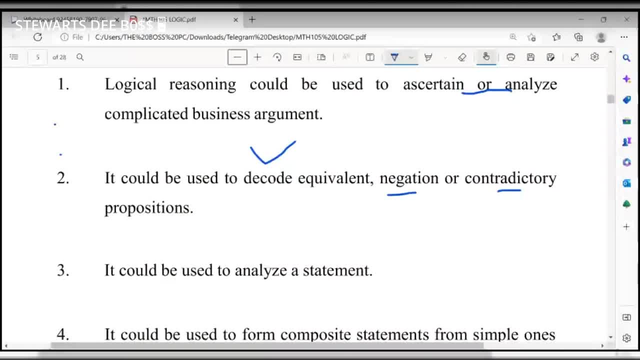 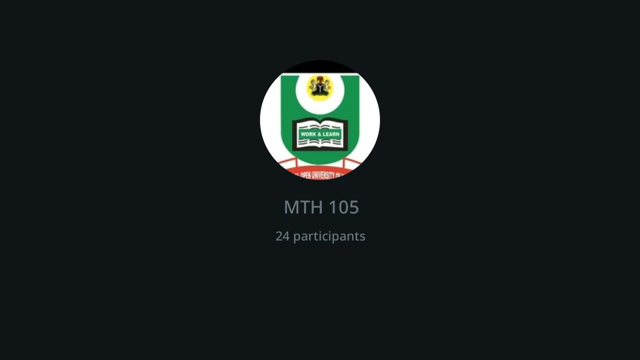 see contradiction. we also know this is somebody is talking. yeah, who could that be? somebody is talking. who could that be? hello, now. it could be used to um analyze a. now it could be used to um analyze a. now it could be used to um analyze a statement. 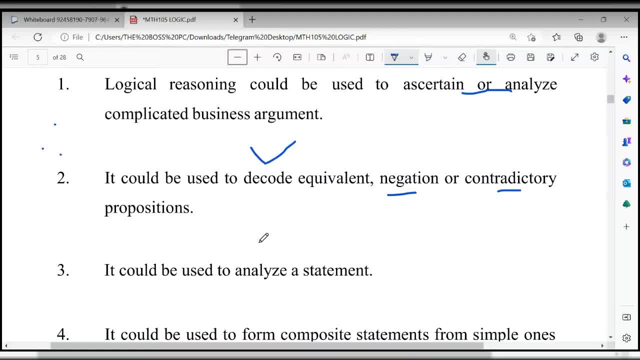 statement statement. right here they talk about analyzing on right here they talk about analyzing on right. here they talk about analyzing on business argument. you can also use this business argument. you can also use this business argument. you can also use this analysis. general statement analysis. general statement analysis. general statement: um. it could be used to form composite. 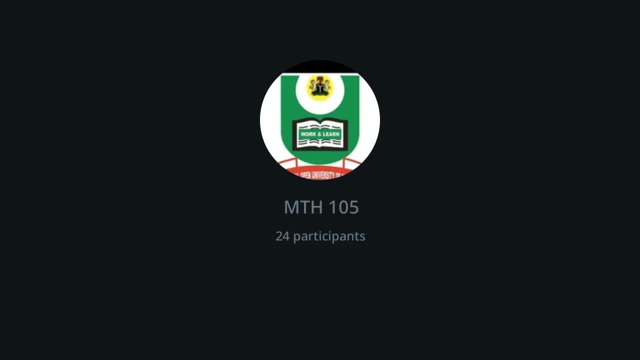 um. it could be used to form composite um. it could be used to form composite statements for simple ones using logical statements, for simple ones using logical statements. for simple ones using logical connect. you're going to do that one connect. you're going to do that one connect. you're going to do that one later. we have two simple statements like: 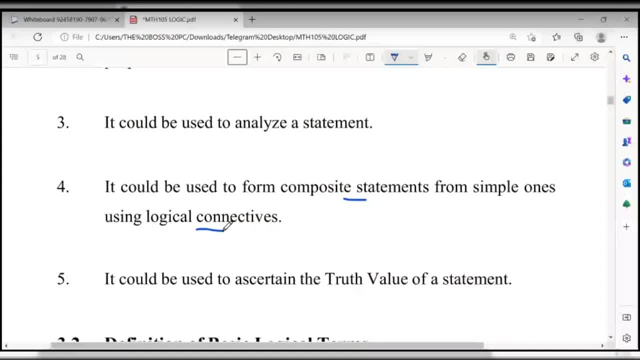 later we have two simple statements, like later we have two simple statements like: i am a boy and that is a girl. you know i am a boy and that is a girl. you know i am a boy and that is a girl, you know. just simple statement. and then you 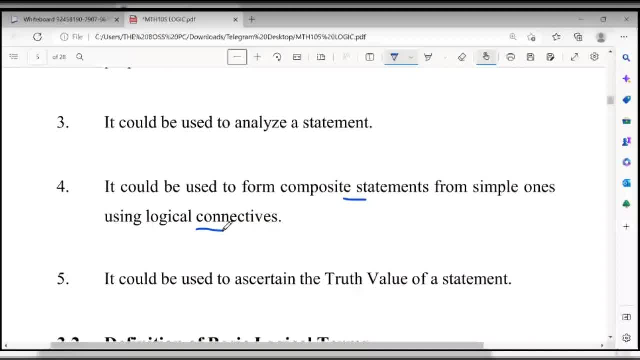 just simple statement, and then you just simple statement, and then you brought it together using. you brought brought it together using. you brought brought it together using. you brought them together using. connecting them together using. connecting them together using. connecting. connected could be and or. connected could be and or. 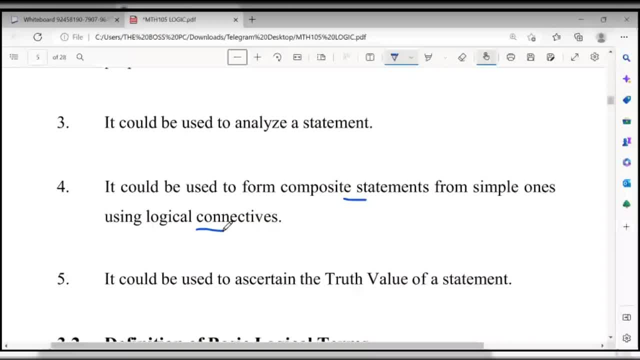 connected could be and or um you know e that is conditional. many um you know e that is conditional. many um you know e that is conditional. many types of i'm connecting we use it to types of i'm connecting. we use it to types of i'm connecting. we use it to combine two sentences. and when you do, 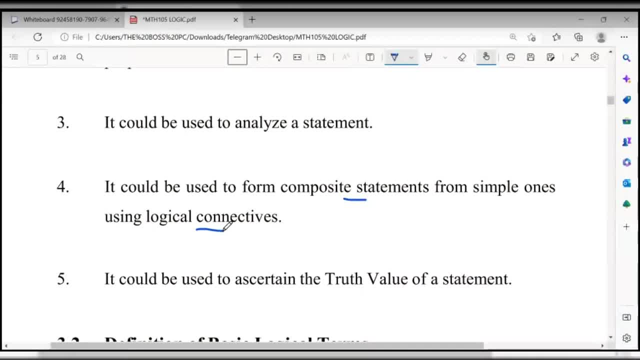 combine two sentences. and when you do combine two sentences, and when you do that, you now have a new type of sentence, that you now have a new type of sentence, that you now have a new type of sentence which you call composite statements, which you call composite statements. 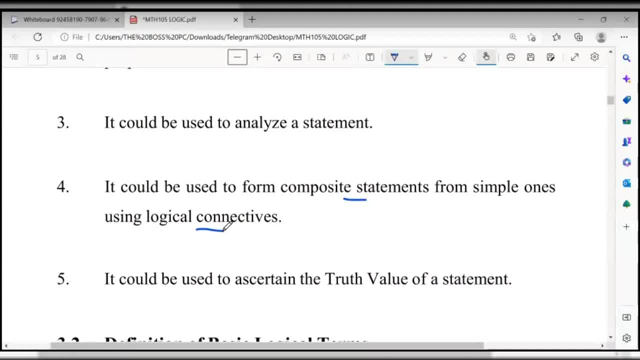 which you call composite statements. now it could be used to ascertain the. now it could be used to ascertain the. now it could be used to ascertain the true value of a statement. that one is true value of a statement, that one is true value of a statement that one is also. just. so now you can be able to tell. 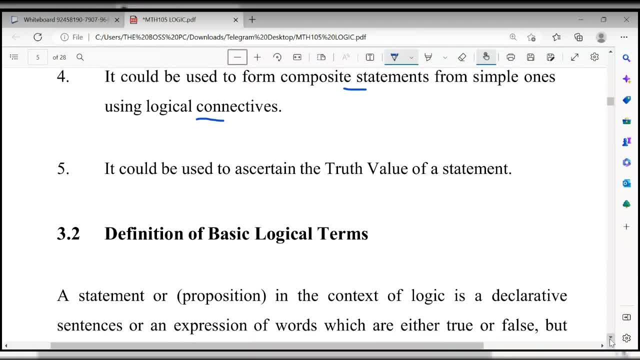 also, just so now you can be able to tell. also, just so, now you can be able to tell if something is actually true or false, if something is actually true or false, if something is actually true or false by the help of logical reasoning. by the help of logical reasoning. 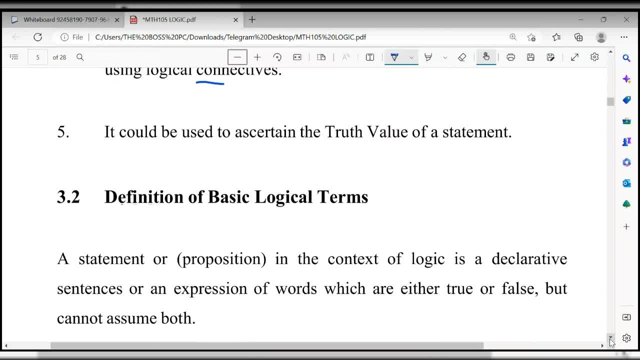 by the help of logical reasoning. now, let's look at the basic terms. okay, now let's look at the basic terms. okay, now let's look at the basic terms. okay, um, if you know basic logical terms, um, if you know basic logical terms, um, if you know basic logical terms, right, 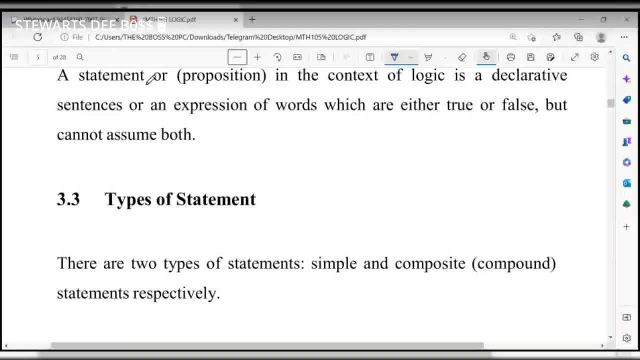 right, right now. first a statement or preposition in now. first a statement or preposition in now. first a statement or preposition in the context of logic is a declarative. the context of logic is a declarative. the context of logic is a declarative sentence. 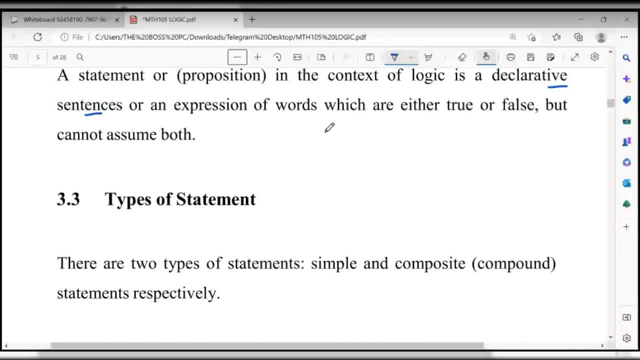 sentence sentence, a declarative sentence or an expression of a declarative sentence or an expression of a declarative sentence or an expression of words which are either true or false, words which are either true or false, words which are either true or false, but cannot be assumed. so it's like now: 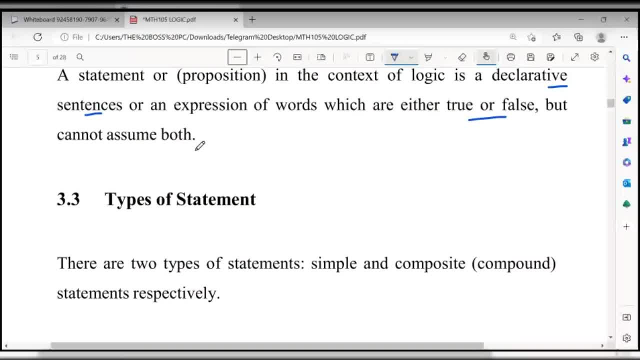 but cannot be assumed. so it's like now, but cannot be assumed. so it's like now: saying that something is both true and saying that something is both true, and saying that something is both true and false is also contradiction. false is also contradiction. false is also contradiction. okay, it can only be one. okay, that is um. 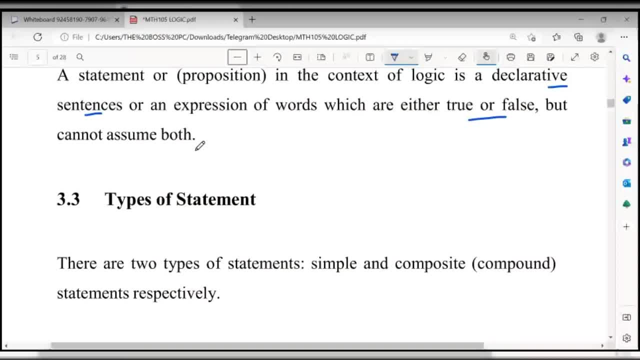 okay, it can only be one. okay, that is um. okay, it can only be one. okay, that is um. statement for you. statement for you. statement for you. all right, all right, all right. yes, just in case he asks you and when we. yes, just in case he asks you and when we. 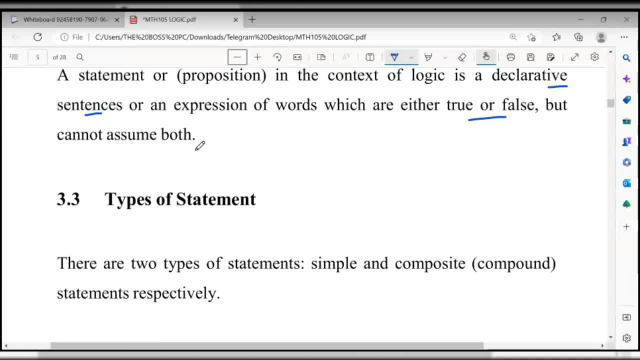 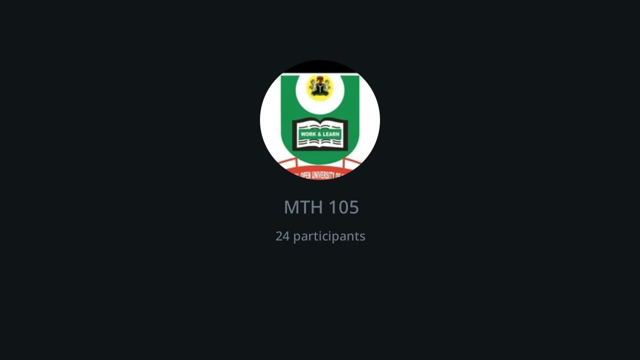 yes, just in case he asks you. and when we say declarative sentence, who can tell me say declarative sentence? who can tell me say declarative sentence? who can tell me what does it actually mean for something? what does it actually mean for something? what does it actually mean for something to be a declarative sentence? 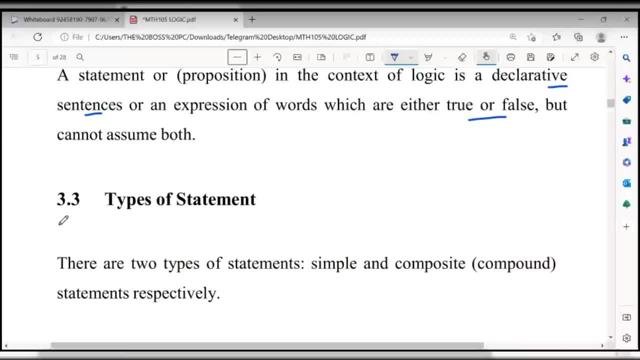 up your life. you can tell us what do you up your life. you can tell us what do you up your life. you can tell us what do you understand by the gratitude sentence? understand by the gratitude sentence. understand by the gratitude sentence. okay, mr tijani, you are alive, can you? 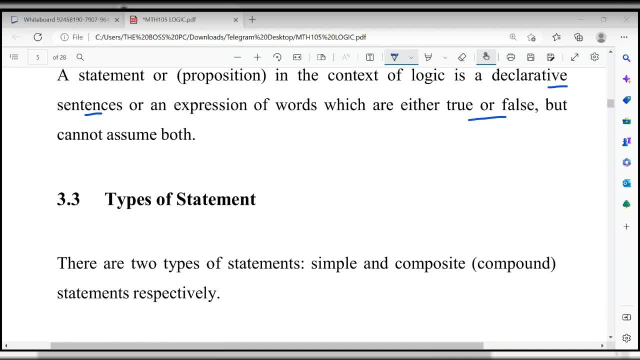 okay, mr tijani, you are alive. can you? okay, mr tijani, you are alive. can you tell us what do you understand by the? tell us what do you understand by the. tell us what do you understand by the gratitude sentence? okay, okay, okay, okay. so declarative sentences are just um. 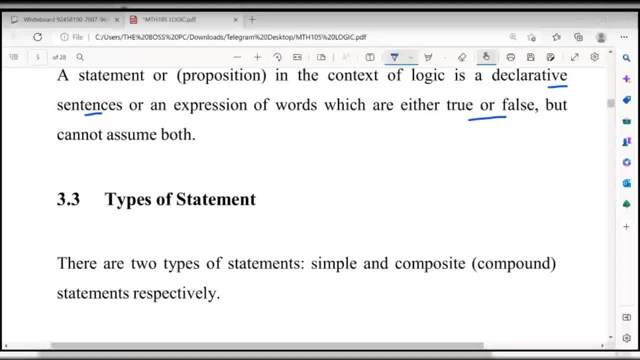 so declarative sentences are just um. so declarative sentences are just um. you know simple sentences. you know simple sentences. you know simple sentences that we use to give information, that we use to give information, that we use to give information, okay, yes, okay, yes, okay, yes. this gives information, is not. 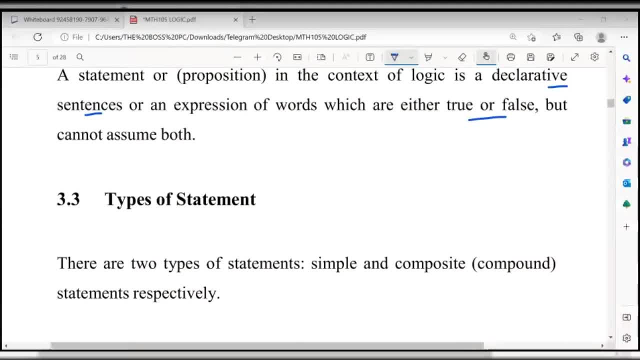 this gives information, is not. this gives information, is not asking you a question. asking you a question. asking you a question, no, no, no. so you will not really see premises um, so you will not really see premises um, so you will not really see premises um state or statements in christian form. 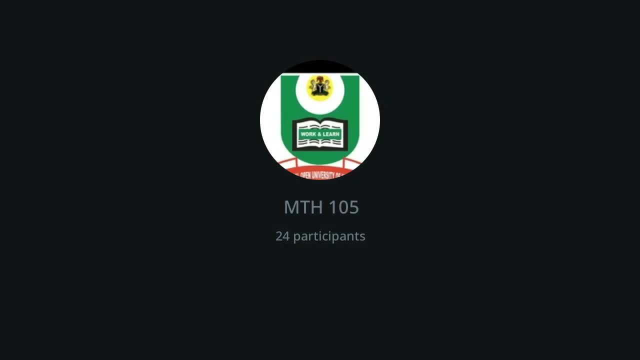 state or statements in christian form. state or statements in christian form. they are always, they are always, they are always um sharing, um sharing, um sharing with you, with you, with you information, things that you really got, information, things that you really got information, things that you really got to know. 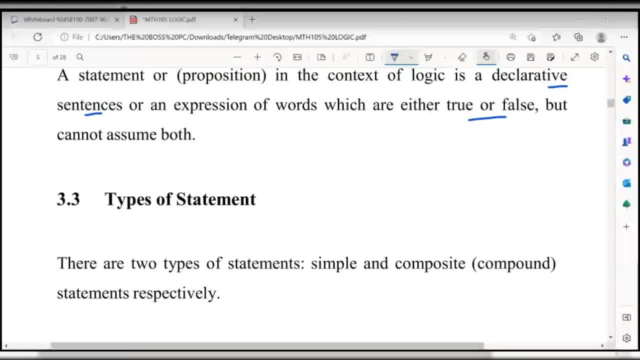 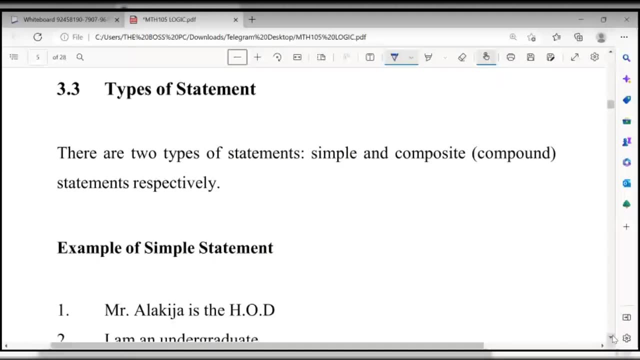 to know, to know and understand and understand and understand better, better, better now. now now types of: yes, i like cheese. that is um a simple. yes, i like cheese. that is um a simple. yes, i like cheese. that is um a simple, um statements. so we have two types of statements. we 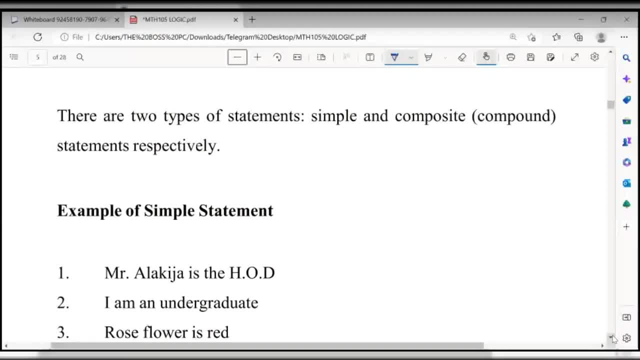 so we have two types of statements. we so we have two types of statements. we have the simple and the composite. have the simple and the composite. have the simple and the composite, composition as compound, composition as compound, composition as compound. so you can see simple, you can see examples. 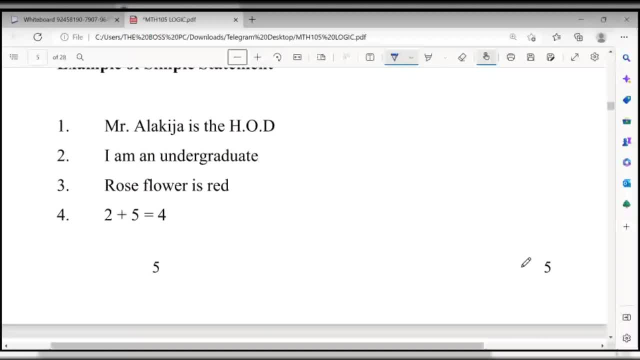 so you can see simple. you can see examples, so you can see simple. you can see examples of simple, of simple, of simple and statements. so you can give me and statements. so you can give me and statements. so you can give me additional, additional, additional, um simple statements. 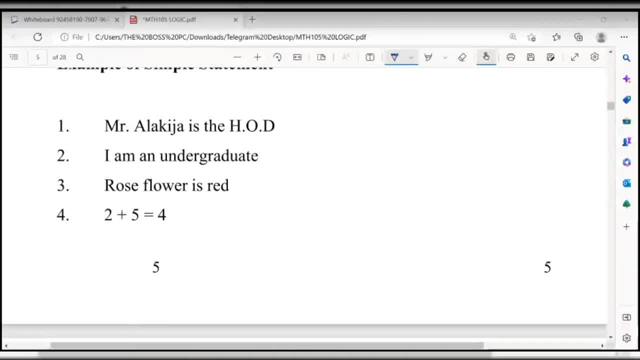 i need additional examples aside from the one. i need additional examples aside from the one. i need additional examples aside from the one because material- i live in lagos. it's an example of simple. i live in lagos. it's an example of simple. i live in lagos. it's an example of simple sentence. 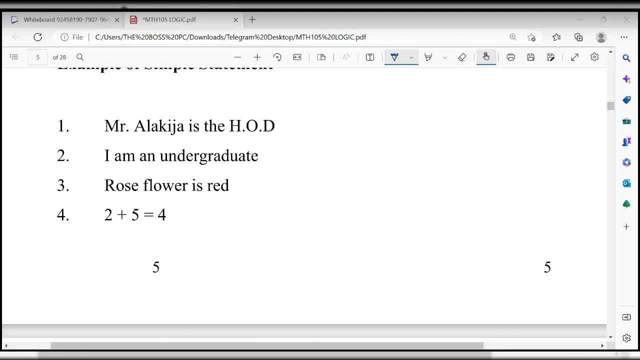 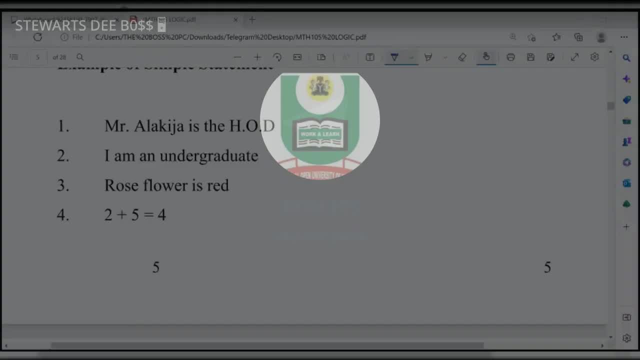 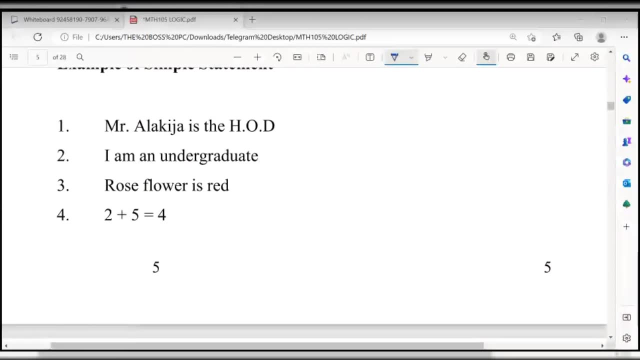 sentence, sentence, simple statement. thank you, simple statement. thank you, simple statement. thank you, thank you so much. we are not passing. we are not passing. we are not passing. my car is black. yeah, my, i am the son. yeah, my, i am the son. yeah, my, i am the son of my father. okay, yeah, that is true. 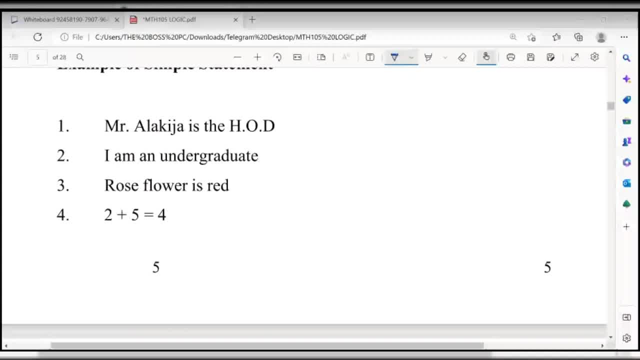 of my father. okay, yeah, that is true of my father. okay, yeah, that is true. the boss- yes, thank you so much. that is another. yes, thank you so much. that is another. yes, thank you so much. that is another one. one one. yes, one more. hello, sir, i want to ask a question. 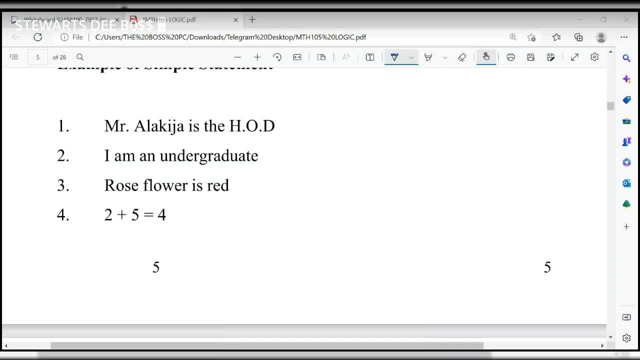 hello sir, i want to ask a question. hello, sir, i want to ask a question. okay, you are live. okay, you are live. okay, you are live. okay, um for this, uh example of statement. okay, um for this, uh example of statement. okay, um for this, uh example of statement here. 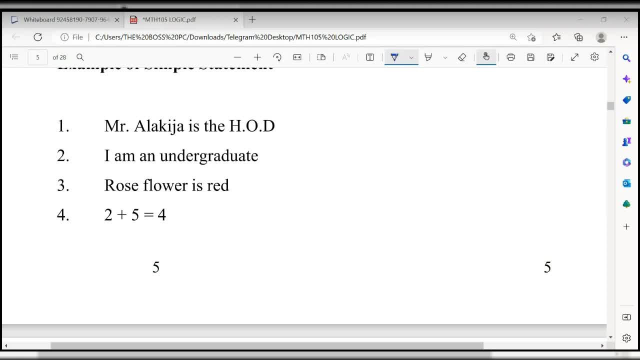 here. here, when they wrote a two plus four, two plus. when they wrote a two plus four, two plus. when they wrote a two plus four, two plus five is equals to four and akra is in five is equals to four and akra is in five is equals to four and akra is in nigerian. 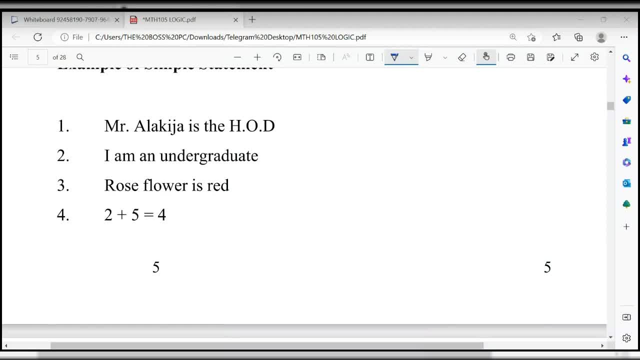 nigerian, nigerian. how that is going to be a simple, how that is going to be a simple, how that is going to be a simple statement when it is not true statement. when it is not true statement. when it is not true. um now, thank you so much for that. 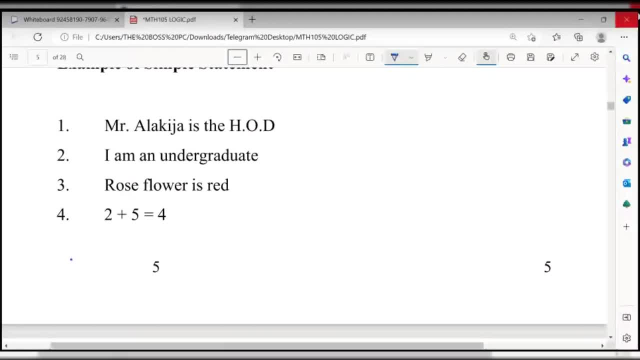 um now, thank you so much for that. um now, thank you so much for that question. question question: if you go back, if you go back to the, if you go back, if you go back to the, if you go back, if you go back to the definition of statements, 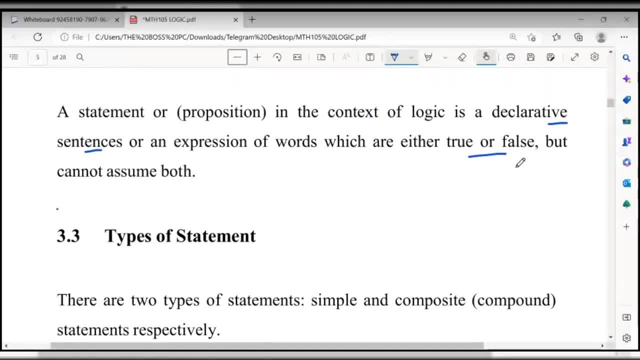 definition of statements. definition of statements: it told us that it can either be true. it told us that it can either be true. it told us that it can either be true or false, or false or false. so your statement does not always have to. so your statement does not always have to. 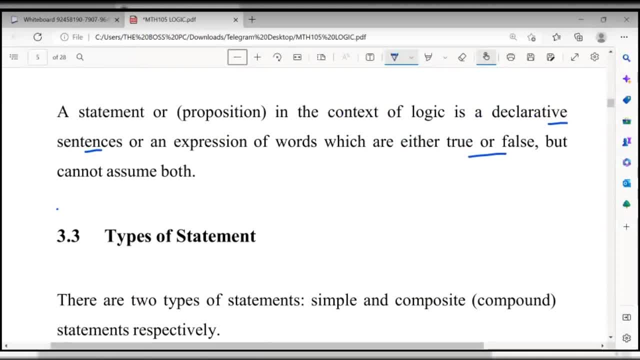 so your statement does not always have to be true. be true, be true. it can be true, can be false. it can be true, can be false. it can be true, can be false. all right, all right, all right. so there's no crime against you saying so. there's no crime against you saying. 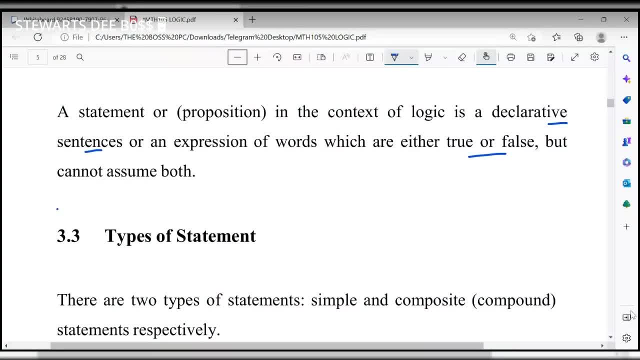 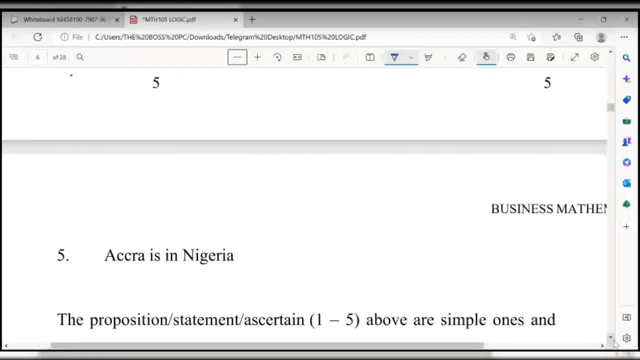 so there's no crime against you saying something that is false, something that is false, something that is false, um, it's part of logic. is that clear? is that clear? is that clear? yes, it's clear, very good, very good, very good. so, if you look at the abuse, um statement. 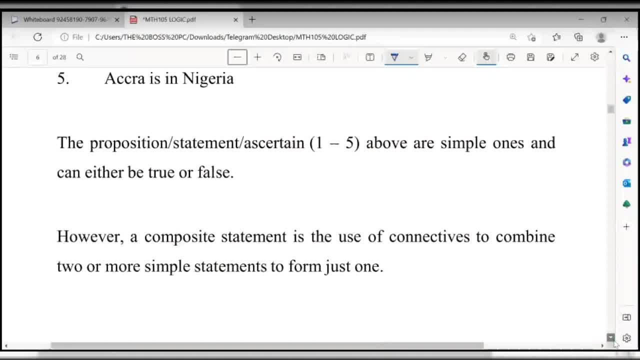 so if you look at the abuse? um statement, so if you look at the abuse? um statement, you can tell the ones that are true, you can tell the ones that are true. you can tell the ones that are true among them and the ones that are false among them and the ones that are false. 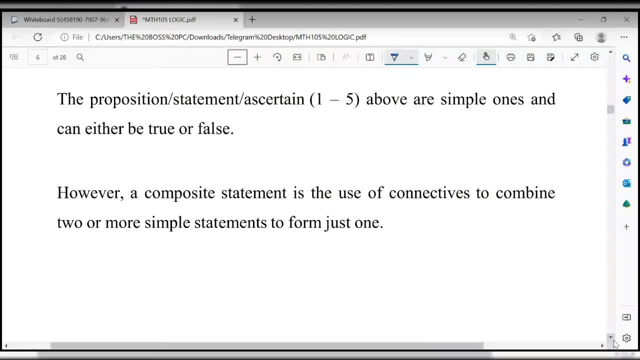 among them and the ones that are false. now a composite sentence on the other. now a composite sentence on the other. now a composite sentence on the other. one is the one, that one is the one that one is the one that has has has been combined, been combined. 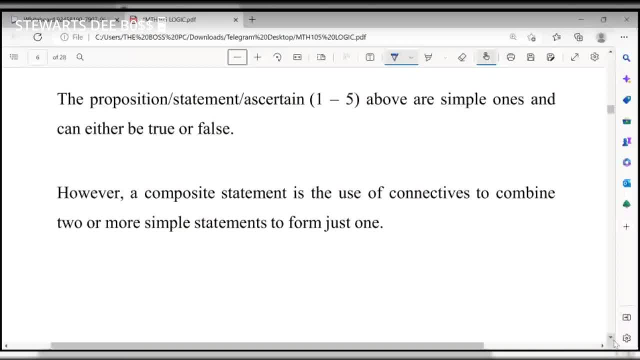 been combined. okay, where you have two stances combined. okay, where you have two stances combined. okay, where you have two stances combined by the help of connectives, by the help of connectives, by the help of connectives, so that it can become one, so that it can become one. 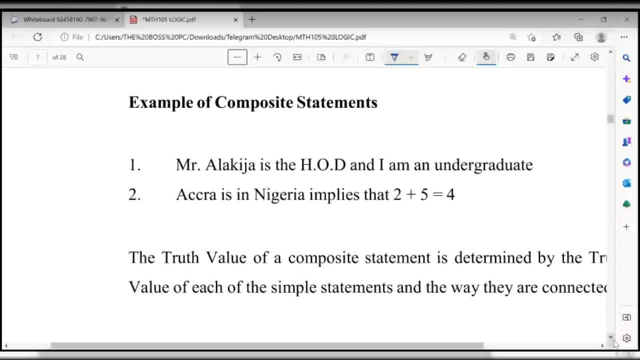 so that it can become one. so you can see examples here, so you can see examples here, so you can see examples here. so can you make your own example for me? make your own example, examples of make your own example, examples of make your own example, examples of composition. 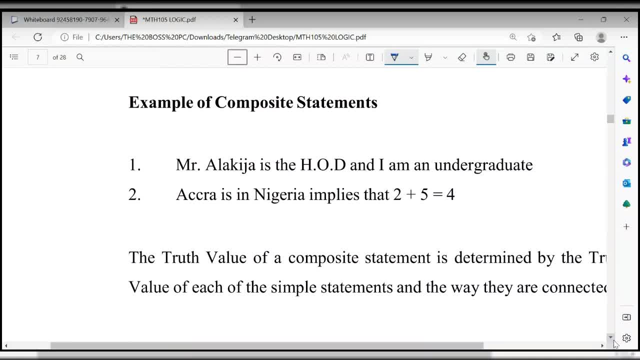 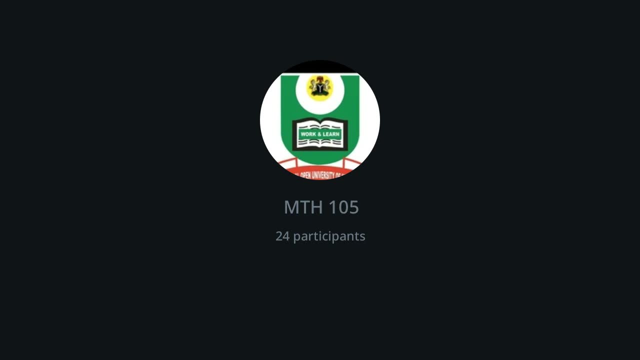 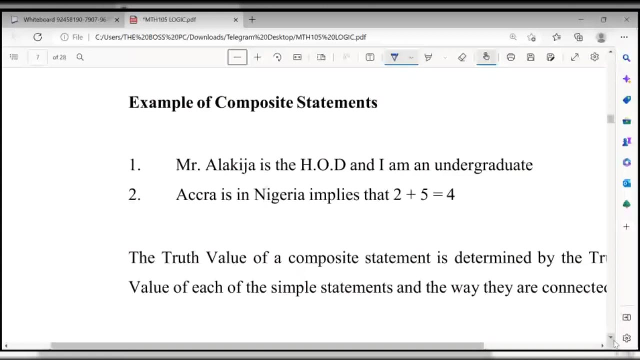 composition. composition. that's this, that's this, that's this, mr, mr, mr, mr, mr, mr. is is a businessman. he lives in lagos. is is a businessman. he lives in lagos. is is a businessman, he lives in lagos. where is the connective mr needs in lagos and 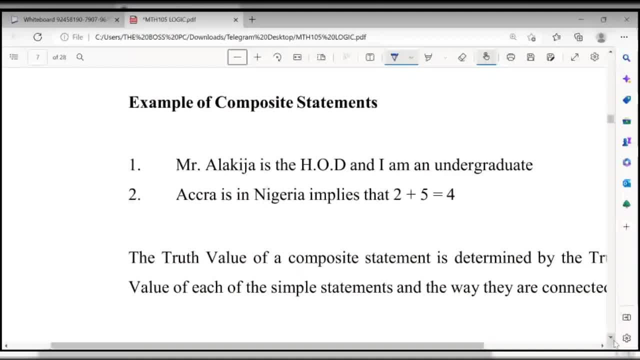 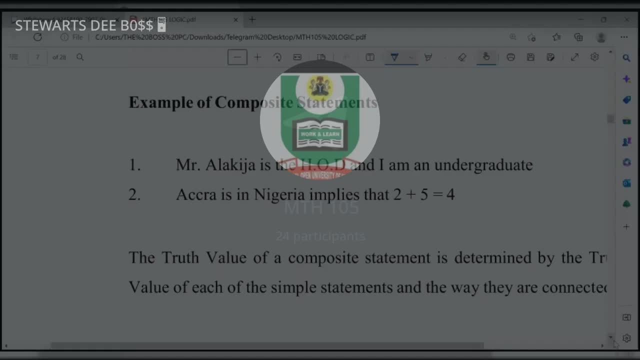 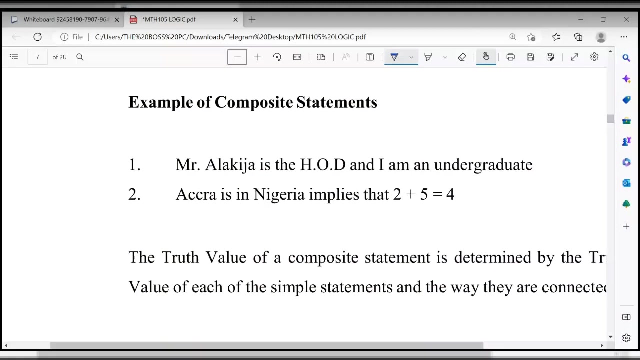 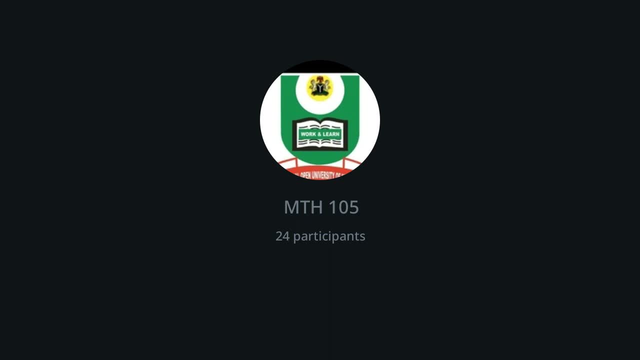 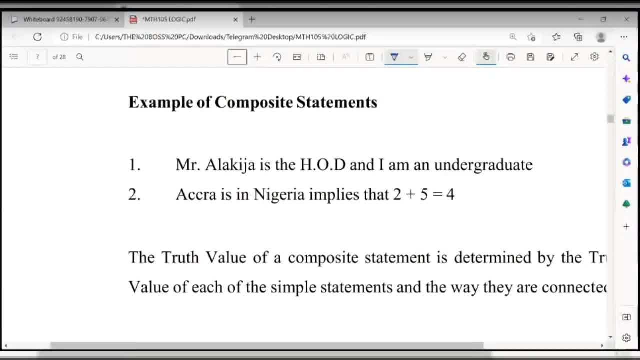 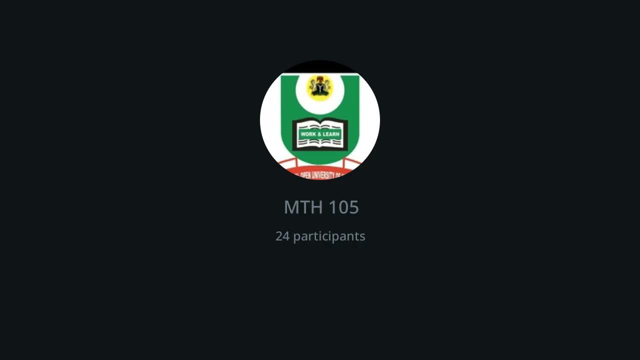 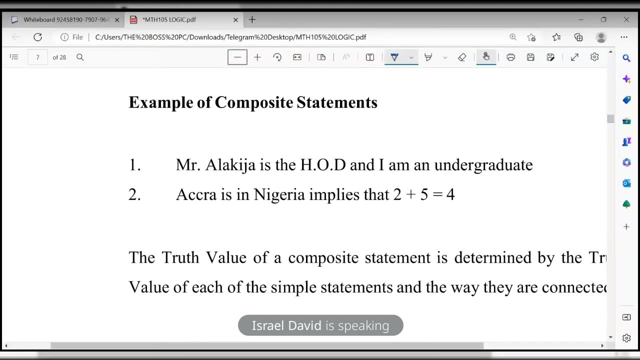 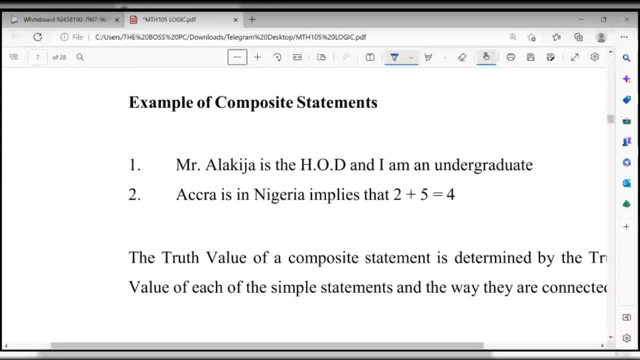 Another example, the one about it is raining and it is cold. Okay, it's raining and cold. right. Also now to present it better: it is raining and cold, not, it is raining and it is cold. Okay, One more. why are we all using and, and and and and? 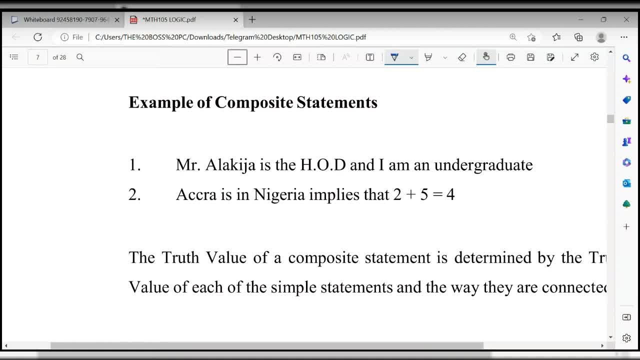 Are there other connectives you can use, aside from? and Okay, let me see, My father is a teacher about mountains. Okay, Yeah, thank you for that, You can. you can either be. you can either do business in Lagos or in Portico. 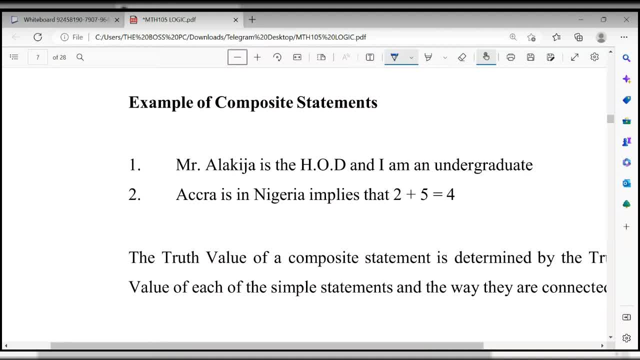 Yeah, thank you so much, Sorry. Yeah, you can use all. Yeah, thank you so much, All right, So there are so many examples out there just for us to draw out. draw out, because it's there, We know it. 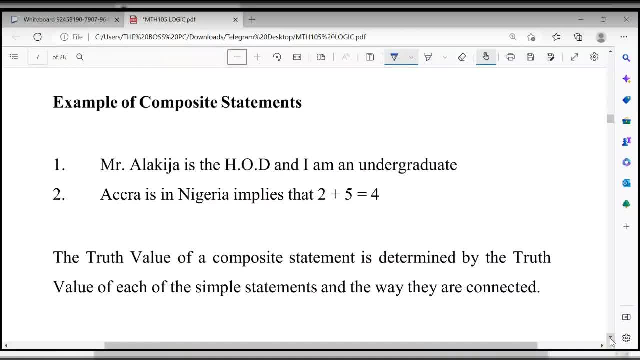 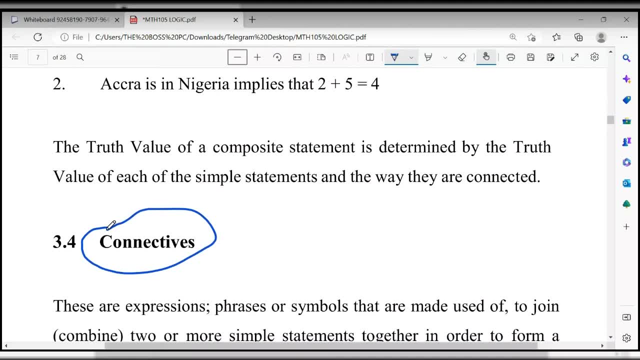 It's just for us to sit back and try to draw from the wealth of our knowledge. All right, So in this subtopic we get to be looking at all that, and this is what we're going to be stopping for tonight. So in our next class we'll continue from the different laws. 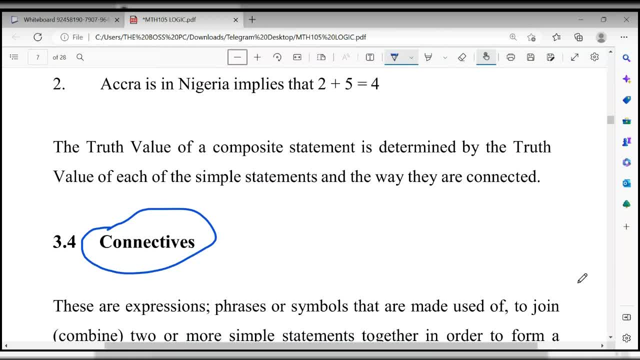 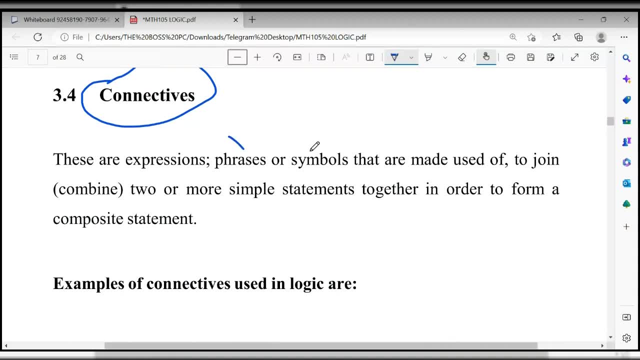 From the different laws of algebraic preposition. Okay, Now there are expressions. These are expressions. Okay, It could be phrases. It could be symbols that are used, that are made use of to join, to join or combine two or more simple statements together in composite statements. 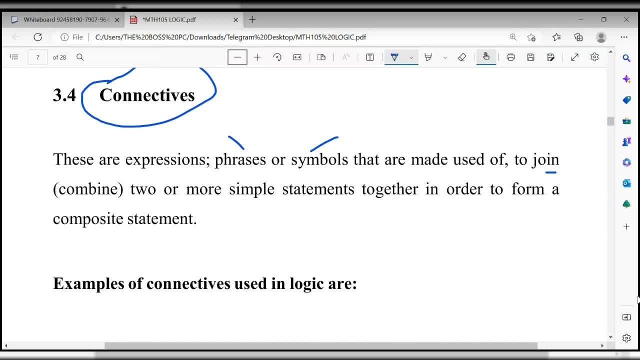 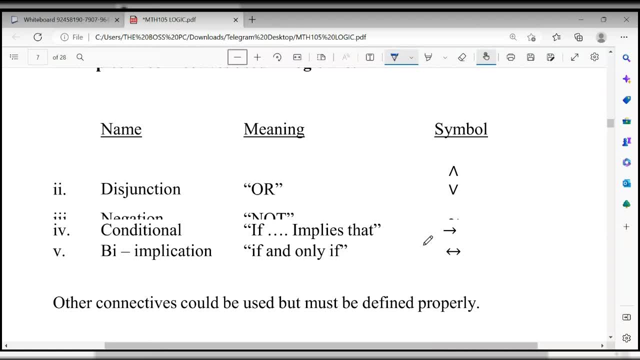 Okay, Now let's get down to business. Here are the examples, So we have them here and you can see they are symbols, Right? So we have something that I missed here. The first one is conjunction, please, So in your notes you can add it. 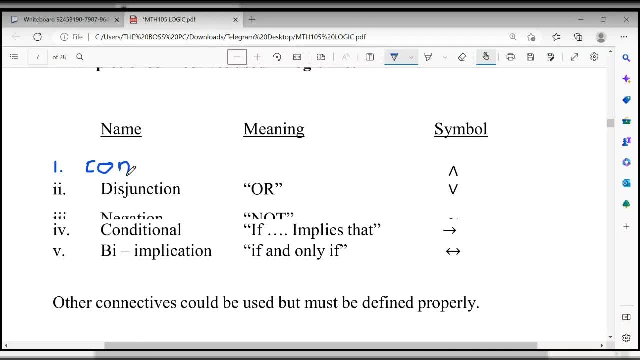 Conjunction, Conjunction, Conjunction. Now, for example, your student is an individual who is studying in the needs of her family, So I can say that there is something that I missed or I didn't mean to use is conjunction. What I want to show you is that I have such information and I will use it to heal someone. 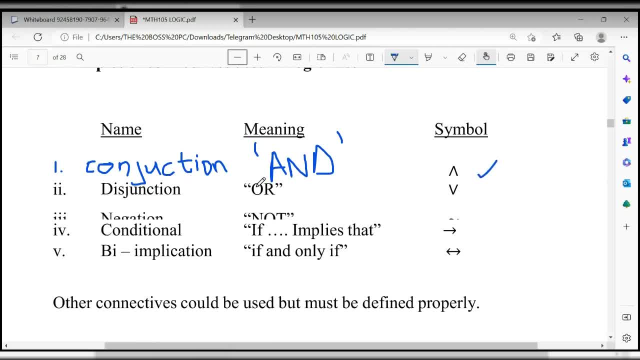 Conjunction and we have this junction. oh, and this is same as like reverse of, and this one is negation, negation me. so the symbol is different with our course material here. this is the correct correct. this is correct one. that one is error. there are plenty around your course material. that's why you need people to put you through. 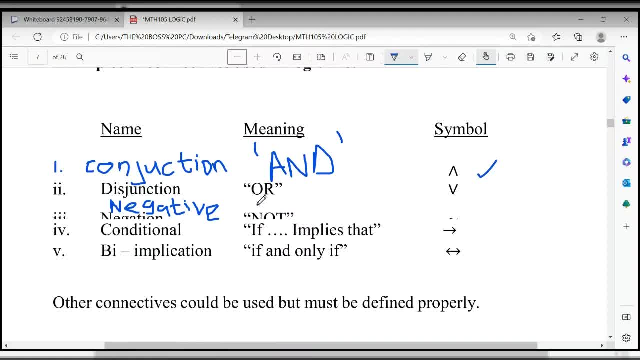 because you just go to the examination. let's see, this one is the correct one, that one is error. when i did, when i did my own mth 105, then it was even 105. so these were the symbols that when i saw- you just saw you guys- i used, i saw the mistakes there. 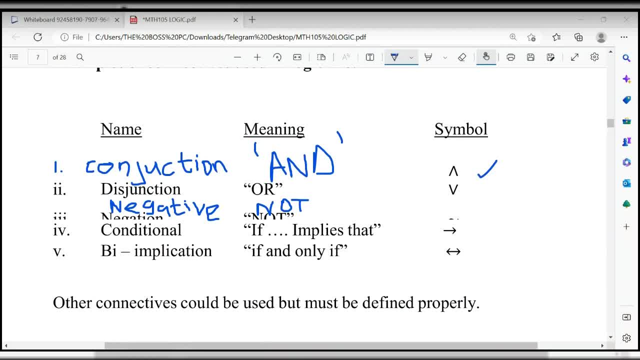 and the facilitator said: i haven't taught. teaches you, guys, that the man is my friend. he himself had to correct it for the students, so you have to correct it. that's what i'm showing you. so start using your bible to do the necessary adjustments, and that's why you need to be coming to the class. 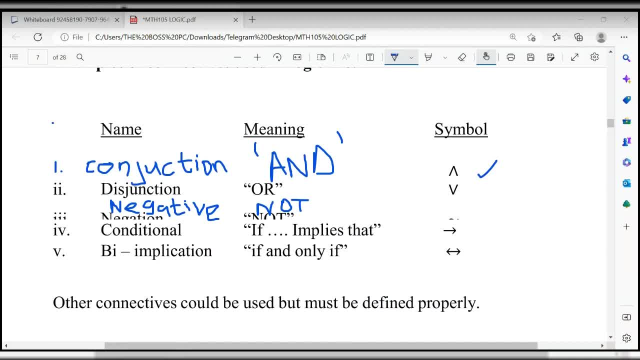 and that's why you need to be coming to the class. some of us don't know the rule of this class. you see, when you, when i start locking us out, you will know the rule i said: when you're in a noisy environment, mute your mic, mute your mic. 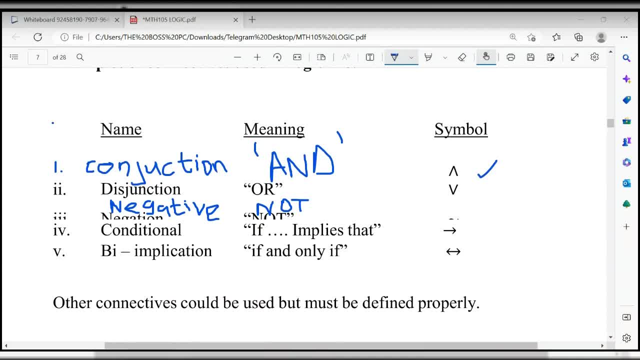 and when you are. if you are not in this environment, you can talk now what i was saying. then people will not even hear because of the whole noise. so, please, this is the right symbol. this one is something like this: please hold on, because you have different variants. 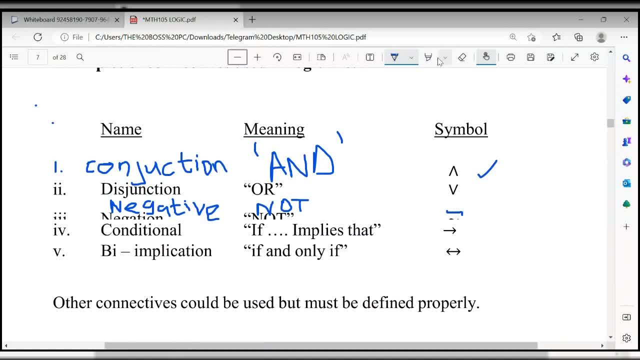 something like this, something similar to that, but what you have in your course material, if i'm not mistaken, will look like this. um right, i think your course material has something like this. oh god, my drawing is so poor. i see something wavy. um, i think this is more like it anyway. 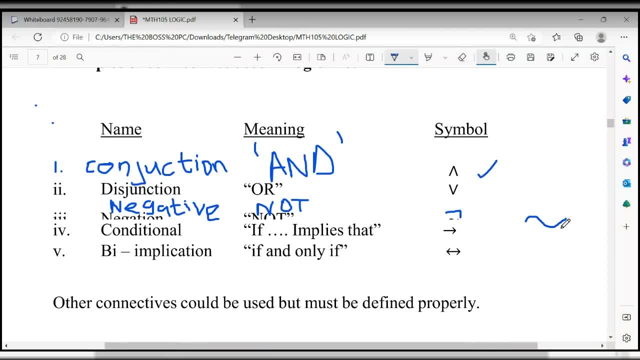 yeah, ways, so these two can actually pass something like this or like this, this symbol then for conditional, conditional, um conditionals, which implies that is a symbol- right, you can see the symbol over there. and then the last one by implication. so that's this. one is simple, two arrows facing. 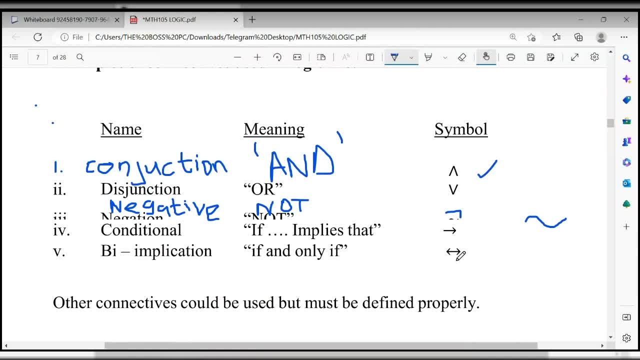 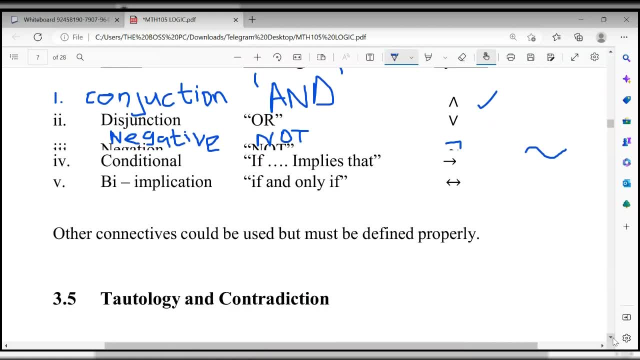 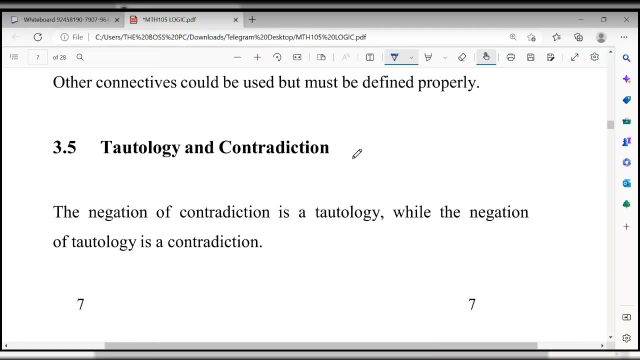 opposites. so now, having taken down the symbol, let's start explaining them all. right, so before we get that, talk about topology of contradiction. i was talking about this earlier when i said the negation on tradition is technology. why the negation of the largest contradiction? okay, fine, but before we get to, 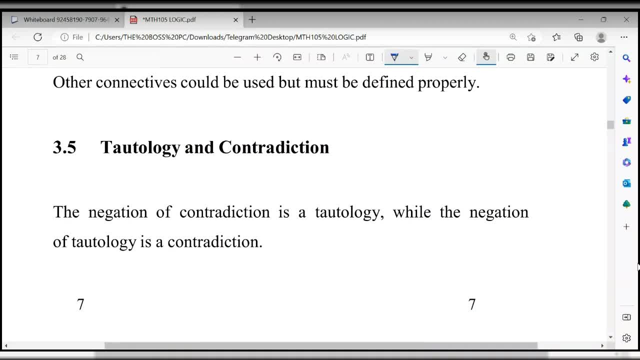 like this: uh, okay, so before we talk about it, um, remember that i told us something about contradiction. now i want to explain it again. okay, so when we see tautology, we use this a lot when we have compound statements, and it's important that you understand it, because i'm talking about connectives. now i know, once you have. 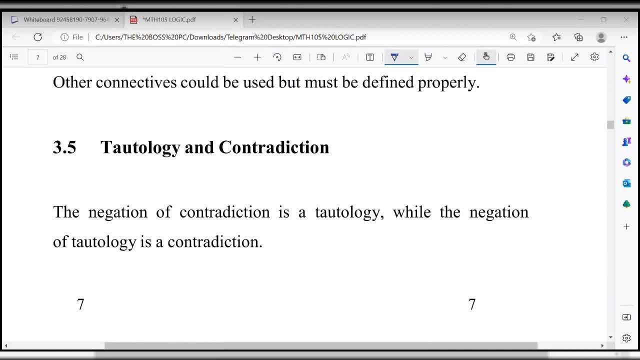 connectives most of all. if I omit those, you don't do anything other than disturb my class and make noise. so I don't know, like most of you, have any reputation of making noise in my classes. so I won't be omitting you guys in my class again, because anytime I omit you just to make noise, 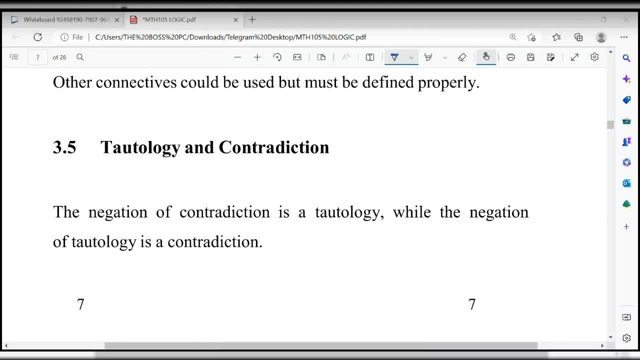 now um, but talking about this tautological condition here, because we have moved to composite statements, because anytime you see connectives, you know the next thing is coming is um compound statement, because there's no way you can use connectives and two simple sentences will not. 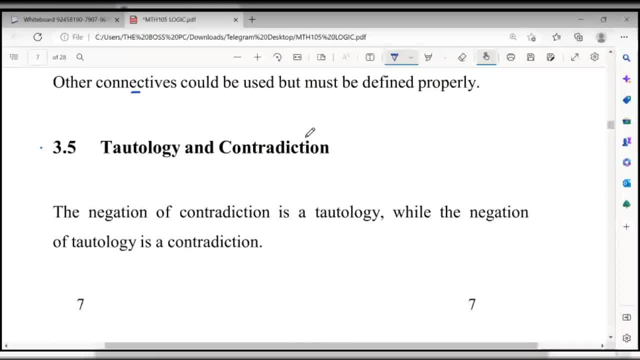 come together. when two simple sentences come together, you now have a compound statement. so when you have compound statements, you are bound to end up having um any of these. it's not in every case. you have ontology or contradiction. there are some compound statements that are true, or 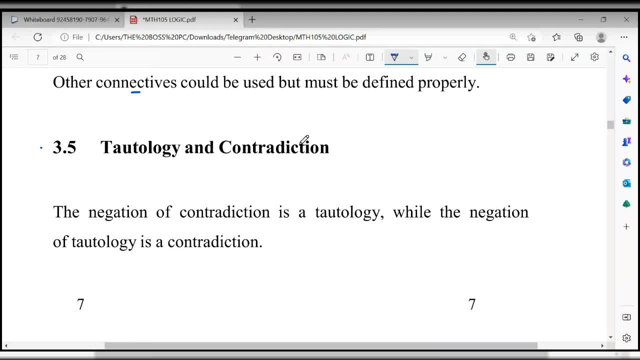 false depending on the situation that we find ourselves. there are some cases whereby it to be true, some cases it will be forced, all right, but when we have, you know, a composite sentence, that is always true, always true. okay, we call it ontology what I say, always true. we call it tautology. yes, 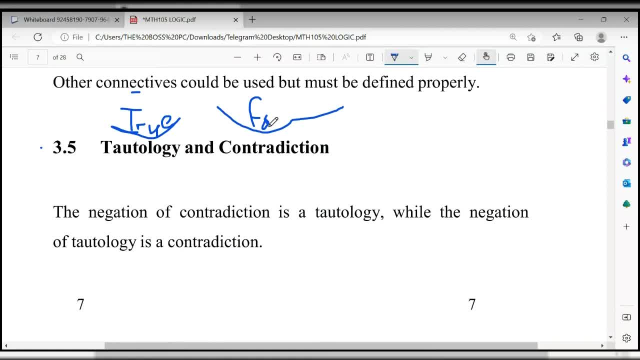 it is always true. we call it one is always false. you call it contradiction. that means tautology, and contradiction means true and false. yes, for composite means always. this, tautology is always true. a composite statement- that is always true. tautology means a composite statement that is always false. 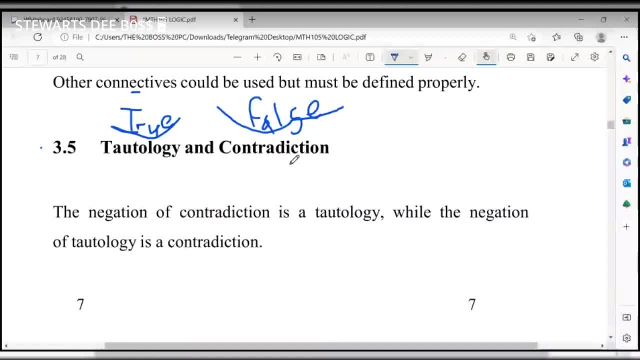 okay, so we have, um, quite a lot of examples. i'll give us exercises to determine. you know, tell me which one is tautology and which one is contradiction. what is tautology and which one is contradiction? let's go to the next one. so this one is a qualitative one that is called uh. 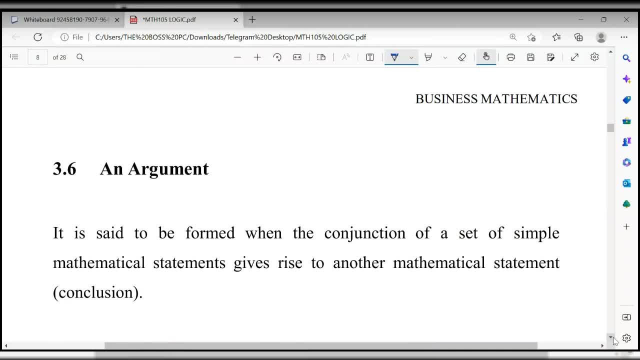 tautology, and this is a classic one that is called a tautology- of the definition of tautology. okay, okay, simple statement, okay, simple mathematical statement. you know being joined, conjunction being joined together, and that that you know together leads to the forming of another statement. 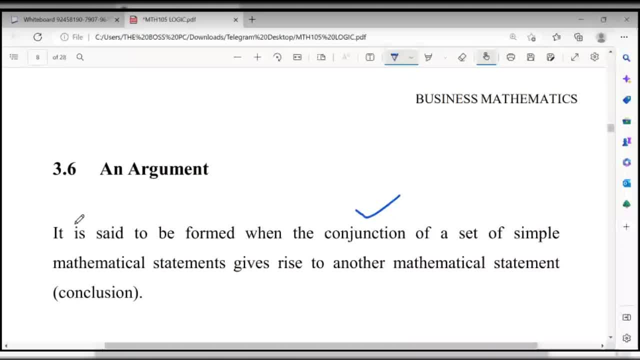 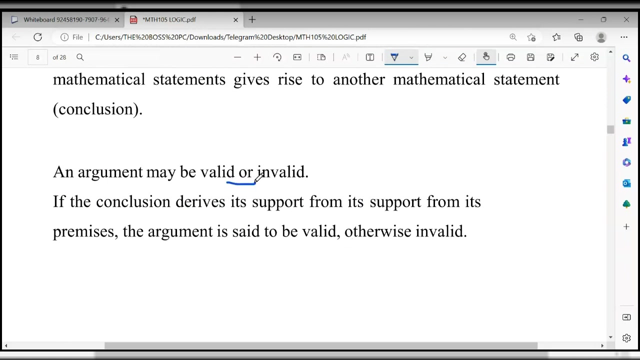 uh, which is known as a conclusion. we know that like argument has been formed, so in our arguments we have what we call um premises and the conclusion. the premise is the um- um statement that leads to another statement which we often have as conclusion, and it may be valid or invalid. now there's a question that asked us earlier. you know what. 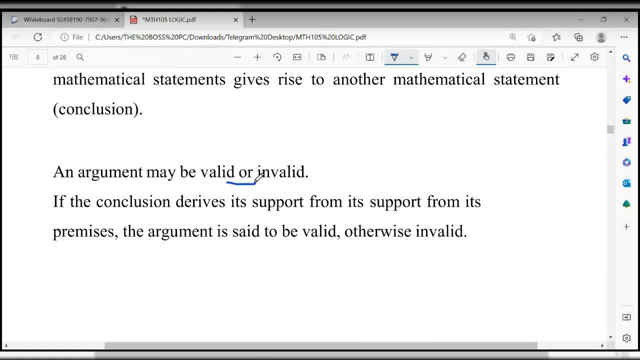 type of argument do we have? did anybody attempt to answer it here? was there anybody here that attempted that question come again um two types of arguments that we have: valid or invalid. all right, other person. so we have what they call- hello, sir. we have deductive and inductive. 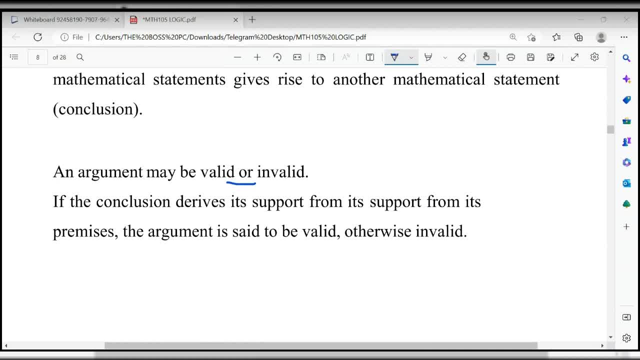 now um, for example, that deductive argument we can say. what i want us to know is that this um argument is valid and invalid. can we hear me- yes, sir, we can hear you now this argument and invite agreements we have here. we can only use it when we are talking about the deductive arguments. 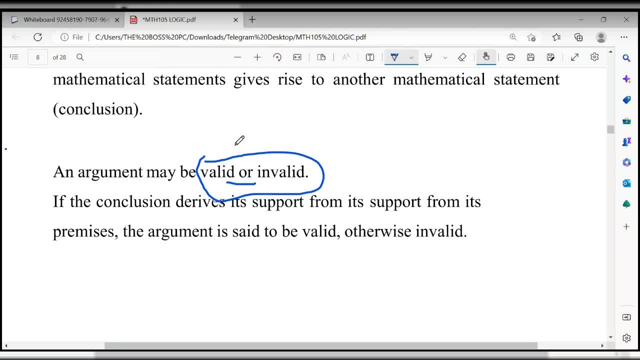 this is only deductive argument that can be valid or invalid. so a lot of the arguments that we have are valid or invalid. deductive argument establishes a conclusion to be true by stating two or more true prepositions and premises. that leads to conclusion being true. okay, now if you come and they said, if the conclusion derives a support from it. 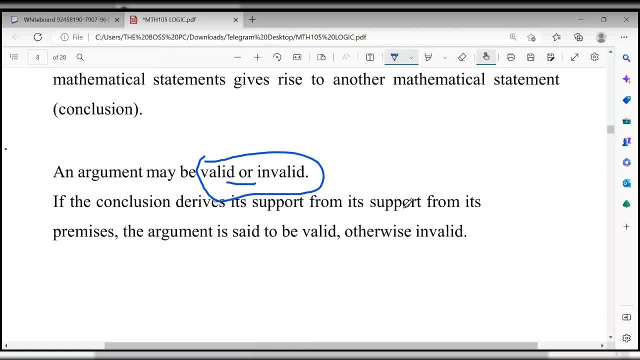 um, derives a support from. excuse me, please hold on a bit up. let's see this point, this point, maybe two, that's okay, i'm back. he said that if conclusion, the rest is support from. yes, if conclusion, the if conclusion derives is support from it, from its premises. so this is the repeated. i repeated it, right? so 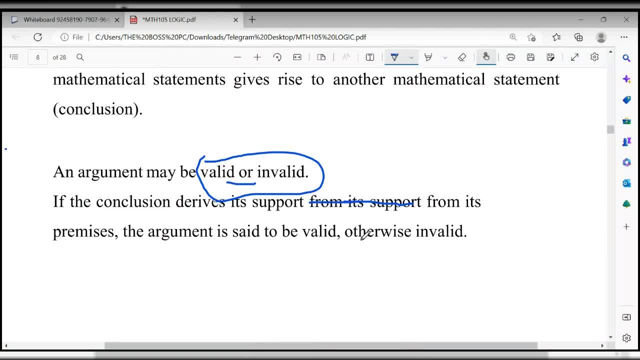 and the rest derives um his support. okay, the argument is said to be valid, otherwise invalid. so i will explain that deductive argument very well to us now. in deductive arguments, a conclusion- all right, um is being established by stating two or more you know true premises. okay, and these premises? 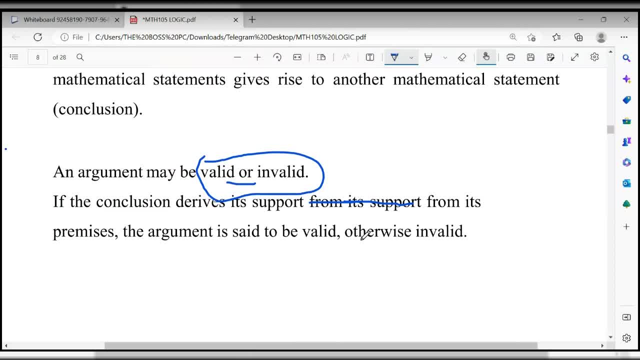 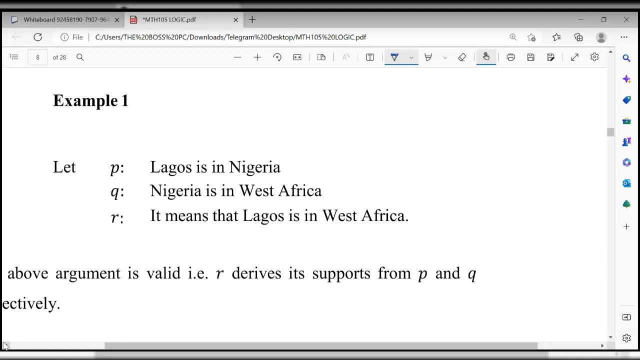 we always lead to a true conclusion. now, if that is not the case, definitely we have an invalid argument. okay, so, um, we can see an example that they gave us here. so in this case we have: lagos is in nigeria. that is, um, one of the premise: nigeria is in west africa. i miss, then, this one. 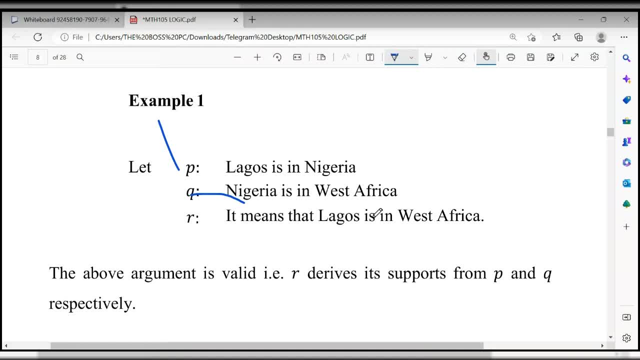 is the conclusion. it means, that's what. so the conclusion of the arrived from this is that lagos is in west africa. so in this case, if a and b are true, then c must be true. so in this case now, if lagos is enough, nigeria is true, and then nigeria is in west africa is also true. 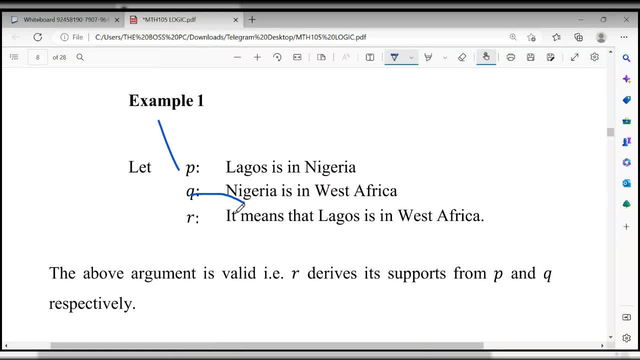 and definitely this one where we say we, where we would have conclusion there that um, because deduction means that we have actually um got seen it from this. okay, it's, this led us to this. it means that what lagos is service in west africa will be true. so we have example. 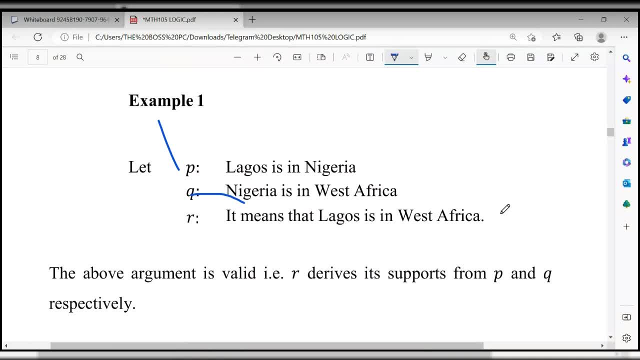 here others are going to give us. all dogs have four leg. um john, john's pet is a dog, therefore john's pet has four legs. so in this case, um you can see that it is worth valid. another example: all dogs are animals. rover is a dog, therefore rover is an animal. 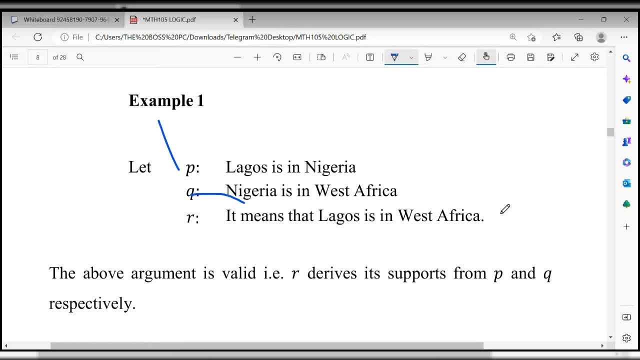 so in this case we can use the example of an invalid dog in the argument. so this is the example of an invalid dog in the argument. then we have an example of an invalid argument if i say here: john owns a dog, rover lives at john's house. therefore, 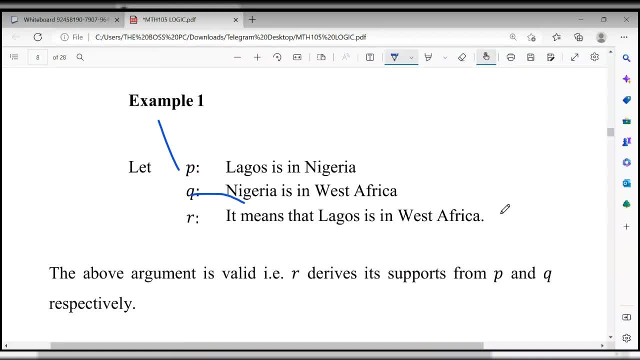 rover is a dog. Is this actually valid? Certainly not, Because, yes, even though John owns a dog and Rover- we don't know who Rover is- lives in his house. There are many other things that could be in John's house. all right, that will obviously not be a dog. Because he owns a dog doesn't mean 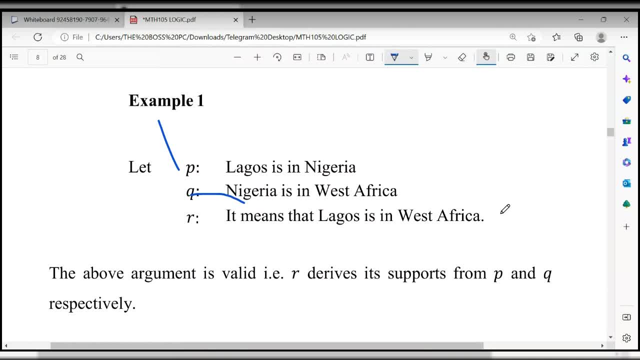 that everything in his house is a dog. So it might not be accurate for you to say that Rover itself is a dog. So that is that for that So inductive. when we say deductive argument, the conclusion is always: 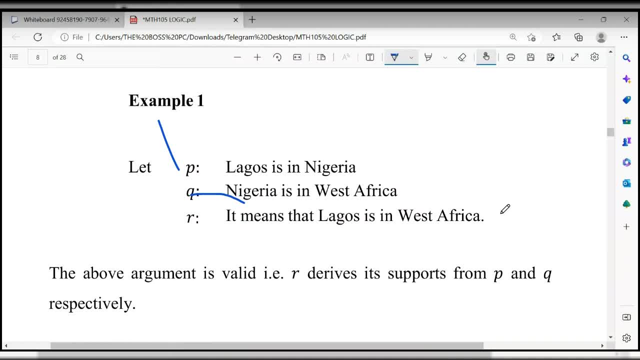 true, okay, Yeah, it's always true. If it is not true, it becomes invalid. It must be true, all right. But when we have inductive argument, conclusion is only probable. all right, Yeah, it is probable. It must not. it does not have to be true, okay. So let me give you an example of 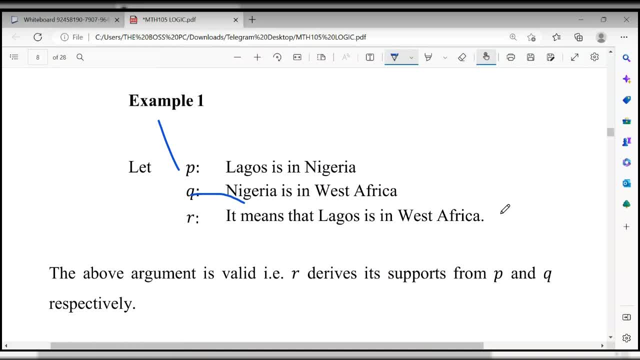 inductive argument We have here: most dogs have four. Rover is a dog, Therefore Rover has four. So you can see here the premises that led to this conclusion. that is the first one. most dogs have four. That is that they are, they are. they are skin, the, not skin the kind of 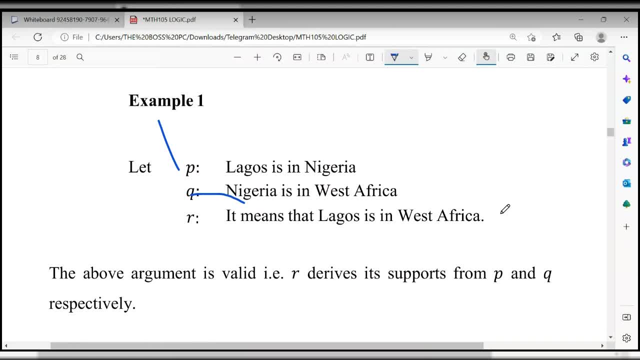 hair is on their skin, all right. The second one, Rover, is a dog And then, because of the fact that most, they don't say all dogs, they say most, not all. So if you look at it, it is said that you. 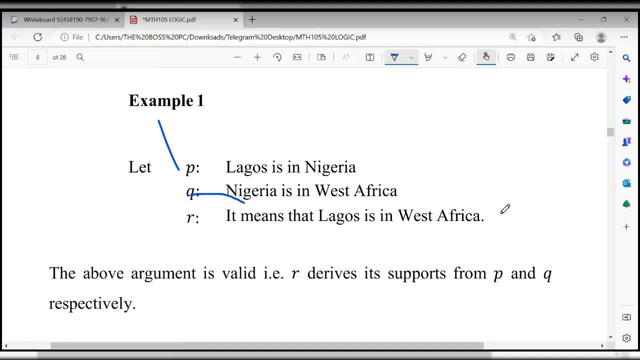 can see what happened last: quality type term grounds. if deductive argument is strong and the premises are true, then it is said to be cognizant. This is like a deductive argument being valid and sound, The exact distinction between deductive and inductive. 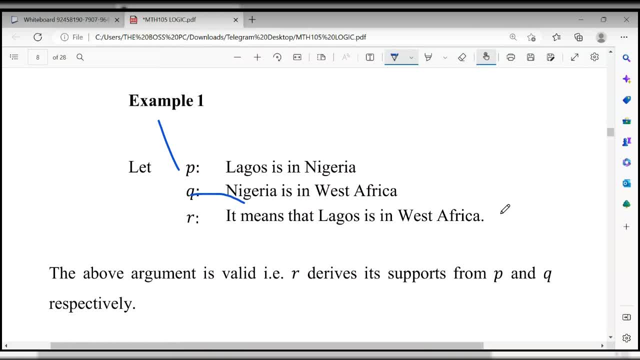 argument is not fully accepted by all philosophers, So only use a slightly different definition. Others believe that there's no clear distinction between the two and that instead all arguments have different qualities. That means their type of category. The end goddamn argument is the one with Tier and what kind of mosquitoes in it indicates that, unfortunately, it has no clear definition. you'd beWhoa the venom of pol管. 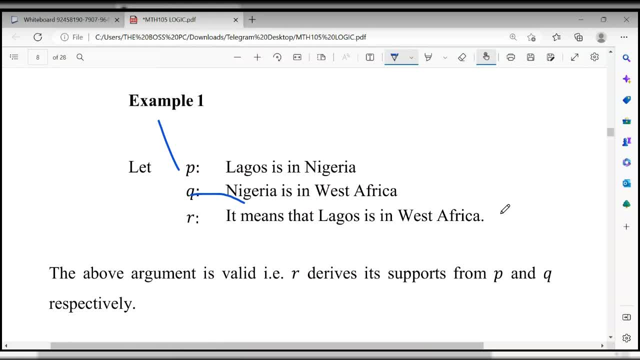 categorization difficult or meaningless. so there you have it. the main thing about inductive argument that separates it from deductive is that act of probability, and deduction is not does not give room for probability. it must be true, okay, otherwise it is worth invalid. so a valid deductive argument is one whose logical structure of form is such that if 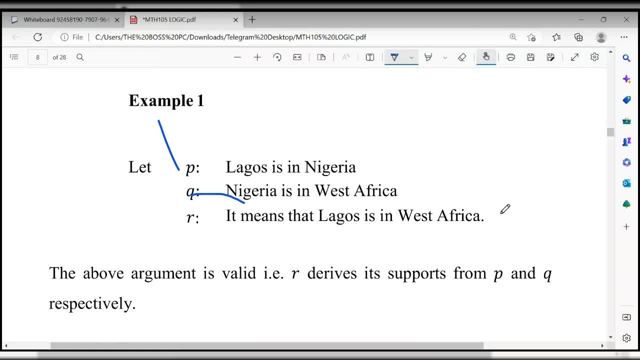 the premises are true, the conclusion must be true. okay, a sound argument is a valid argument with true premises. so once you have the premises, which is, in this case, P and Q, once they are true, conclusion must be true. that is what deductive arguments for you all right. 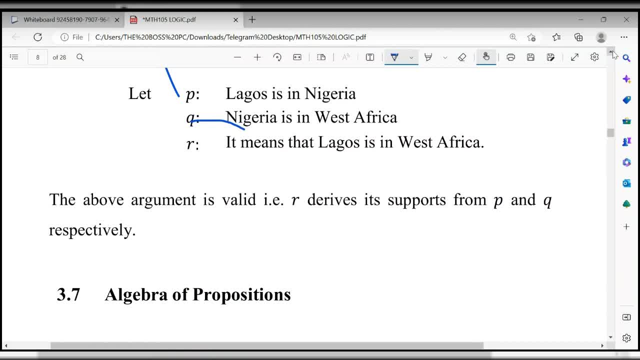 so do you have any question on that? so what does the R stands for? that's the conclusion. that is simple. that's the conclusion. okay, I'm going to give you guys two premises. I'm going to give you guys two premises in the comment section and I expect someone to give me, um, the best conclusion for that argument. are we ready? 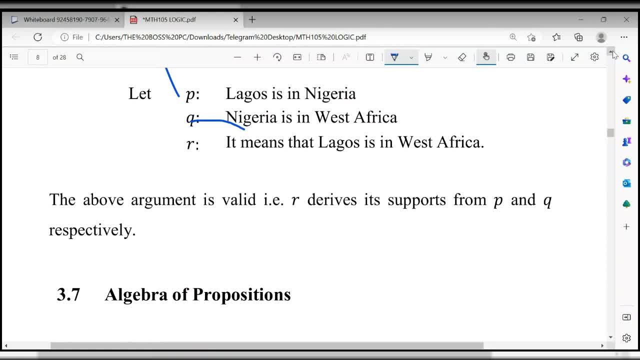 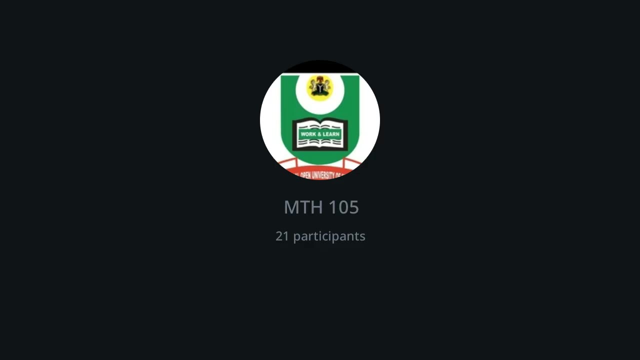 are we? yes, we are ready. okay, so I have one for us here. all dogs, five years, all right, that's the first um premise. let me call it P. okay, it's going to be in the comment section, so reply to it. and the second one is that, um, I'll call it Q now. um golden retrievers. 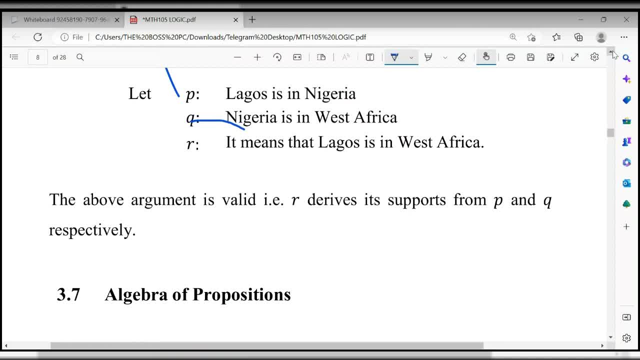 are dogs, are the second ones. so, ah, which is the conclusion? somebody should give me that. so what will be coming again, please, come again, please. comment session: is there? all dogs have ears. golden retrievers are dogs, therefore. oh, now, so give me the conclusion: foreign, foreign. 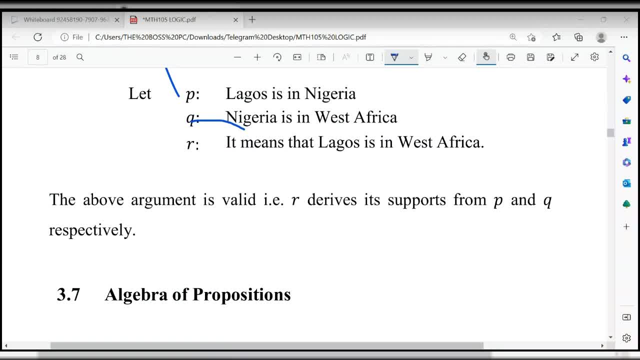 the question has been typed. the question has been typed. um, while we are on that, I also have another one. all racing cars must go over 80 meters per hour. the Dutch charger is a racing car, so I need a conclusion for that. um, um, I'm enjoying this. let's keep it coming. 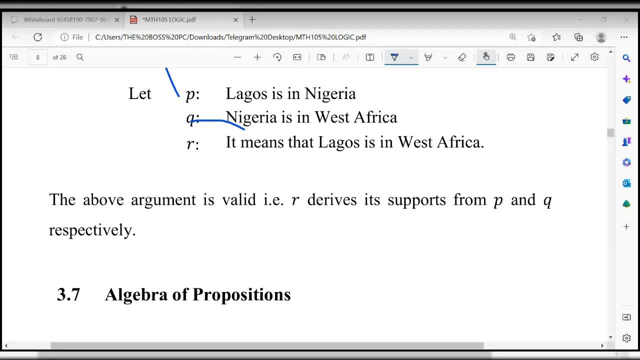 some of us are making me laugh already, so let me call this on a: all racing cars must go over 18 meters. I said I thought I called it reason. you would think you would think like your brain, because these things you think is simple, some people don't think they are logic. very simple thing. then you sit down, look at it. you know it's not simple. it can confuse you. 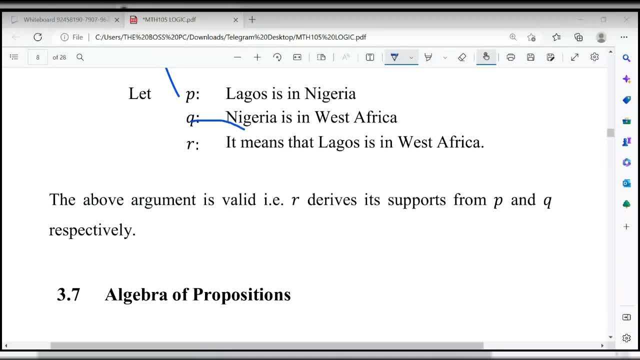 so um, another one is there. all racing cars must go up over 18 meters per hour. the Dutch charger is a racing car, therefore are they Ocean Catherine? so I'm seeing some of our comments. Mr said that all those are wooden. the question is: all dogs have ears? what 30 cent dog? 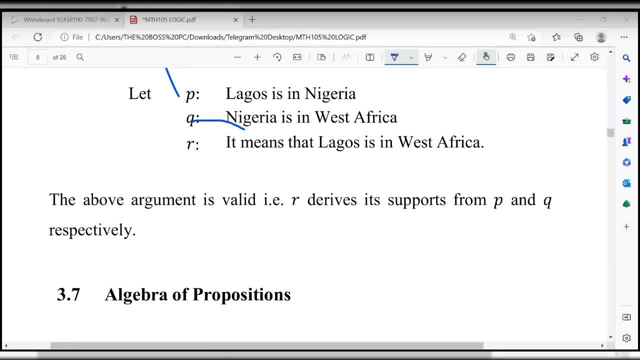 find that and therefore all those are golden retrieves. okay, um, miss, I do see you is your, is your master. um, all dogs have ears. golden retrievers are dog. therefore, um, golden retrievers have ears. um jason, hey, jason, you, how do they pronounce this? your name, mr jason? 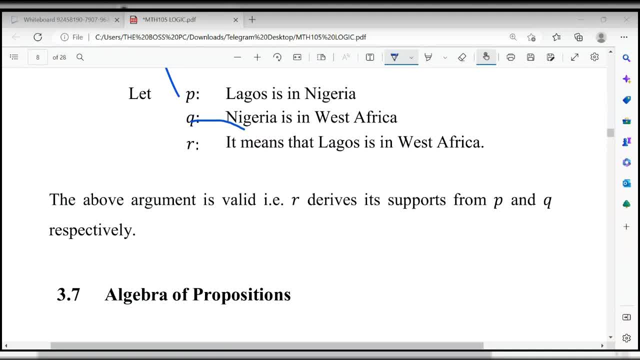 so, um, he's saying that it means that all dogs are golden retrievers. uh, mrs adib bruce, doing me salami said that therefore they have ears. um, michelle says: um, therefore, all does have golden retrievers, all does have golden retrievers have. 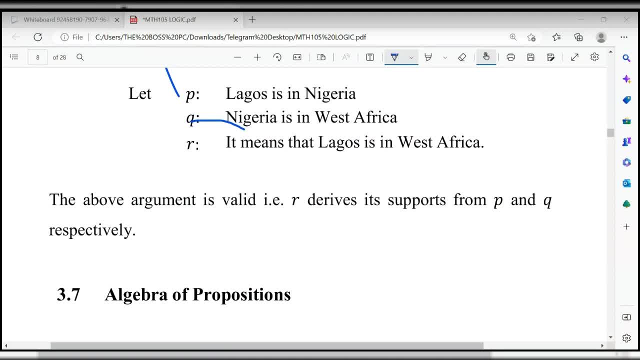 ears. hello, yes. well, the next one is also. there's another one there. the other question as well. yes, um, for like five minutes, let's see. so mr said that all racing cars must go by 18 meters per hour. the douche charger is a racing car. um, therefore all racing cars have huge charger. okay, noted. 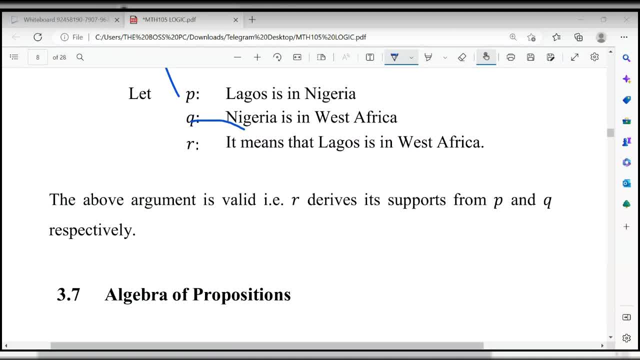 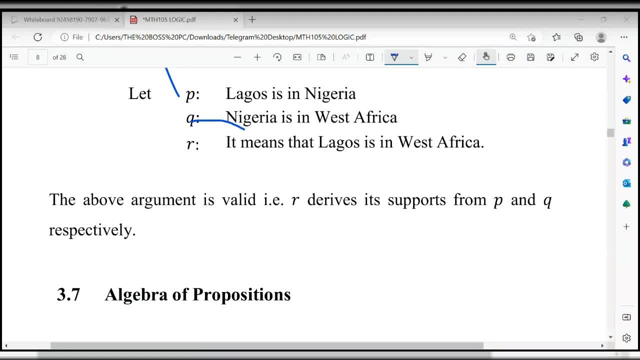 If you have questions, you can also drop in the comments section. my eyes is on it. Okay, Jason is saying that all racing cars must have a dual charger. A dual charger is a racing car. That means all racing cars must have a dual charger. 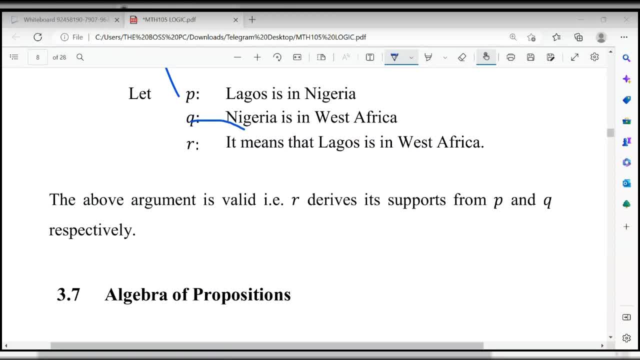 Okay, All racing cars must have dual charger. All racing cars must have dual charger. all of you are copying yourself. that's not fair examination. my practice examination, my practice. what brings around the course material? um, this could be typographic, typographical error, you know. 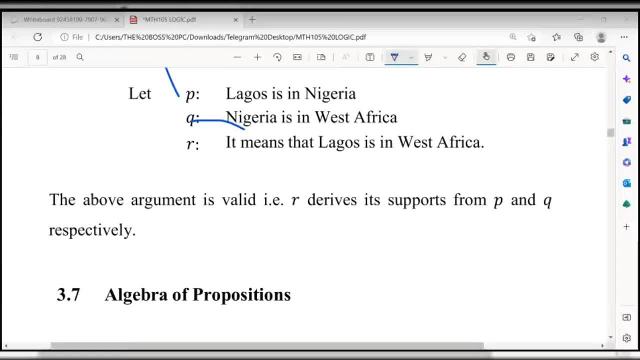 maybe the ones that i know. most of these symbols are not easy to locate on on the keyboard. some of them you need to use additional um additionally, this addition in depth knowledge of um you know. all right, so let me give us the answers. okay, let's keep um commenting. anyway, we have been doing well. 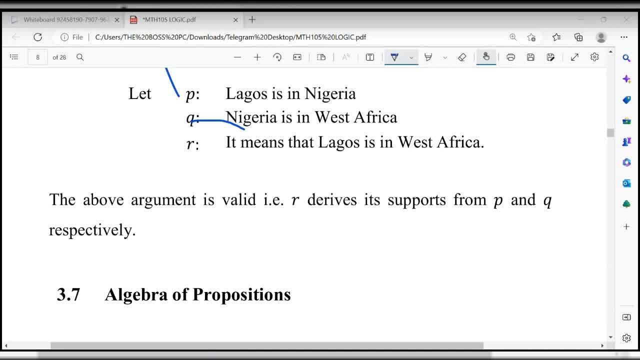 so, for the first one, all dogs have ears, go, the retrievers are dogs. okay, therefore, so all dogs have ears, golden retrievers are dogs, therefore they have. yeah, that means golden retrievers have ears, since they are dogs, and we definitely have, yes, since all dogs has it. 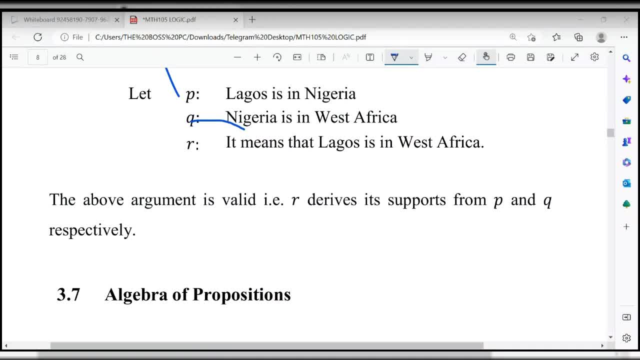 that should be the conclusion. if you got it, start celebrating yourself in the comment section. now, all, all dogs, all racing cars must go over 80 meters per hour. now the dutch charger is a racing car, since all racing car must go above 50 meters per hour. 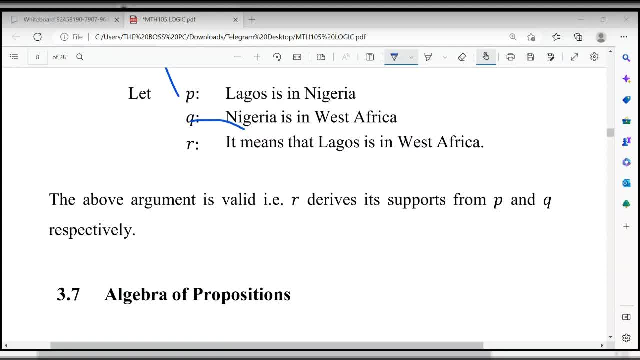 can you hear me now? hello, can you hear me now? yes, um, hello. so since, yeah, i'm hearing you, yeah, thank you. so it's all resting: 80 and 80 meters per hour. it means that the dodge charger, which is a racing car, must go over 80 um meters per hour. if it doesn't go over 80 meters per hour, then it is actually not. 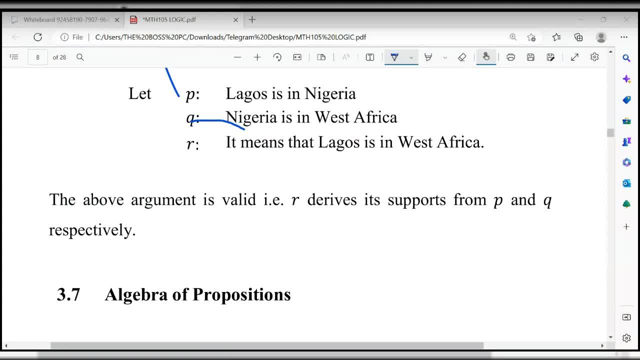 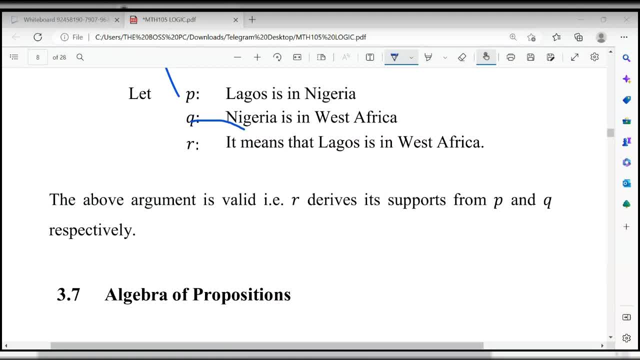 fast. hope you had fun. hope you learned something. eventually i've learned something. give me a love emoji, email emoji. if you still have issues, you know. give me an excuse me a comment session. i mean, where to excuse? you are already getting so much love already so you can see the. 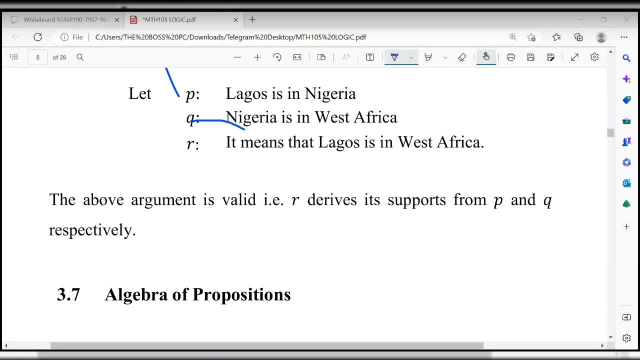 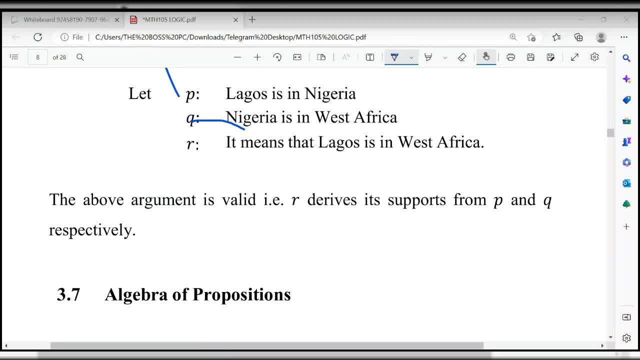 wonderful doing this with us. probably maybe if we don't meet over the weekend then we'll meet next week- need to be very, very busy because most of these things if you don't, if you keep going at it, you know consistently you might get forget completely. so we need 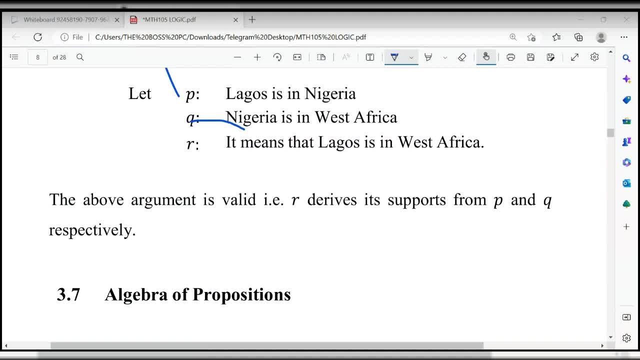 to keep ourselves busy until the next time we come around. so everybody that actually participated in the class, God bless you. all those of us that joined us much later, later, later. yeah, God bless us. so I'm going to, you know, send, I don't know. let me see how we were going to use think I prefer working on this platform. 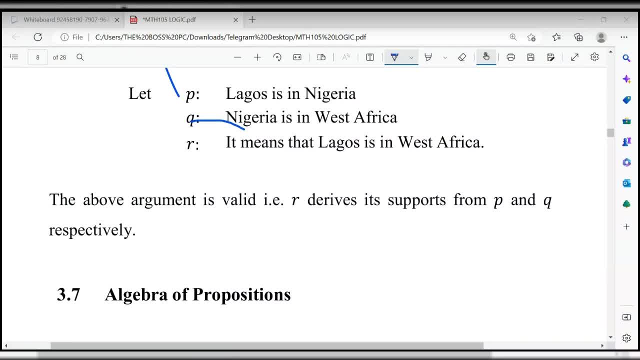 for. so I'm going to you know send I don't know. let me see how we were going to use. think I prefer working on this platform for serious businesses than I'm what's up because of I'm this platform. you know what's up if you lose any message. now that's me, all my messages I can't find. 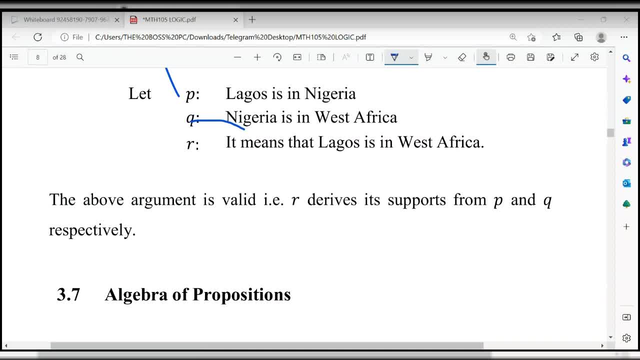 them again. anything happens, your what's up look for you start looking for your chats. that's why I feel like, okay, this one, you can always even assess messages that we are not in the group when it's when you and with our way in the group when you're not even a dead. so I think I will, I will. 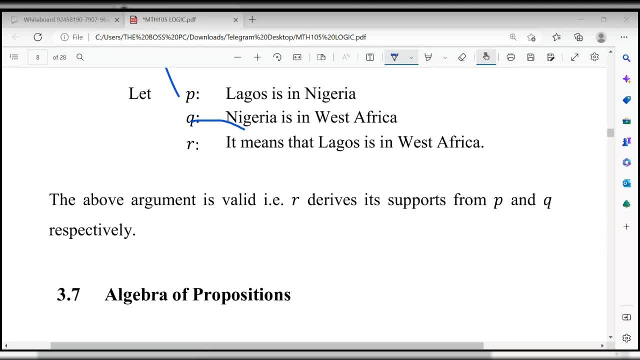 go to send the Mathematics on link. that is much, but much is for managers. you will be arguing outside the link. I'll send to me. I was at D so I'll send to you. and then we're supposed to share mr position, because to share on my 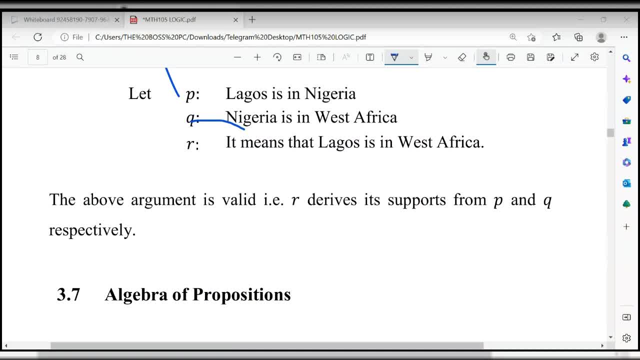 social I can join and then so tomorrow, so more money before you need to come and come on to my page. I have a link in the description so you could see what I just did. so I will send a link in the description for my business. now I'll send to miss Abbas a d, so I'll send to you and then you were supposed to share. miss Abbas a d, so I'm supposed to share on my social, can join and then so tomorrow, tomorrow morning before we need to come, and you can. yeah, that's really useful. 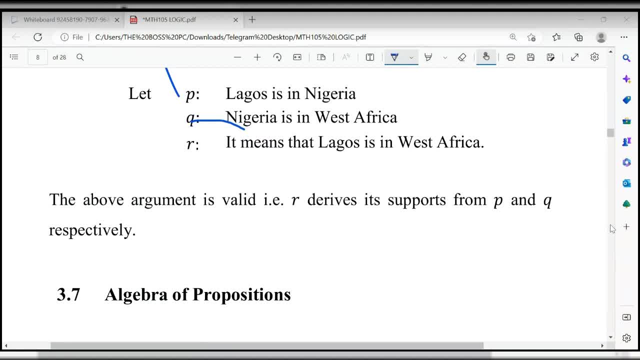 can write in your notes and share with them and type. you can use voice notes. anyhow, you know that you can be able to share um what um we learnt so that those that were not here with us live we know what they have missed and can also recap and um see why next time we call for meeting, they should. 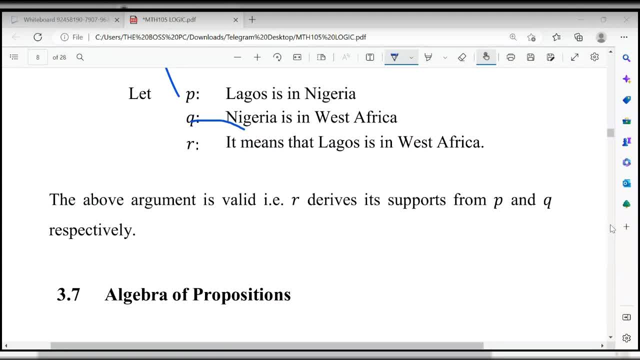 be able to join us live and um, while you are done, i'm going to later in the day- um, it will be. let me see how that person that was. we thought from the very beginning, okay today to be miss m at the bc, adib salami. so both of you will work tomorrow as a constant discourse to make sure that okay. 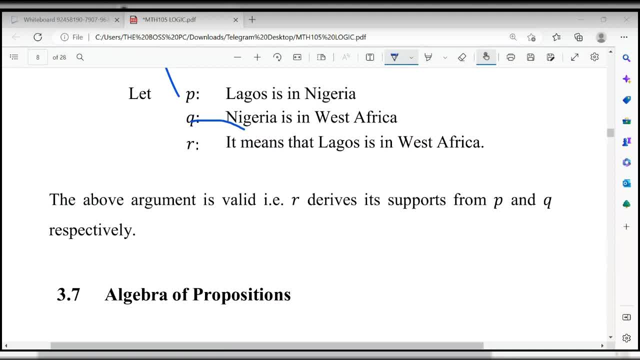 just to like talk about what you people learned um today and then if there's any assignments um that was giving, you guys will share and also encourage your colleagues to subscribe better. subscribe because first this morning it's not easy to see us. i've been talking since morning. how many hours. that my voice is already lost. i still have a lot of work to do, so i'm going to go ahead and share with you guys. i'm going to go ahead and share with you guys. i'm going to go ahead and share with you guys. my voice is already lost. i still have a lot of work to do, so i'm going to go ahead and share with you guys. 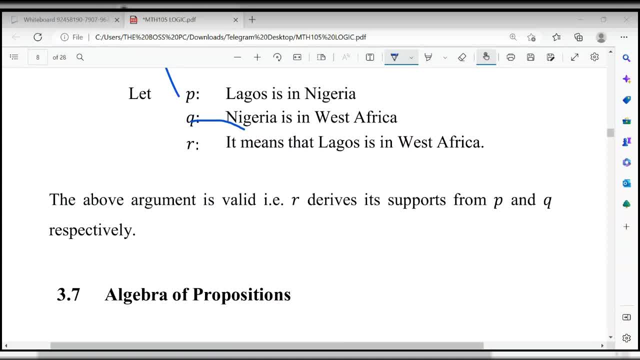 a class by nine o'clock, please subscribe. okay, and um, that would be it. so on sunday, another two people we have to come out as well. is we still be on this same course? okay, we will have our classes. like you know, other things will be going on, other activities will be going on, but still on the same. 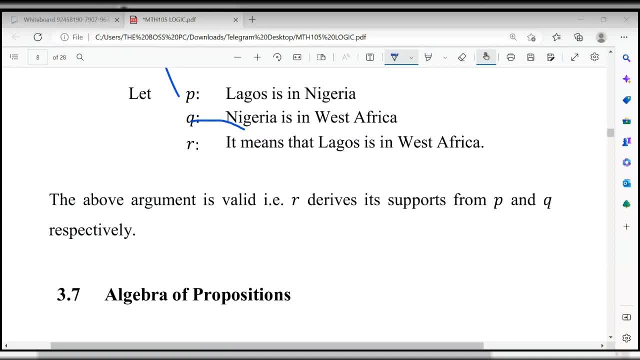 topic so that when we come again we can continue to be sure that everybody has. i'm very sure that some people now where their lives like this. some people are not even getting what they're saying. some people network or disturbing them. some people we are, you know. 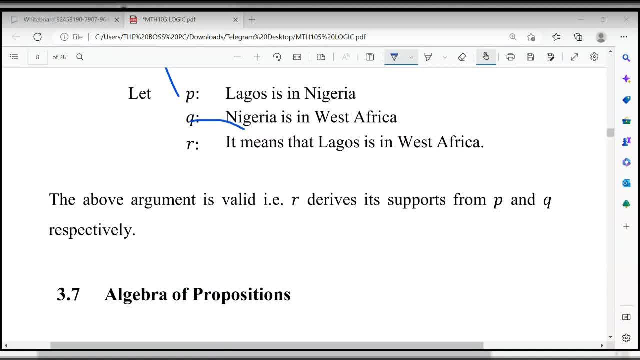 um, so um from our feed. but by the time you drop that your comment, people will definitely react. some people will still tell you that: oh, no, no, no, no, no, this was not what was what was said. look at it before you know it. you know, i myself too, i'll be seeing reactions and knowing where to also come. 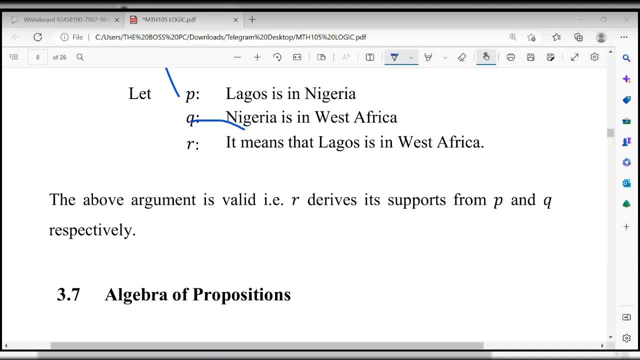 in. if i need to- um, you know, put more clarity into what we are doing, so that will be. um, it's for that right. so on sunday we'll be having mr israel. so mr israel, take notes. having mr israel, and, um, we have mr israel, and mr boss said this, we still have to work with him, so 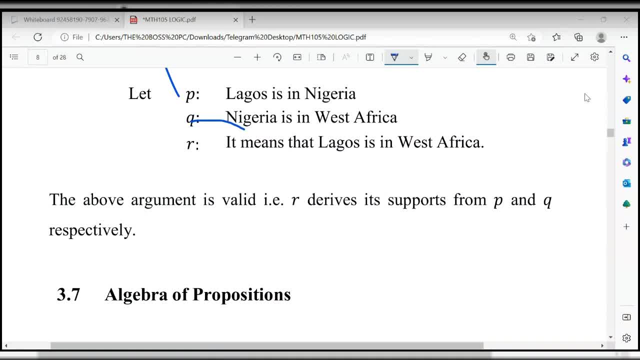 on sunday it will be mr israel, and mr boss said this. so, um, obviously, from what you have from your international tomorrow, you obviously have learned one or two things. you can still top up on sunday. so if you have any- uh, any questions about the west, one or anything else, we're glad to hear from you. 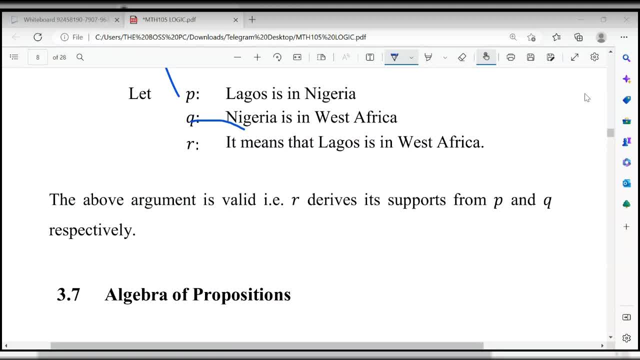 so, um, we'll be uh, around sunday. we'll also be doing, uh, a podcast about, um, about the west, um, so we'll be doing, uh, some moreonte, our let's. also, we will be doing JST, and the most important word we will do is: we're gonna have 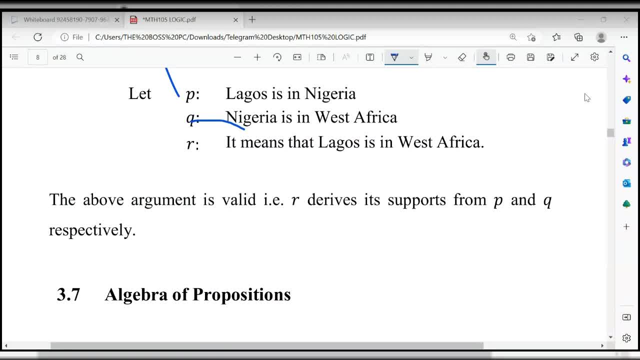 a workshop there, uh, and we'll be doing something about the us and our um their church church service, um, we can just do that. so that'll be for um mathematics. so let's also we have a class. um, we'll still have a class later. that is the GST. we also do that. defense of people. we. 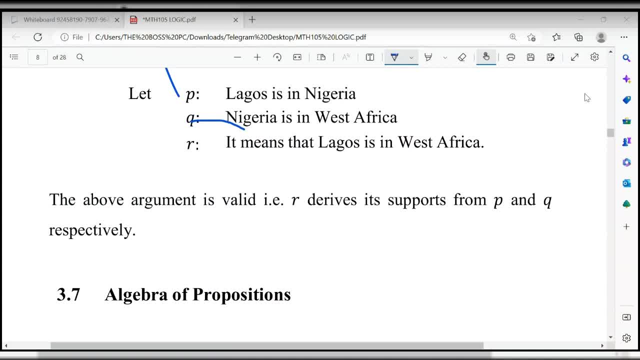 the topic and course you are giving to like review. you will. review is people will come in there. they will, you know, and some people also study on their own and go through replays as well. they also come in and drop their own imputes and stuff like that. so we can always also learn from each other, even 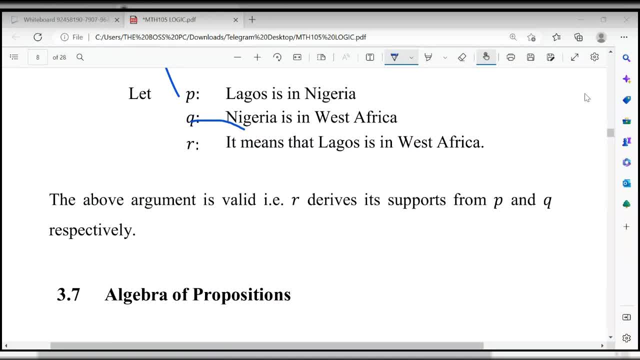 aside from just coming here live, you also get to pick another thing from your colleagues as well, based on what they have learned from being in the class. i believe we actually um, buy that idea, do we? yes, we do, yes, we do, and we are ready to work. and you know, do i play our part? well, please play your. 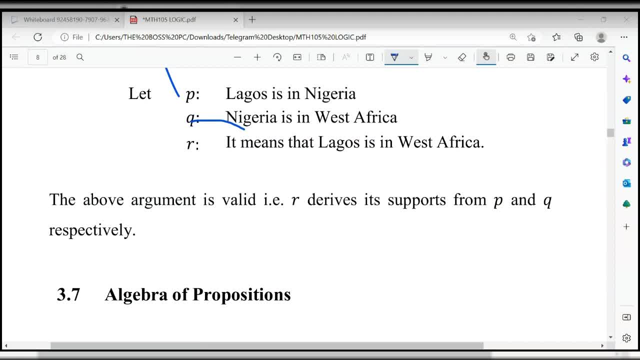 part very, very important, because we're not doing magic here. the boss is not giving you and i'm not. i'm not lying to you, i'm not gonna tell you. there's one, there's no secret anywhere that to read your book right, read your book now. exams are difficult when you don't prepare okay. the question is how much? 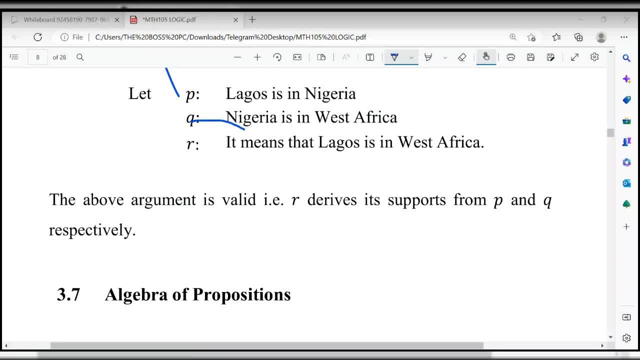 of preparation are they expecting from you? do you have what it takes to prepare enough for them to for you to pass their exams? so there is no any magic, any way at all. if you do not reach, you do not read. all right, if you like, join all the groups in now. okay, if you are not reading your book, if 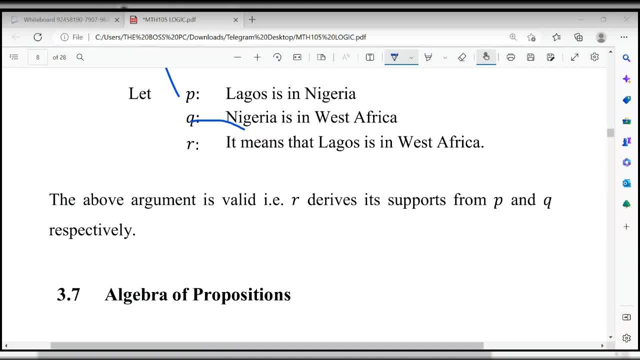 i'm not putting something into your brain, or that day you see, before your sister you come out, you ask your story. you're ashamed to say because you have done. not, it's not by paying anybody, it's not by doing it, it's about, you know, being ready. 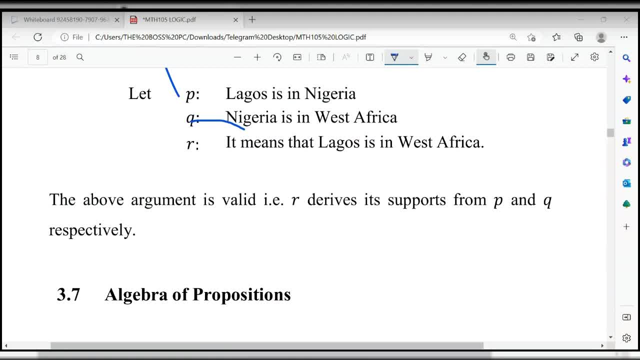 so let everything you are doing be a channel to help you understand what you are doing. okay, yes, so that is basically all i can say to us. um, at least so far, so good. i really appreciate um how we've started some of us after they very, very well and, um you know, long may. 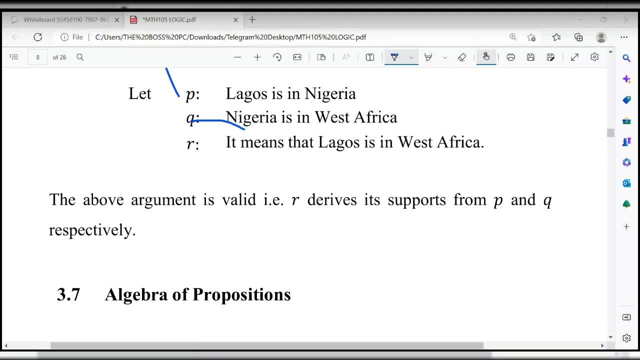 this good thing continue. so i think i can allow us to go so that we can take a breather and then come back at the top of the hour for our gst 107.. all right, so someone can pray for us, please, um, miss chantelle. chantelle, eunice, you can pray for us. are you a ghanian? 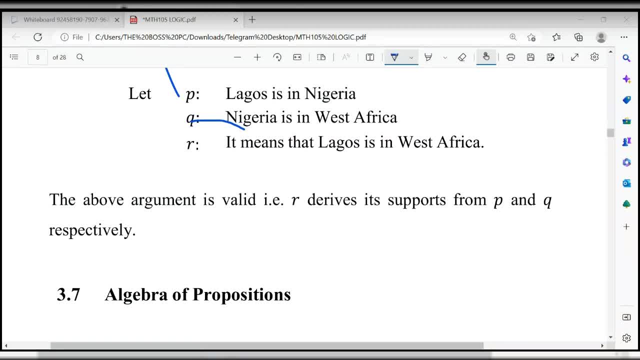 miss chantelle, you can pray for us, miss chantelle, are you there? all right? miss m isyoma, pray for us, please, please, don't forget your, your, gcb, um, gcb, your, your, your name, those that i i called out to do your work, and i believe all of us have gotten. 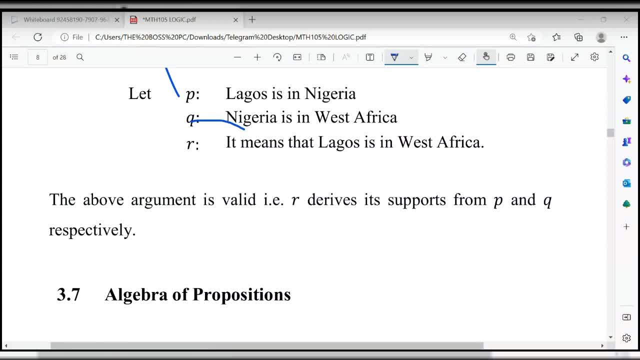 our numbers so that we can, i can be, i can know, um, when you, when you hear your number, you know it's you. that has been addressed, mrs. are you there, miss? okay, the girls are not going to play. the guys can pray for us then. mr jacob, mr israel, any of you can pray for us in the games. i want to. 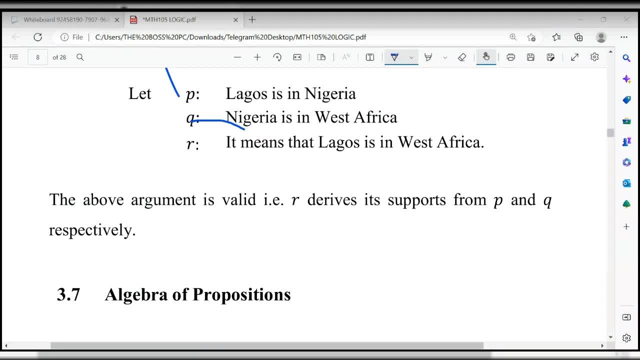 pray in the mighty name of jesus. okay, amen. father, king of glory, thank you for bringing us to the end of this class today. thank you for the knowledge we don't understand. we have a candidate in the beginning of this class, oh lord, all right to conclude. this guy to grow this guy, oh lord. 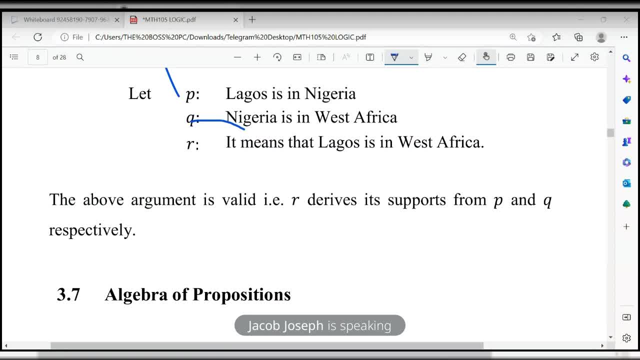 that's whatever we learned this night. whatever we have seen against you, whatever you have wrong against you, please have me and forgive us all, but we know that we are not right, so we are not perfect, but we're only working on that progression, oh lord. but as we are the students, whatever i think we may find as a difficulties, 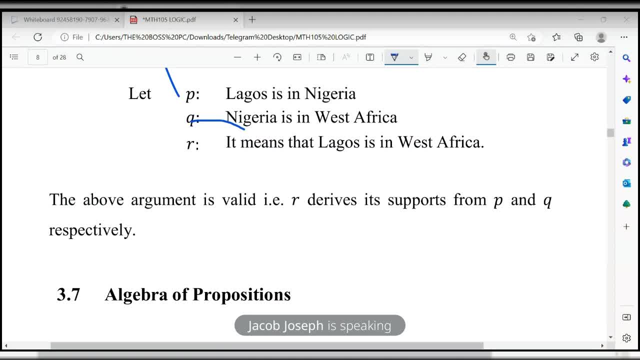 in our studies. oh, lord, open our eyes and give us the spirit and say more like be able to overcome every obstacle that may come our way. in the mighty name of jesus. all right, thank you, oh lord, for you know that we are god, that we still do matter lost in our life. oh lord, please tell me your name.